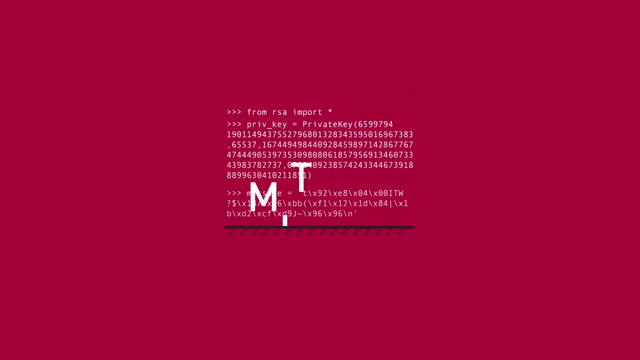 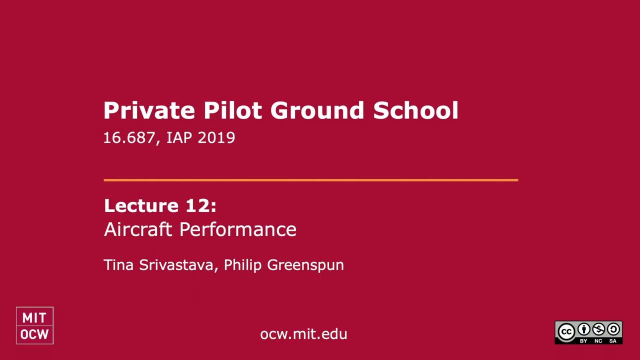 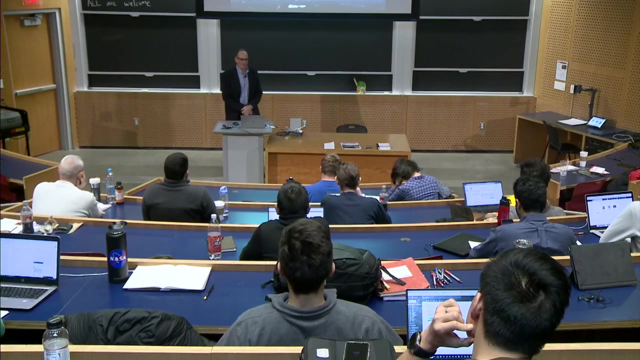 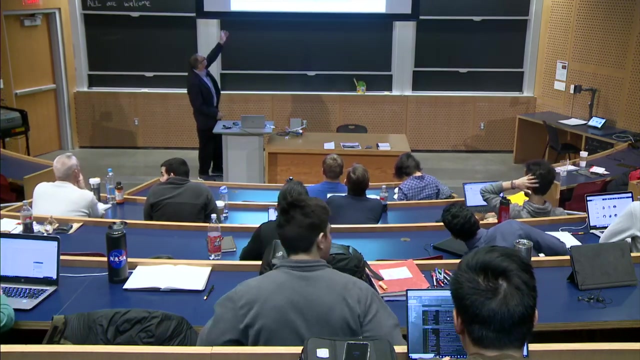 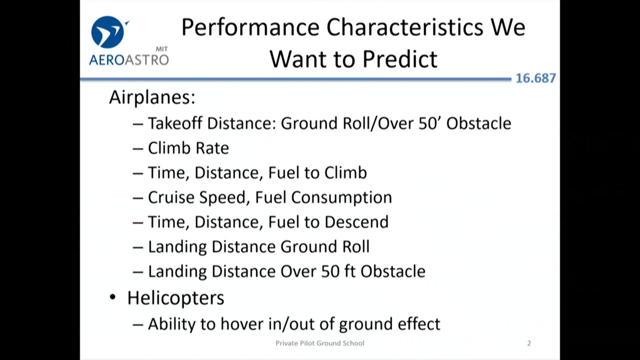 All right, we're going to talk about aircraft performance, which is figuring out all of this stuff. if you're an airplane, basically how much runway you're going to use on both ends, how long it's going to take you to get there, which, 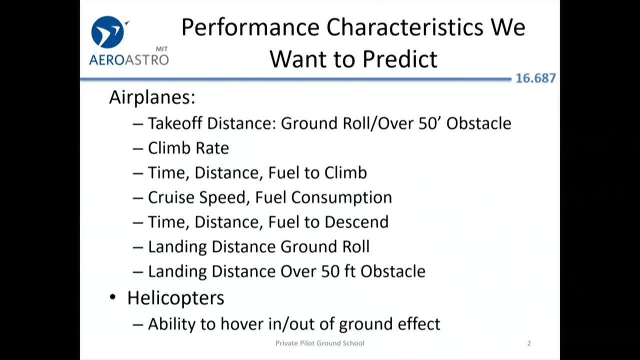 is another way of saying how much fuel you're going to use. If it's a helicopter, it's a little bit different. Mostly you're worried about hover performance. So if you're going to a friend's house, are you going to be able to park the helicopter in midair? 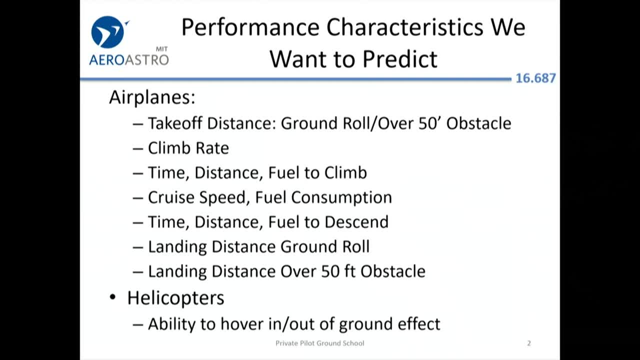 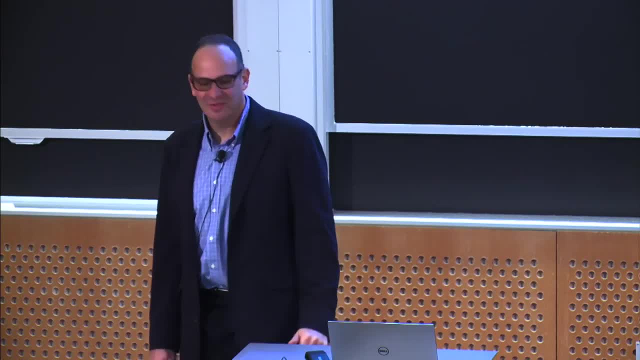 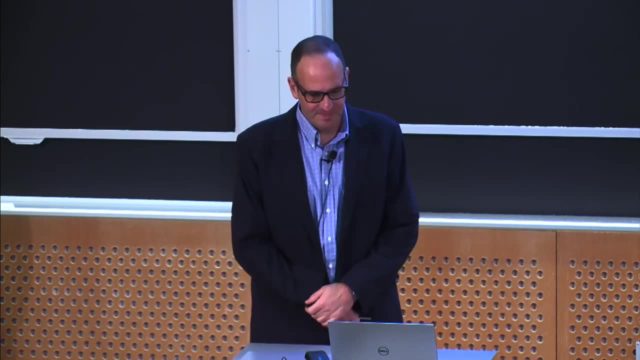 That's called an out-of-ground effect hover and very slowly descend into the backyard, dodging the trees and power lines and anything else. So these are all things that can be found in the aircraft manuals, and the FAA will test you on them a little bit. 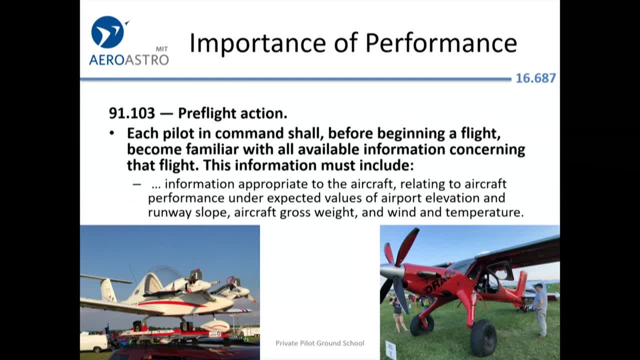 This is important, partly because you want to be able to complete your flight safely and also because of FAR 91-103, which is that before you do a flight, you've got to become a. It's pretty all-embracing, all available information. 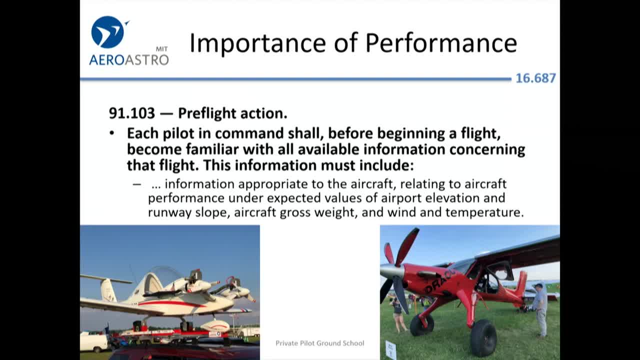 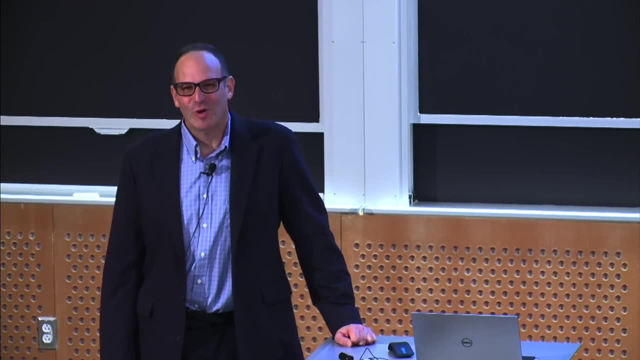 concerning weather and aircraft performance: how the aircraft's going to perform given the altitude of where you're going and the temperature that's prevailing there at the time. Wind also, If you find out that there's a 40-knot wind scheduled for where you're going and it's a direct crosswind. 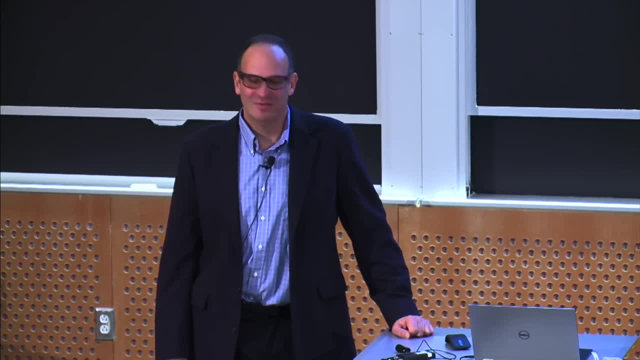 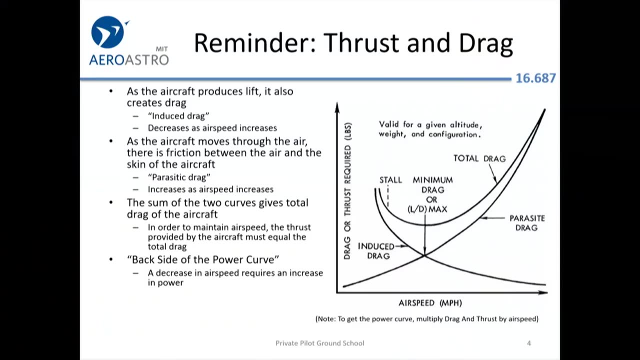 to the only runway, then that might cause you to choose a different airport. OK, Here's a reminder of Thrust and drag. Whenever you're generating lift, you're also generating some drag, And that's lift in the unwanted direction of backwards usually. 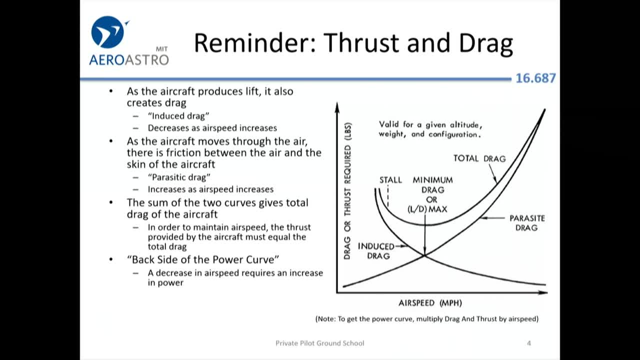 So the aircraft is also producing parasitic drag by trying to punch its way through this viscous fluid of air. Where these summed-up drag curves intersect is pretty much the bottom of the total drag curve, the minimum drag, or L over D max. 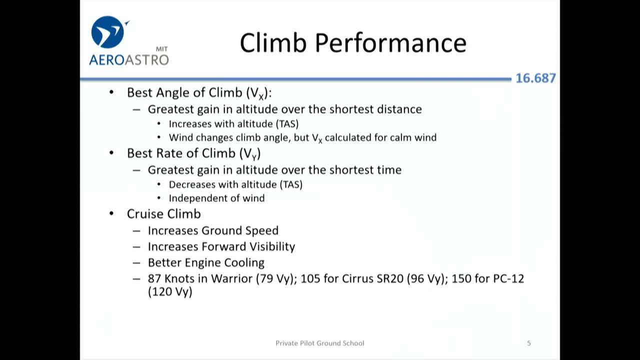 The climb performance, the best speeds to go are all kind of tied into this drag curve And the best angle of climb is what you use. That's a slower airspeed and the best rate of climb If you're in a small airport trying to clear. 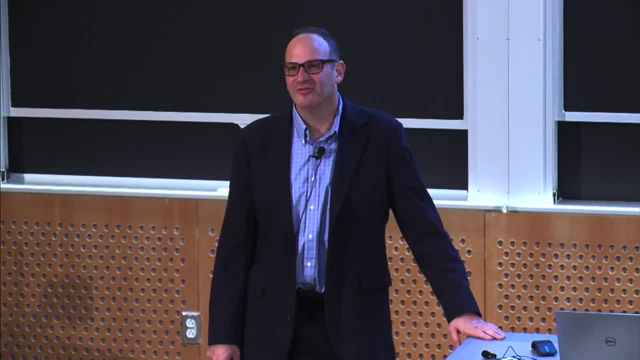 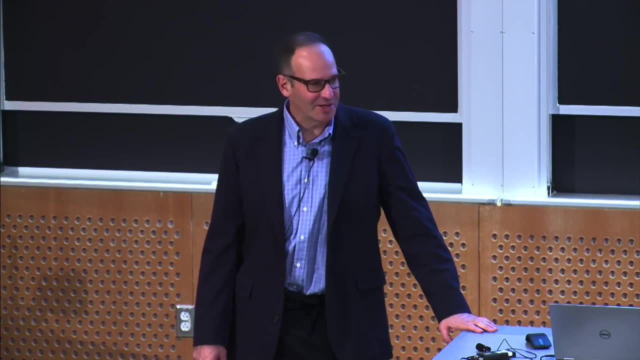 the trees at the end of the runway. you're going to fly VX, the best angle of climb. This is one of those few V speeds that you're actually expected to know the abbreviation for, And if you're going to just take off out of a big airport, 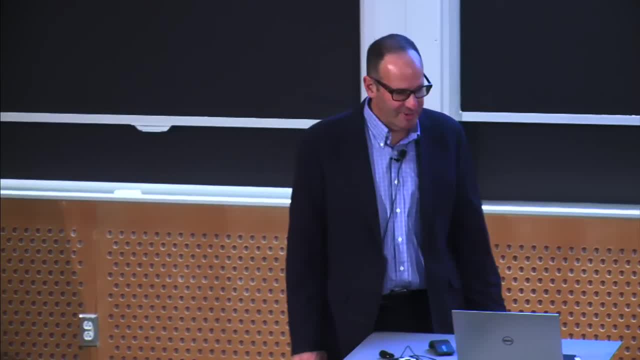 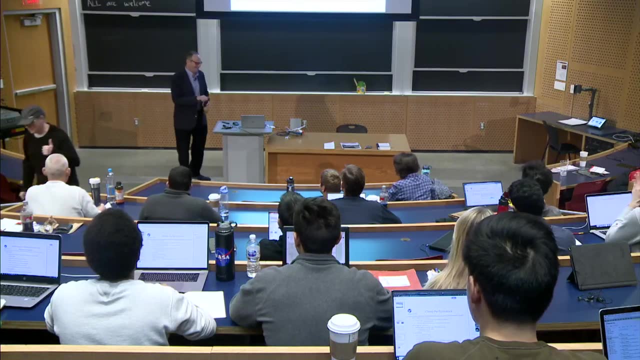 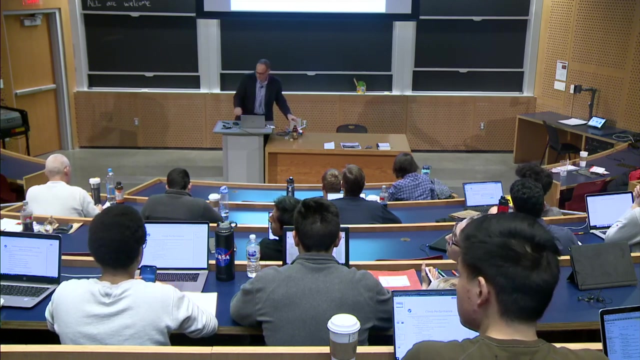 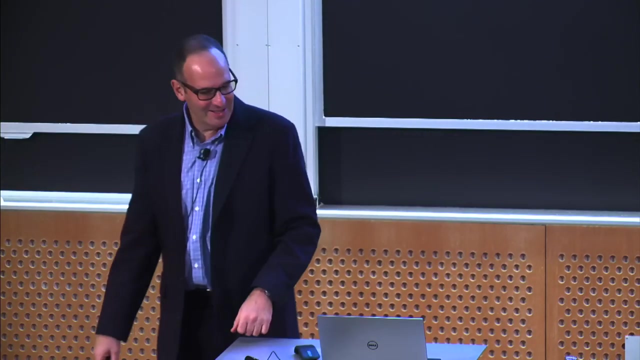 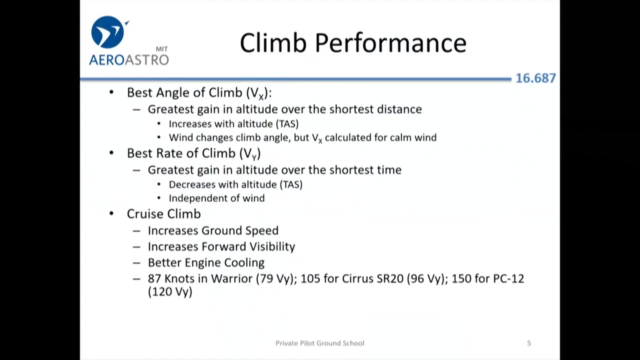 like Hanscom Field and just want to get up to your cruising altitude reasonably quickly, then you hey, thanks, Richard. Richard's, a Mooney pilot Made it to California many times. So if you actually look at the VX, one thing to notice. 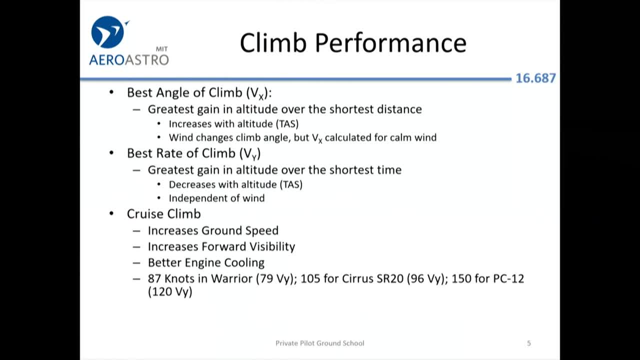 is that it will depend a bit on the wind. Let's say there's 100 knot wind blowing down the runway. You don't need to fly very fast in order to clear the trees at the end of the runway, because you're basically already flying. 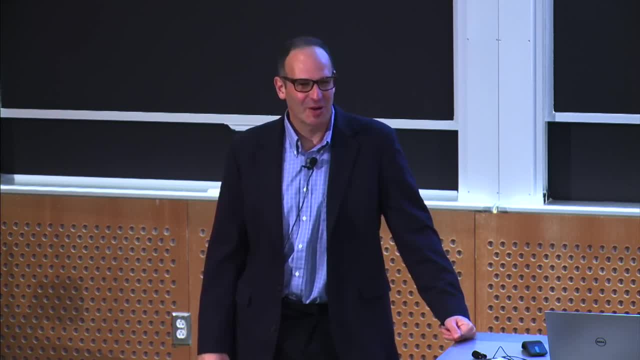 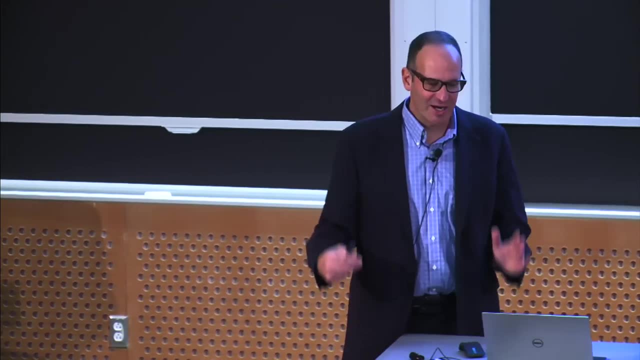 and you can go straight up like a helicopter In terms of your path over the ground, Whereas VUI just to gain altitude, that doesn't depend at all on the prevailing wind. So if you're trying to clear something on the ground, the wind matters. A tailwind would be very destructive- It'll be pushing you towards the obstacle- And a headwind will be very helpful. Cruise climb. most of the time you don't actually push the airplane to these speeds. They're pretty far nose up which. is a little bit alarming to passengers And it's harder to see over the nose and the engine isn't getting as much cooling air at these lower speeds. So typically we'll fly about 10 knots faster in a GA airplane. So for the Cirrus, for example, 96 is the book VUI. at sea level. 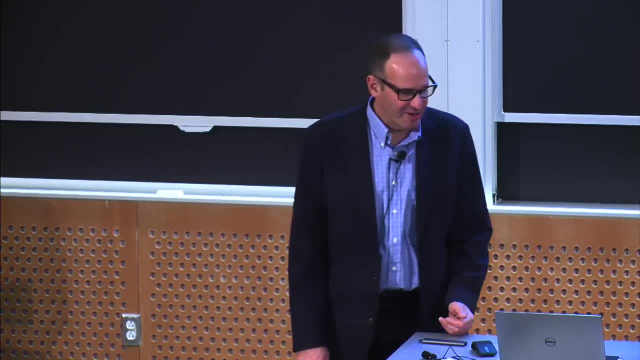 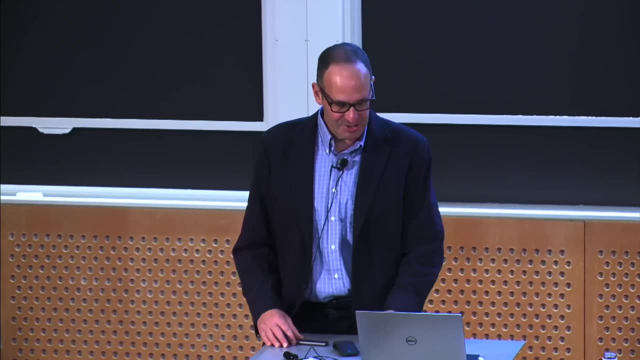 And flying something like 105 knots is more conventional. The PC-12 climbs, you know it might be able to do 3,000 feet a minute at 120 knots, But if you're not in a desperate hurry to get up above the bumpy clouds or something, 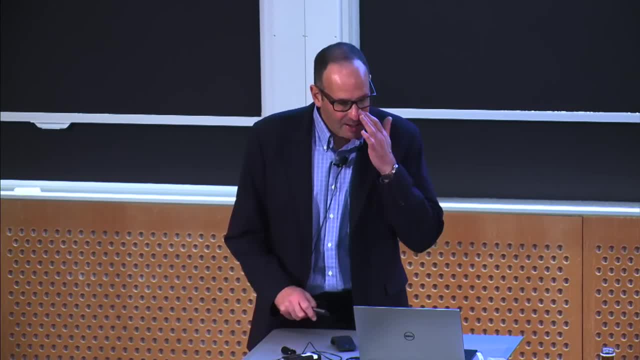 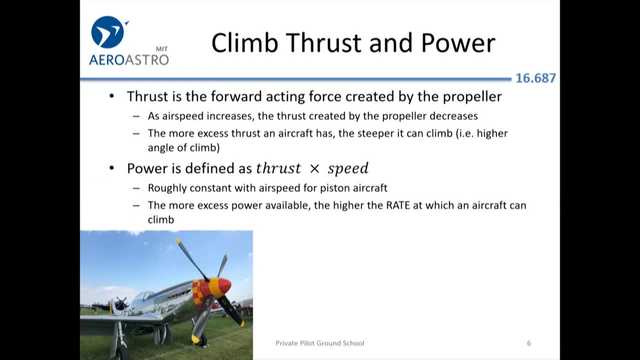 then 150 knots is more conventional, OK, so let's remember that you've got thrust and power. So the thrust is a force that lets you climb up over the trees, The power is thrust times the speed, And it's thrust operating over a period of time. 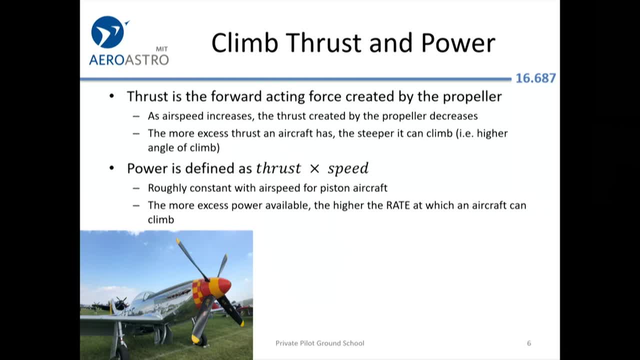 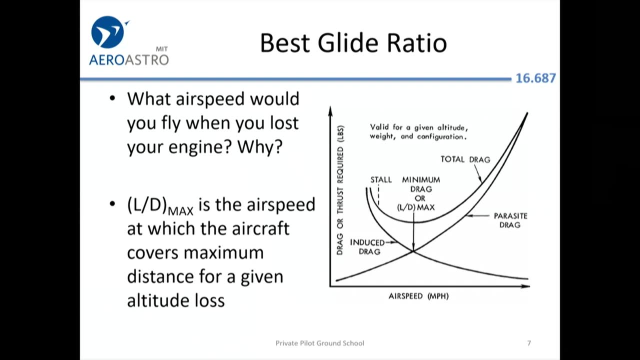 So the more excess power you have, the higher the rate at which you can climb. Anyway, we'll see some more of that here. You've got best glide ratio If you want to get to the decent place to land and you've lost your engine. what's a good speed to fly? 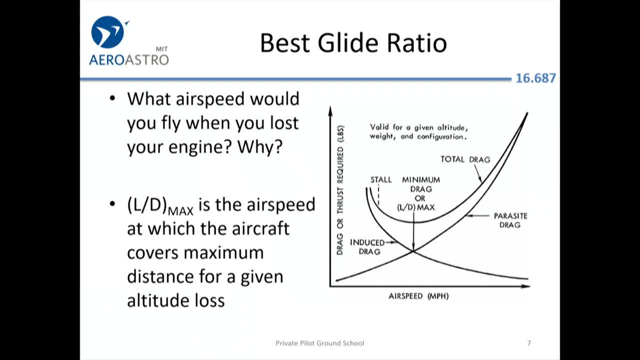 Well, L over D max is an excellent speed to fly, because that's where the speed is OK, The lift over drag is at its highest point And you'll make the best time over the ground. Again, that has to be adjusted a little bit for wind. 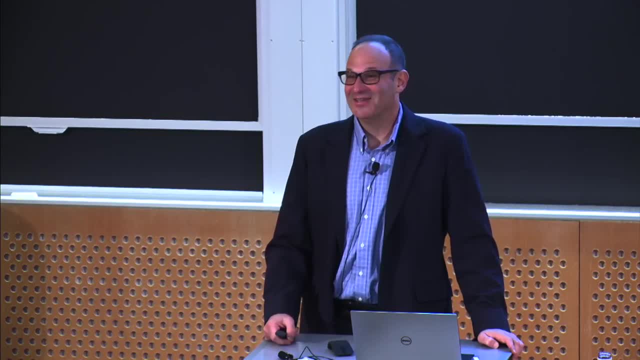 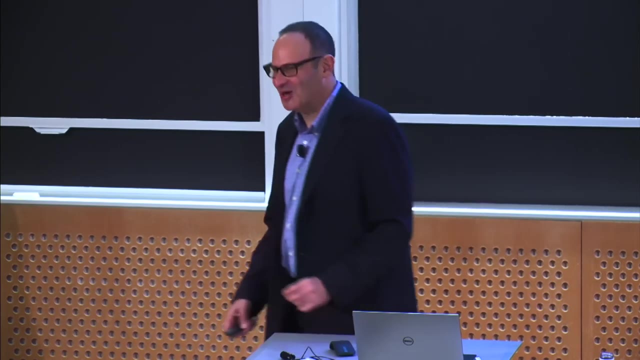 If you're going into 100-knot wind and the Cirrus' best glide speed is 96 knots, that's not going to work out very well. You're not going to go anywhere over the ground. That's a photo that I took at the Newport Jazz. 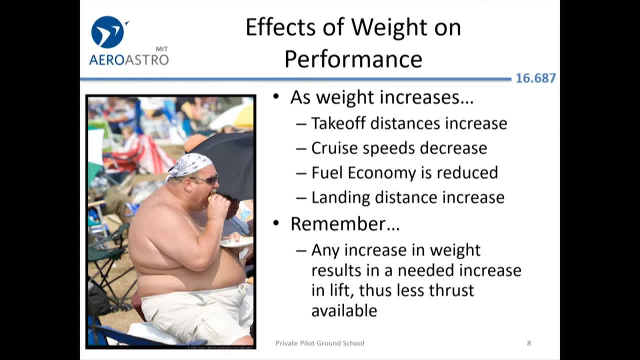 Festival. I don't want to say self-portrait. Anyway, weight has a huge factor on all these speeds because actually a lot of them are related to angle of attack And it certainly affects your performance. So everything about higher weight is pretty bad. 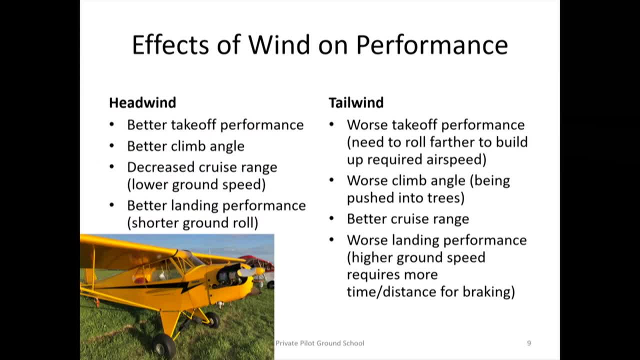 Wind. you might think that a tailwind is always good, But really the tailwind is only good for extending your cruise range. Everything else pretty much the headwind is better for. So think about the headwind again. Think of these extreme cases. 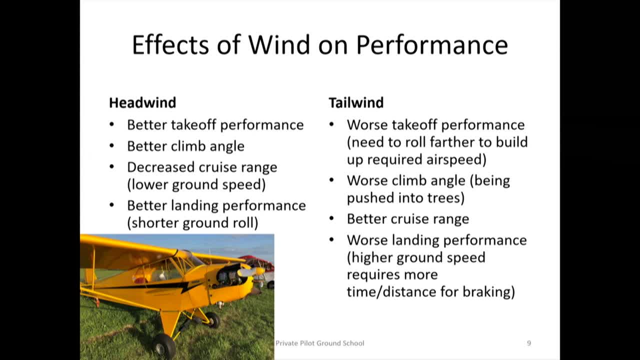 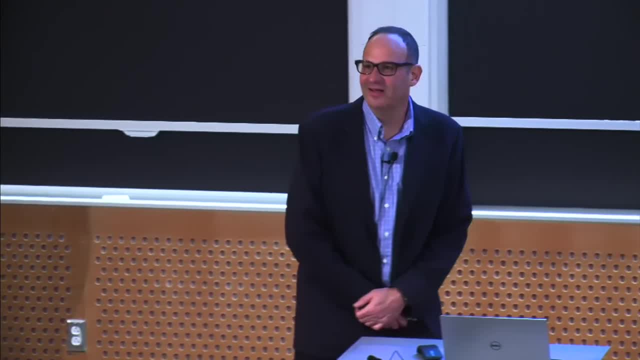 If you've got 100-knot wind right in your face, then you can fly without moving. That's basically a wind tunnel, OK, center of gravity. This is also a little bit counterintuitive. If you load the airplane up, you're going to have a lot of wind. 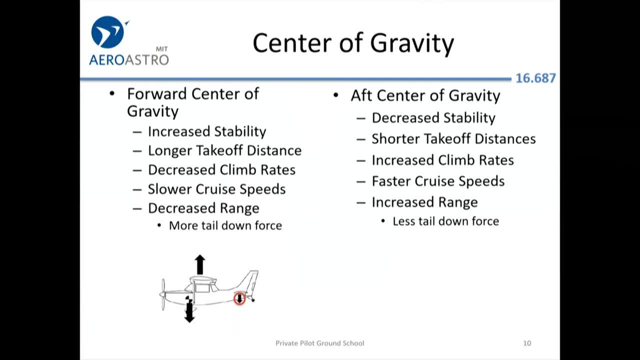 If you load the airplane up so that all the weight's at the back and it's super nose up and you're having to push the stick forward to keep the plane level. that actually is where you get your maximum performance. Everything is better about having an aft center of gravity. 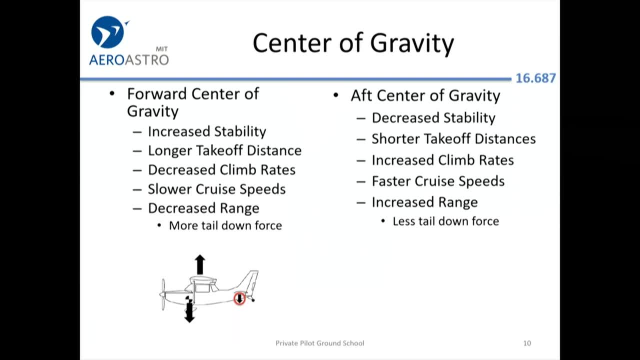 with one exception, which is the stability of the handling of the aircraft, And obviously, if you load it up so much in the back that you can't push the nose over, that would be outside of the CG range or well outside of the CG range. 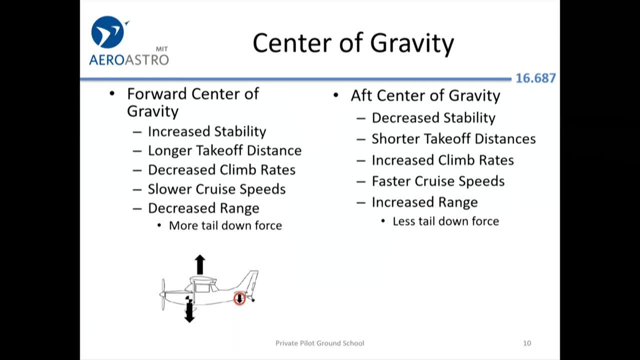 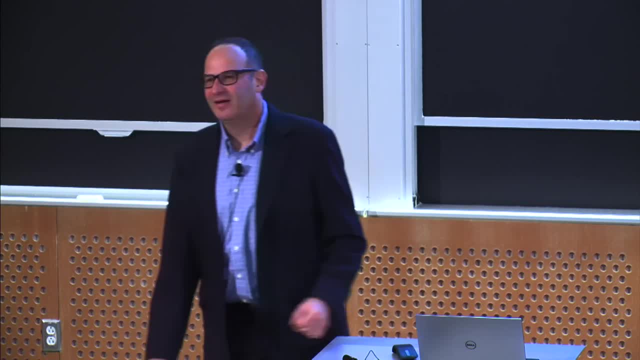 Let's hope. Then you wouldn't even be able to control the aircraft because you can't get the nose down enough. So having that forward CG gives you more stability. That's where you're going to be when you're a student pilot. 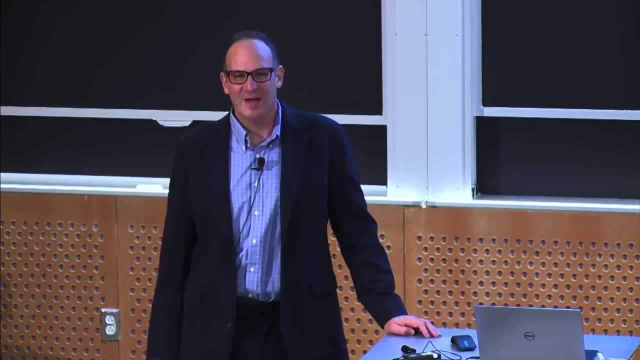 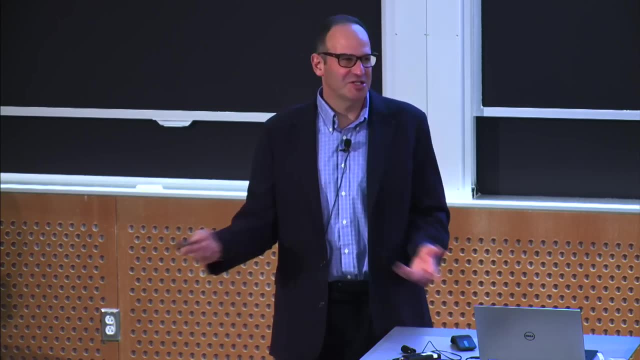 If you're in a four-seat aircraft and it's just you and the instructor in front and the back seats are empty, then it's pretty obvious that that's going to be a somewhat forward CG, because the aircraft is designed to hold at least. 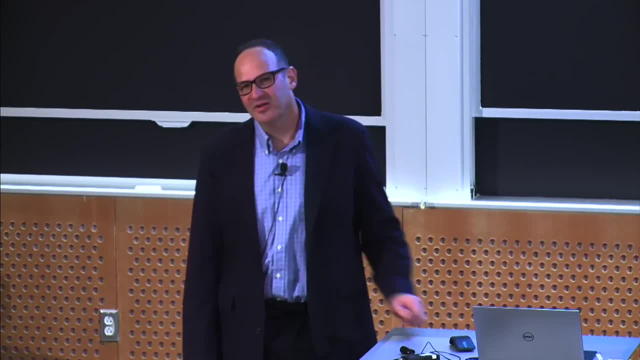 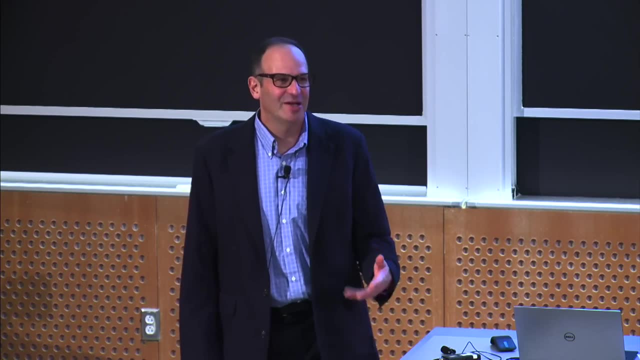 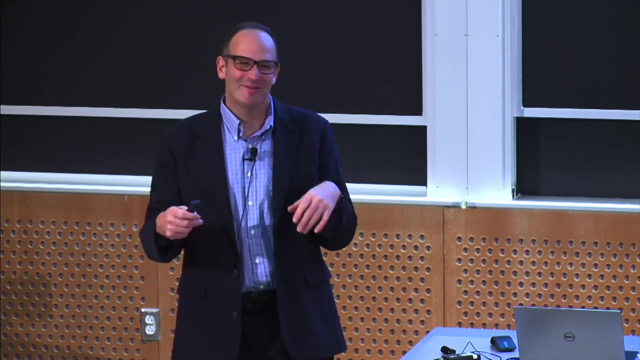 some weight in the back seats. One thing you can do is, just as a first approximation- pay attention, We're going to have a talk on weight and balance later from Tina. But just keep in mind that the aircraft is kind of designed for two adults in the front and maybe one adult in the back. 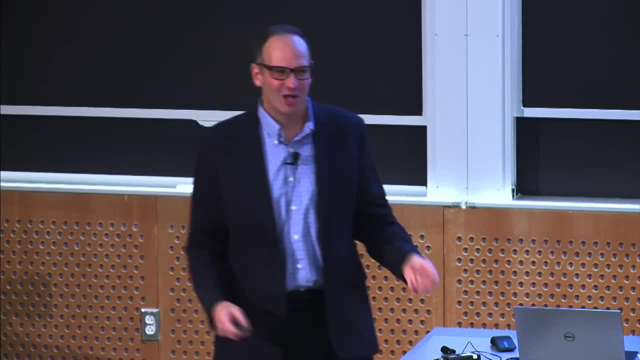 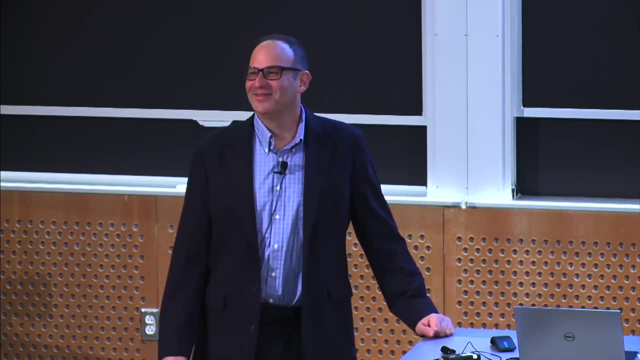 or two kids in the back. So if you load it up that way, it's almost always going to work. If, on the other hand, you have a big heavy friend and his other big heavy friend or his box of anvils, 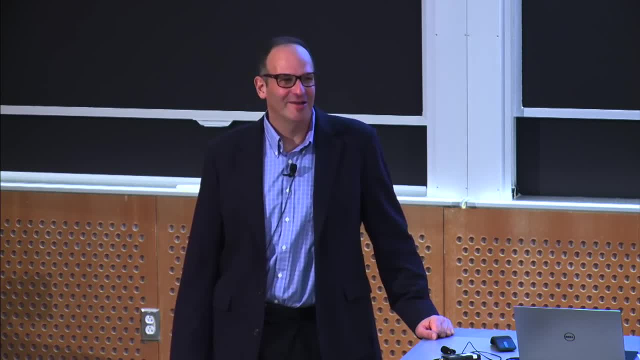 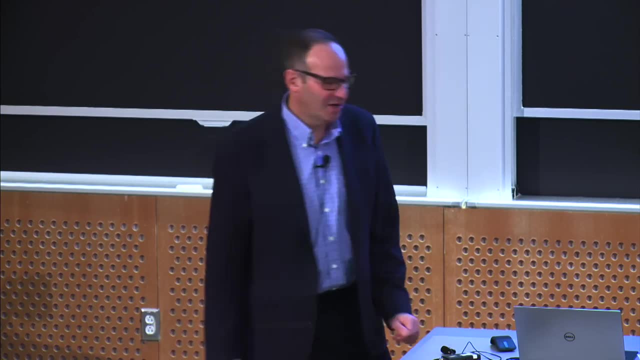 and the guy says: well, look, I just want to sleep in the back, I don't want to be out front and get distracted, And you're a lightweight person all by yourself in the front. That's a situation where it's important to really do. 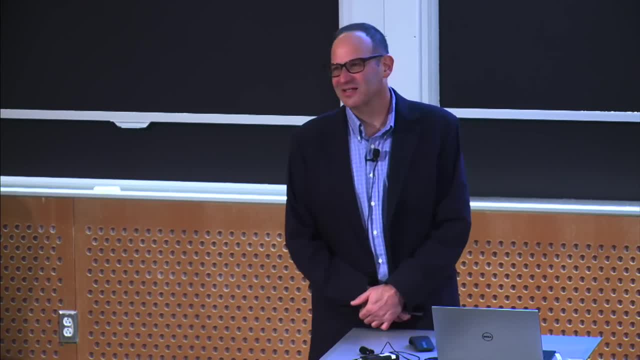 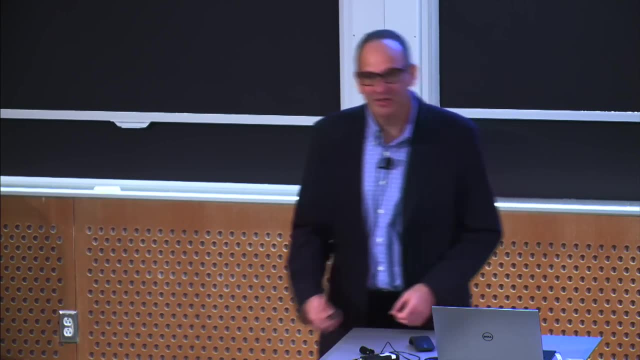 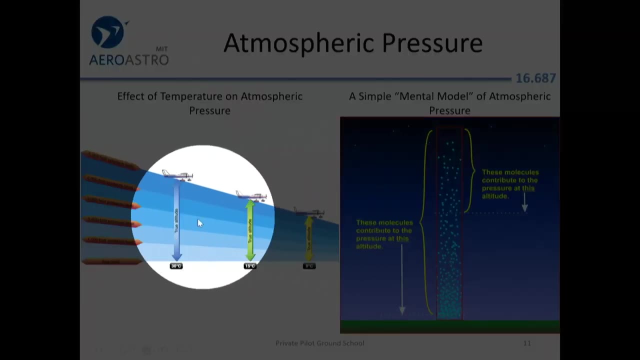 the calculations and think carefully about it, because that wasn't something that Cessna and Piper were thinking about when they designed the aircraft. OK, atmospheric pressure. So a simple remember. we talked about how the atmosphere is going to be expanded when it's hot. 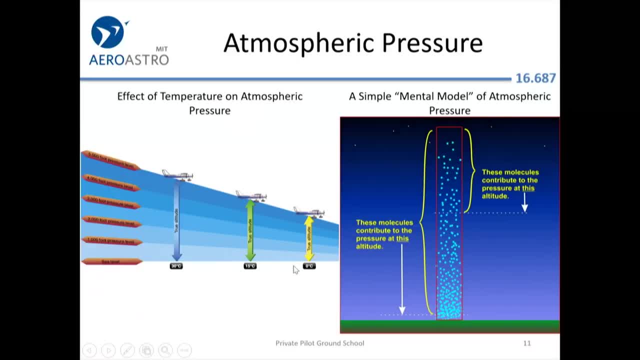 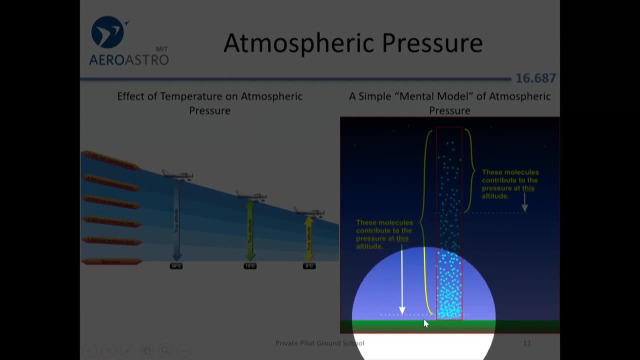 and contracted when it's cold And the altimeter is really telling you how much of the atmosphere you've climbed up through. So you can see here on the right, if you look over here and you're measuring your altitude, you're basically getting this whole stack. 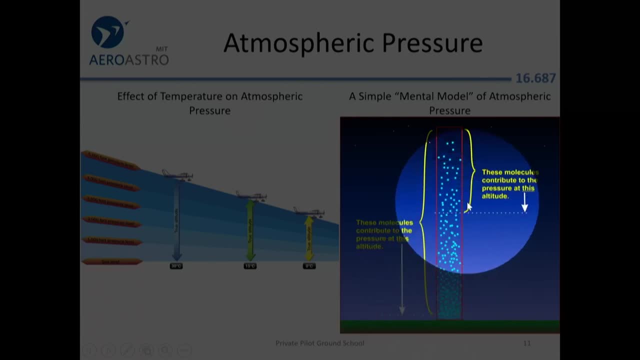 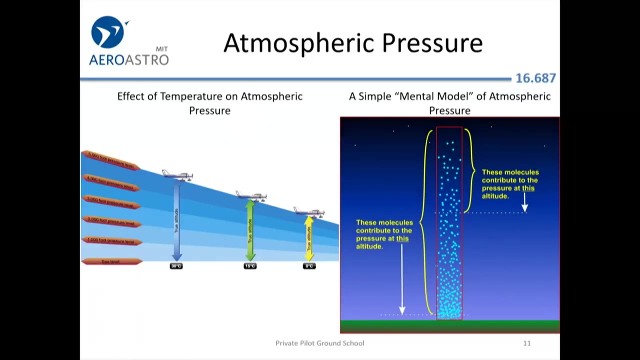 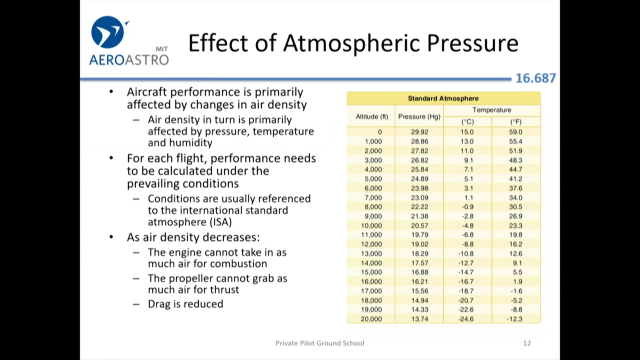 of molecules contributing to the pressure, whereas if you're up high in the stratosphere or something, only a handful of molecules are on top of you, putting pressure into your altimeter. OK, here's that standard atmosphere again, So you can see it's 299, or 2 and 15 degrees at sea level. 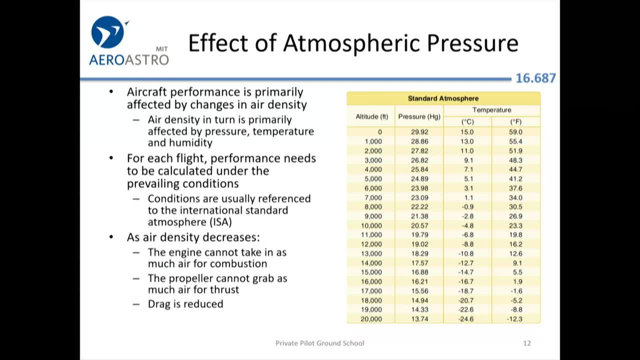 So the aircraft performance is hugely affected by changes in air density, which themselves are affected by the prevailing pressure, which is mostly a function of altitude, the temperature and the humidity. Usually the conditions are referenced to the ISA, the standard atmosphere. 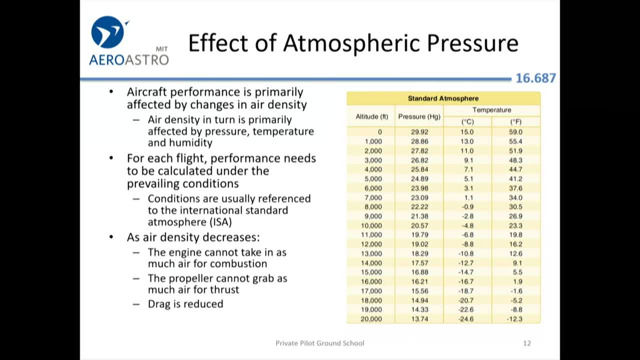 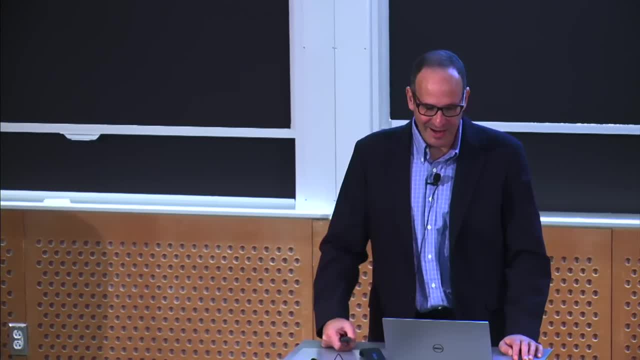 If it's the summertime it'll be ISA plus 15 or ISA plus 20.. And if it's the wintertime it might be ISA or ISA minus 20.. When the air density is reduced and they're fewer molecules around the engine, is not taking in as much air for combustion. Remember that the jet engines are normally aspirated and the piston engines also that are without a turbocharger. they're just trying to burn up a fixed volume of air And that's going to correspond to a different number. 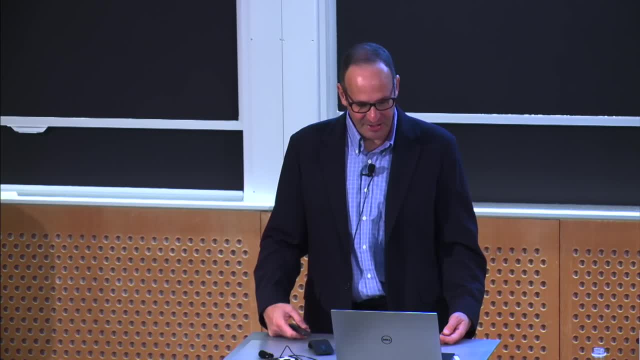 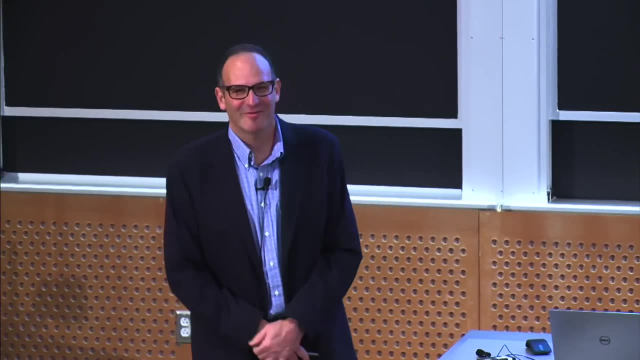 of molecules of air and fuel, depending on the altitude. The only good thing about going up high: the propeller is also not grabbing as much air for thrust. The only thing good about going up high is that drag is reduced and that's. 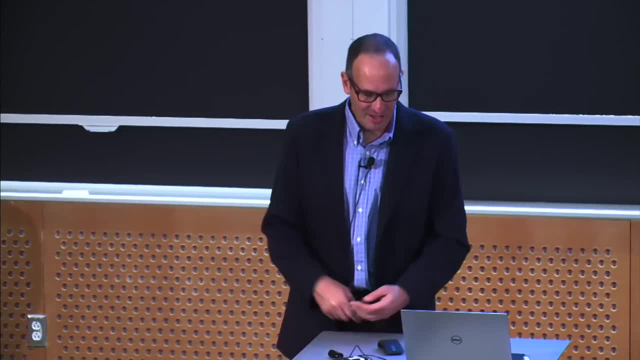 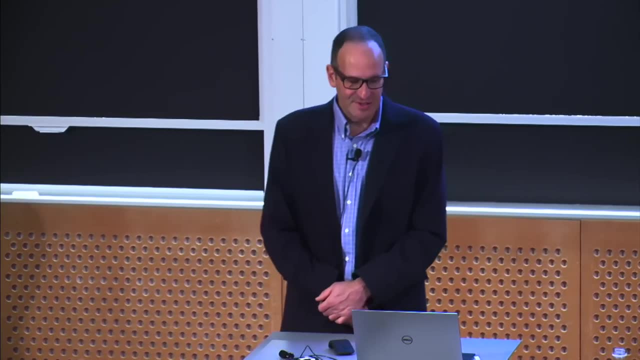 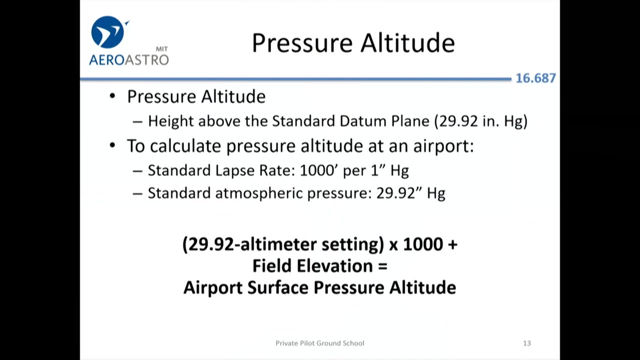 why you see the airliners up high. They go faster and they save a lot of fuel. OK, some definitions. The pressure altitude is just the. it's going to be your height above sea level, with the altimeter set to 299 or 2.. 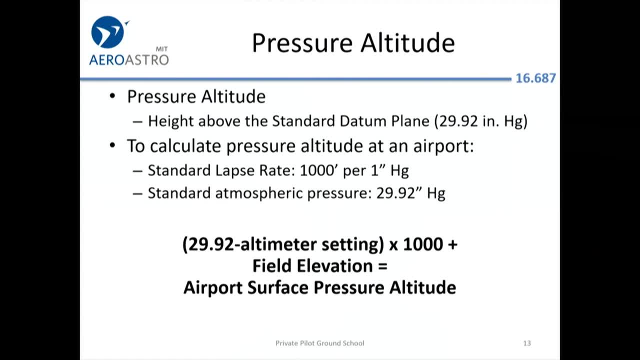 You just have to take the 299 or 2 minus the actual altimeter setting that's being published. multiply that by 1,000.. So a full inch of altimeter adjustment, like from 299 or 2 to 309 or 2, would. 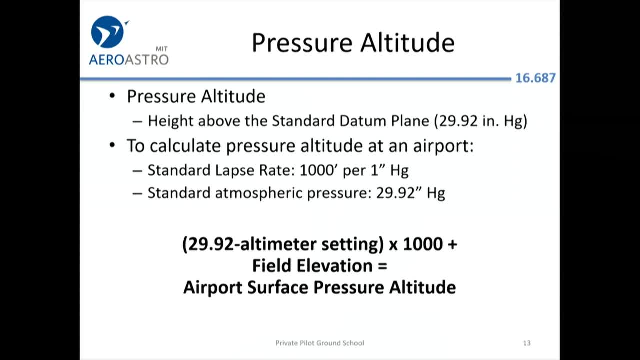 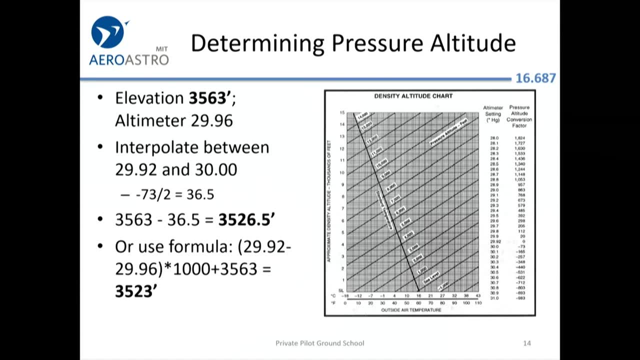 correspond to 1,000 foot difference in pressure altitude And you can calculate that by a chart. Here's a chart that they give you if you don't like the formula. So they're saying this is something again you might have to do on a test. 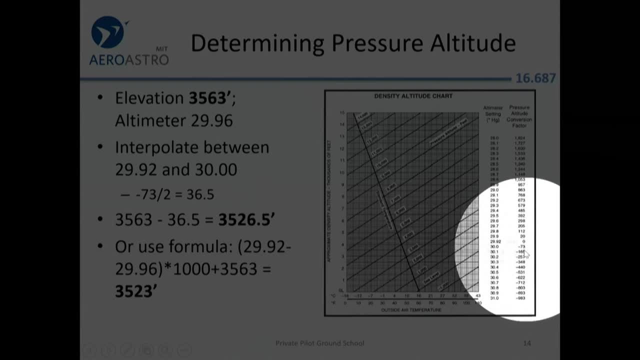 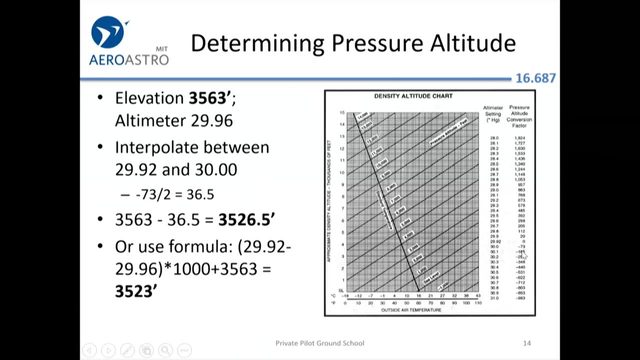 They'll say: OK, 299 or 2,, the correction is 0.. At 3,, 0.0, the correction is minus 73.. So up here you can see, we've got this formula where we interpolated between the two. 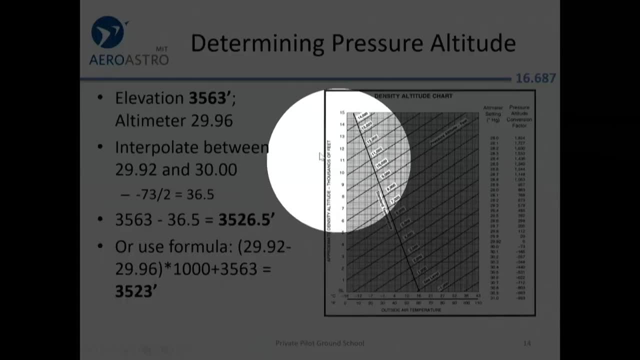 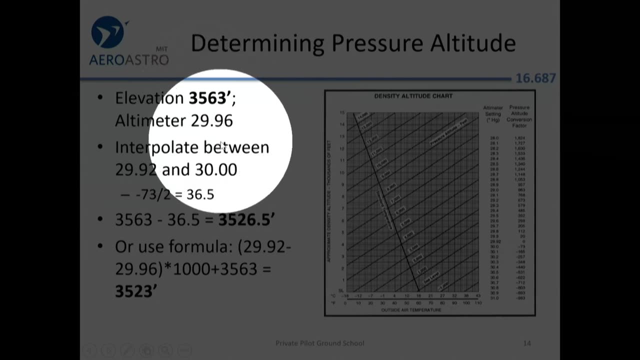 to try to figure out. what would the pressure altitude be If we start with a field elevation of 3563, and the altimeter is 299 or 6,, which is just a little bit nonstandard. we would expect a 40-foot difference. 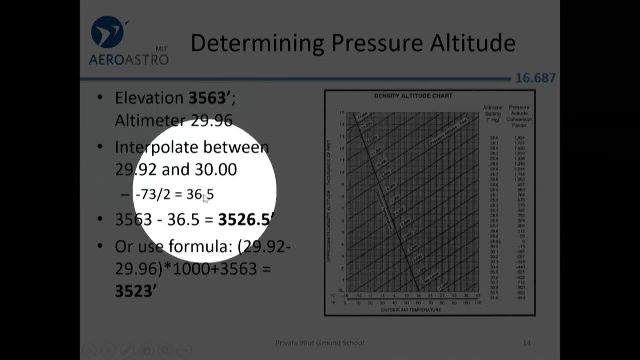 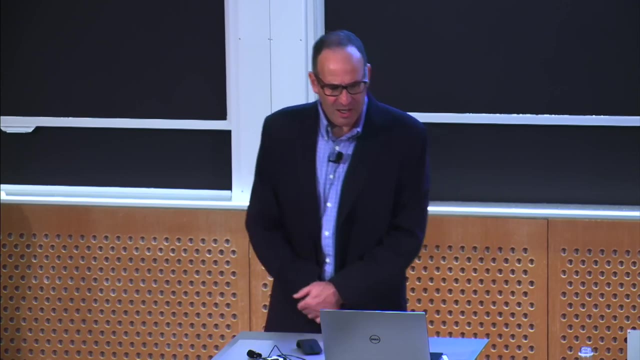 If we look at the table and we interpolate, we come up with a 36.5-foot difference And we find out that the airplane feels as though it's only at 3526 feet above sea level, assuming the temperature matches that ISA standard. All right. so density altitude is a lot more important And oftentimes it will be reported on the ASOS or ATIS, So the airport will actually tell you density altitude is 3,000 feet or 2,000 feet or whatever it is. 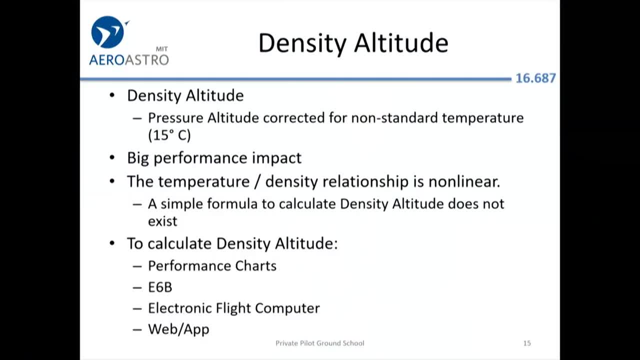 That you get from correcting what's usually a relatively small correction for pressure altitude compared to the actual altitude, but correcting it for the nonstandard temperature. I think, as I said earlier, flying is a lot more popular in New England in the summertime. 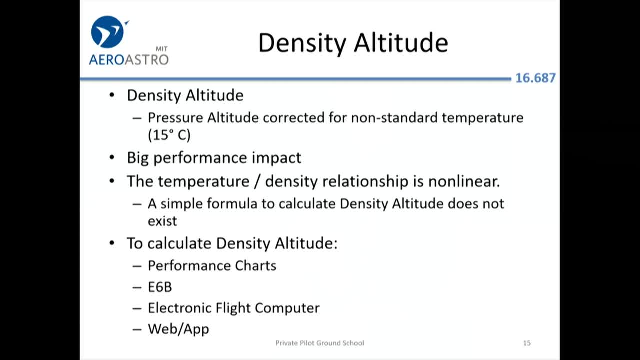 than in the wintertime, So it's usually warmer than standard Density. altitude has a huge effect on performance And it's a nonlinear relationship. So you have to look it up in a table or calculate it with the E6B. We'll see. 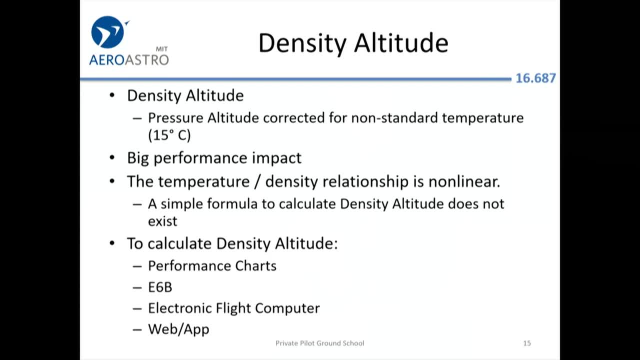 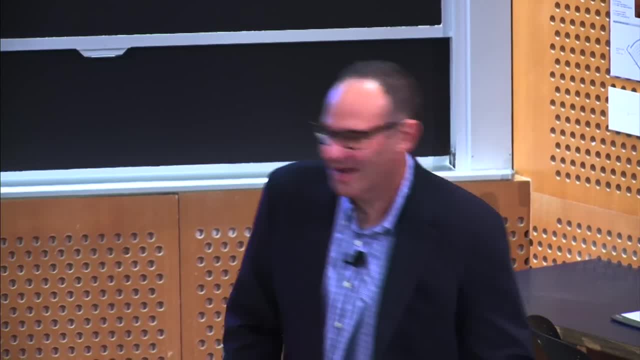 Maybe I'll play around with the E6B or also people can look at it during breaks. I have the slide rule and the manual right here And I think I will try to get the document camera going So maybe I can show you guys some exciting slide rule. 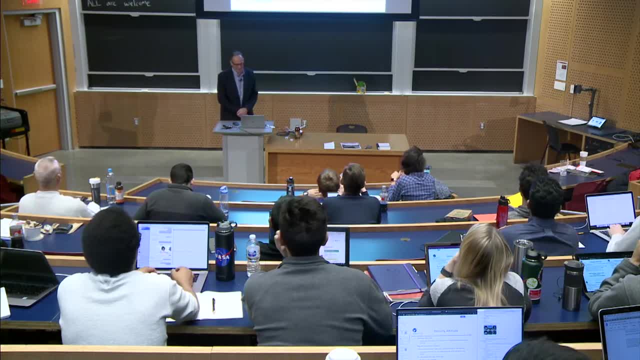 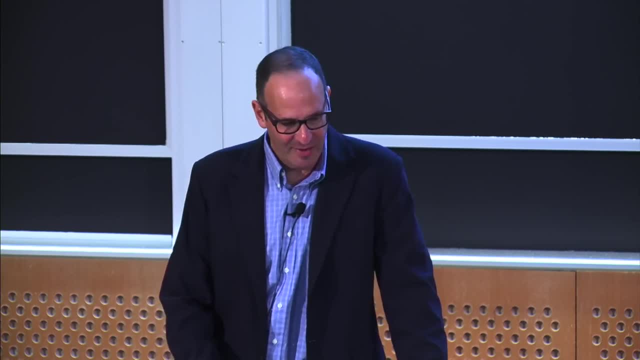 activities. OK, so you can calculate it though using the E6B, like I said, using charts, And there's various. OK, There's a web and app way of doing it. So the density altitude: here's a chart. 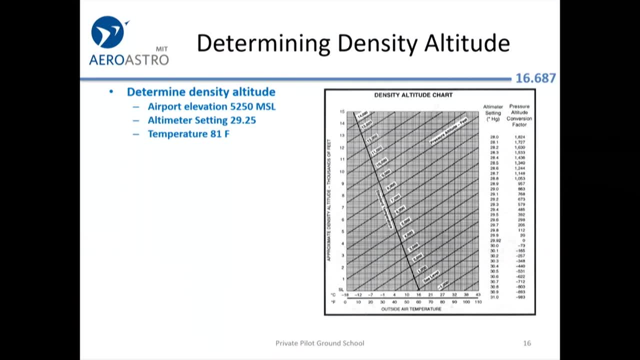 So, again, this is the kind of stuff that's on the written exam. You guys are all pretty good at working with charts and tables, So I'm sure you won't have any trouble. They're giving you these initial conditions up here on your left. 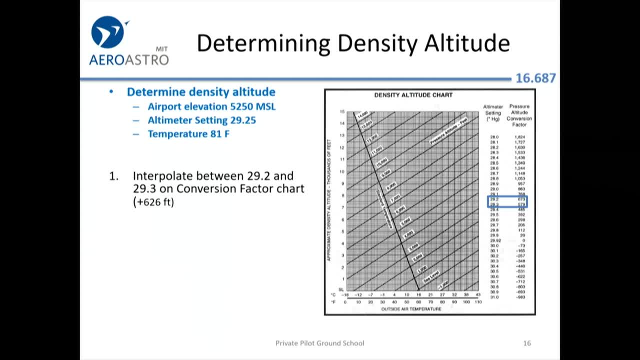 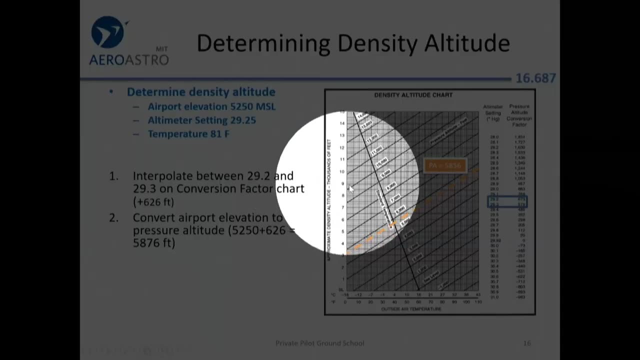 So you look to find where the pressure altitude is on the chart And it says to add 626 feet, which is interpolating between those two. Then you've got this pressure altitude line of going from here down to here at 58, 56.. 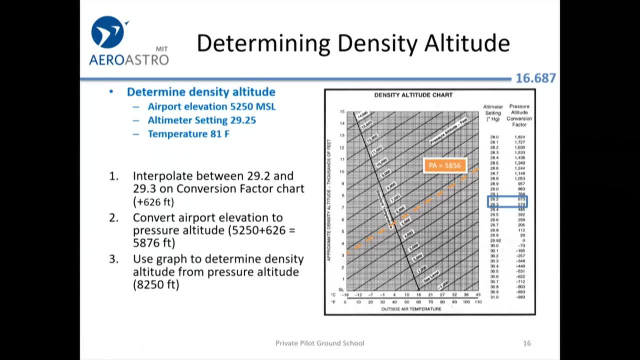 And now we've got to correct that for temperature. So here's our temperature of about 80 degrees, 81 degrees, And then we go over to the left And we can read that. I think I told you guys that in the summertime usually the density, altitude 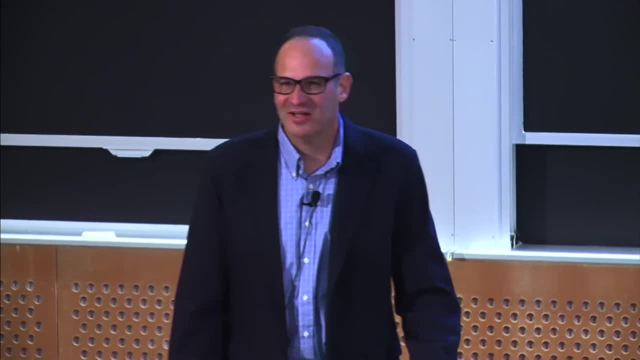 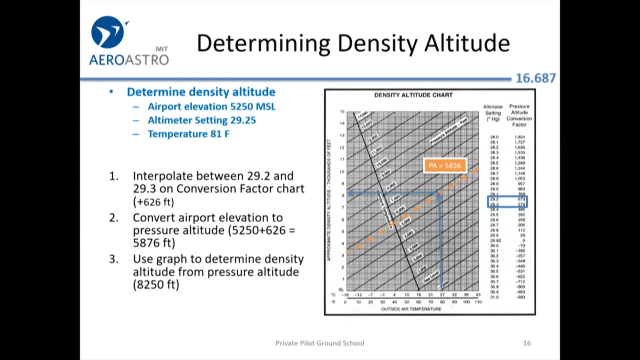 is about 2,000.. 2,000 feet higher than the pressure altitude. And, sure enough, here it's 8250,, which is about 2,400 feet higher than the pressure altitude. So the density altitude gave us a little more. 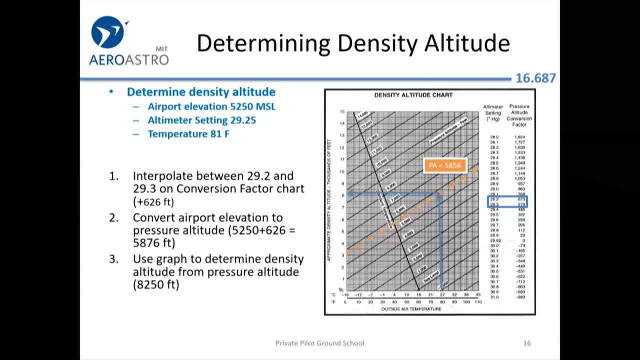 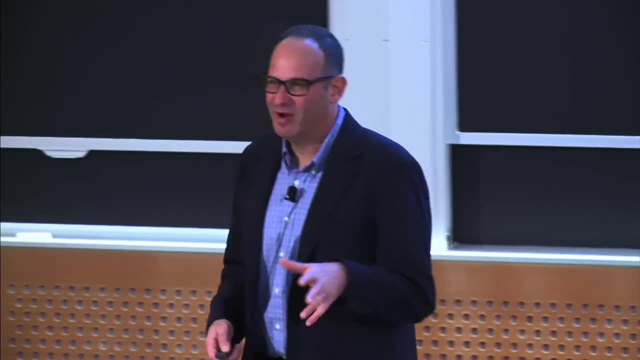 than a 2,000-foot boost for that nonstandard temperature. The reason it's so much, I guess, is it's not 80 degrees at sea level. It wouldn't be that high above the sea. It's a standard temperature. But 81 degrees Fahrenheit at a mile above sea level is quite a spectacular temperature compared to the standard atmosphere. Let's go back to the standard atmosphere. Yeah, so at 5,000 feet it's only supposed to be 7 degrees Celsius. 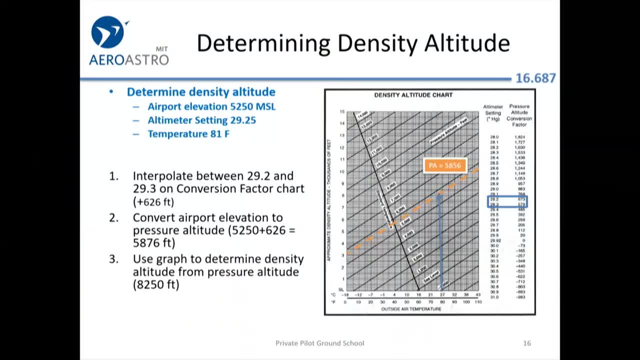 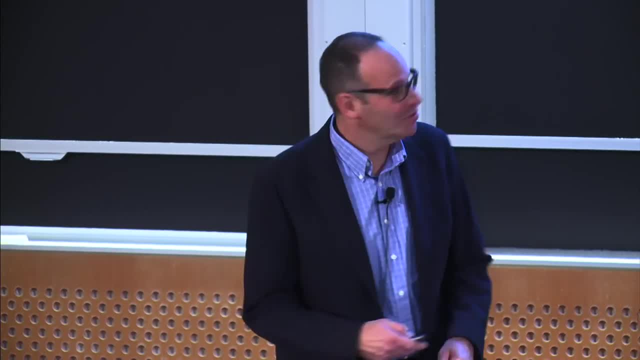 And here we said it was about 27.7.. So that's ISA plus 20,. just like I said, If you look at a lot of jet performance charts, you have ISA minus 20, ISA and ISA plus 20.. 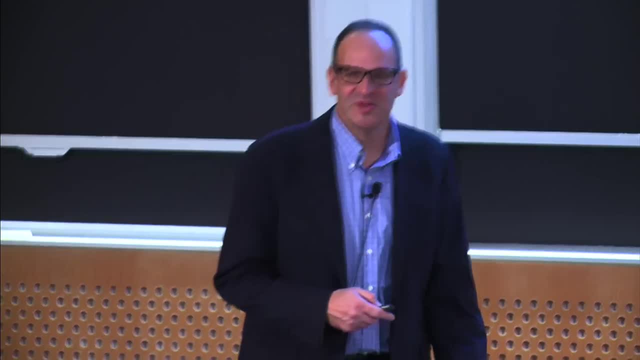 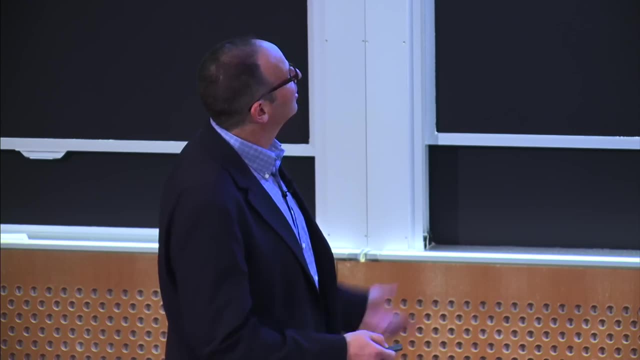 Flight computer demo. if there's time, Let me just futz with that. at the end of all this I'll give you an E6P intro. When are they the same? I think this is an FAA test question- When the temperature distribution is the same. 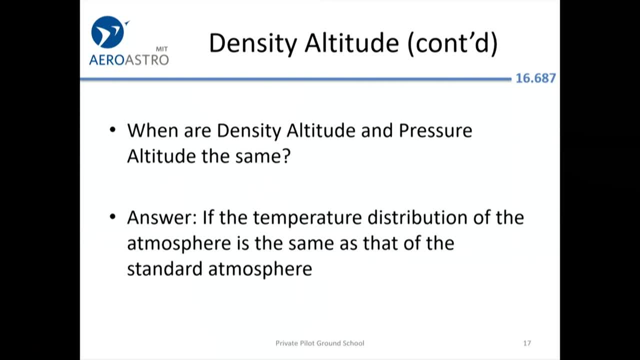 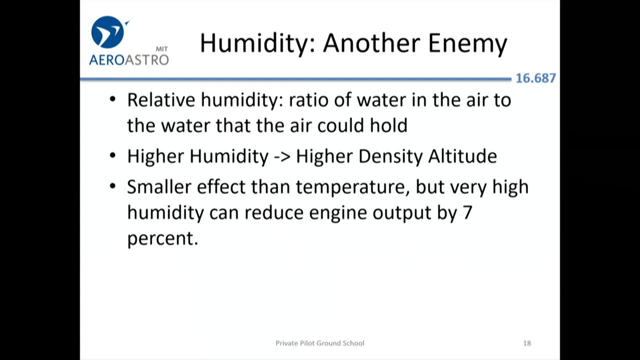 It's the same as that of the standard atmosphere. OK, Humidity is also another enemy. a little bit more surprisingly, The water vapor molecules in the air actually reduce the density of the air. You might think that they would increase it. I don't know. 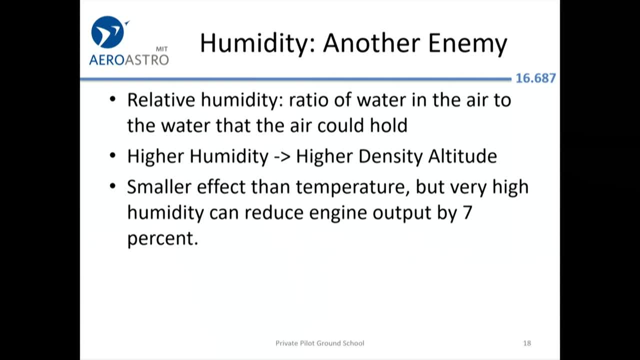 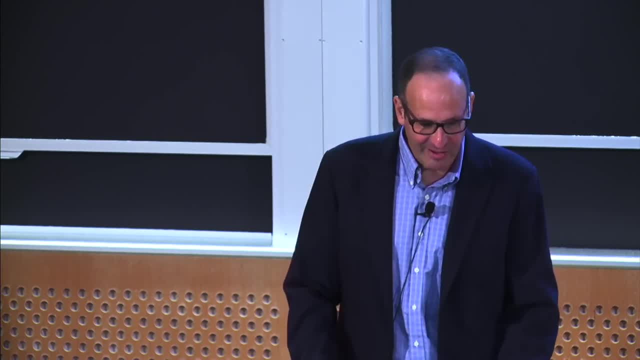 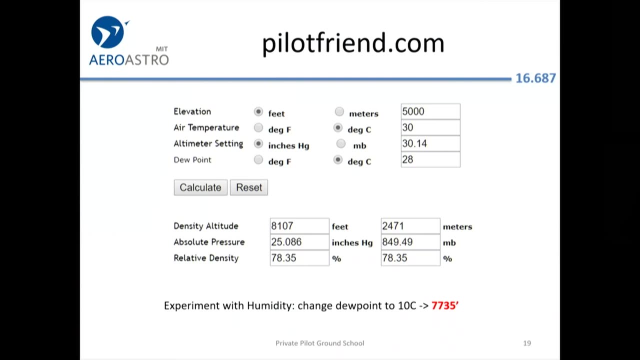 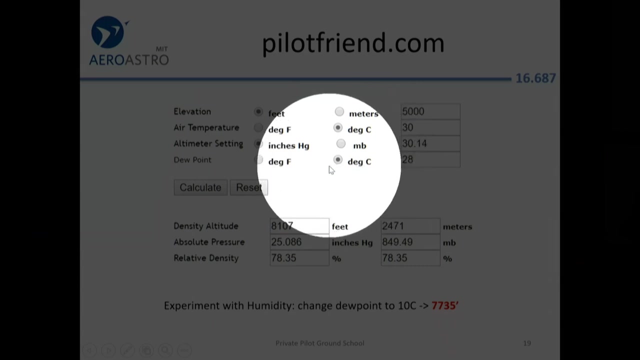 This is not something that we normally correct for. However, there is this nice web calculator that I found for free on pilotfriendcom And you get to enter the relative humidity of the air. Where is that? We have the air temperature. Oh, we have the dew point, right. 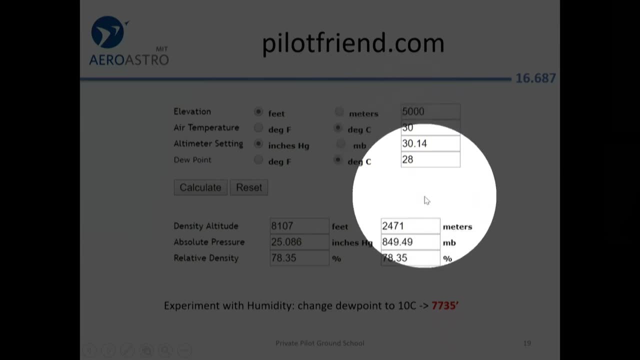 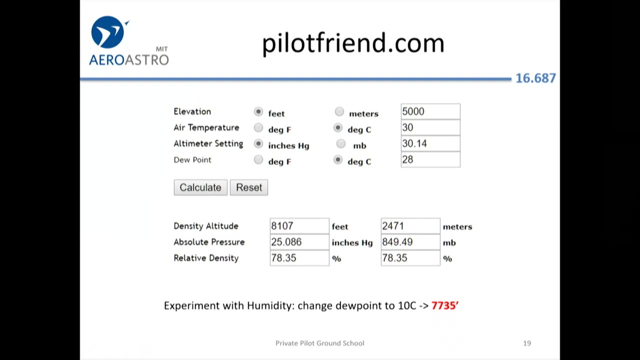 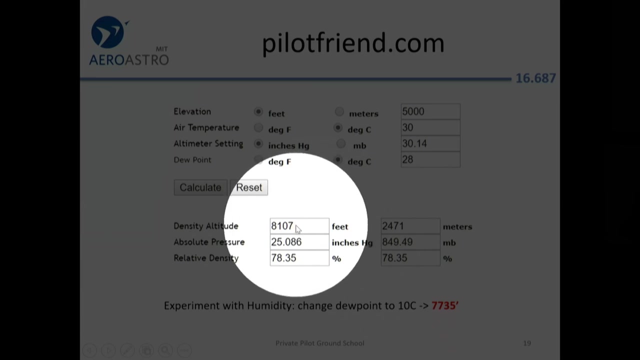 So we said it was a 30-degree temperature and a 28-degree dew point, So that's a pretty narrow spread And therefore it's a pretty high humidity day. So they say, well, it's 78% humidity And we're correcting that up to 81.07.. You can play around with this on your own. If you reduce the dew point to 10 degrees Celsius, which is going to be really dry, 30 to 10 split is a nice dry day out west or here, occasionally a crisp day. then it's only 77.35.. So the change in humidity had about a 300-foot effect on the altitude, But the change in temperature was nearly 3,000 feet. OK, The maximum convenience way to do this is with apps, So ForeFlight, for example, will just tell you. 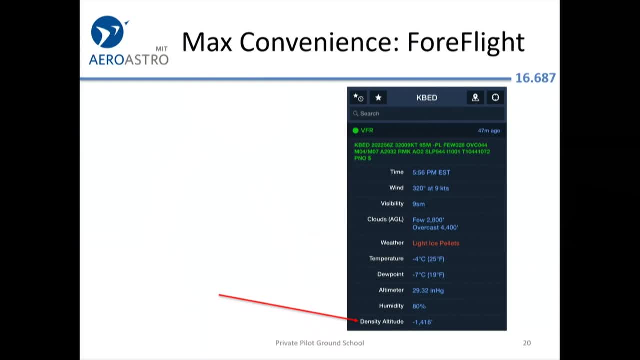 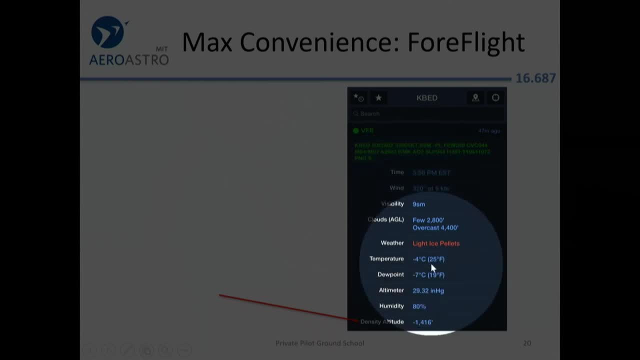 the density altitude. This was, I think, Sunday night at Bedford. Let's look at this beautiful. I don't know how many people will come to New England now. So Bedford's approximately at sea level about 130 feet above sea level. It was minus 4 degrees And the density altitude was minus 1,400.. So we were like flying, You know, skimming the surface of the Dead Sea or something in terms of performance. So the airplane will be really happy about flying. 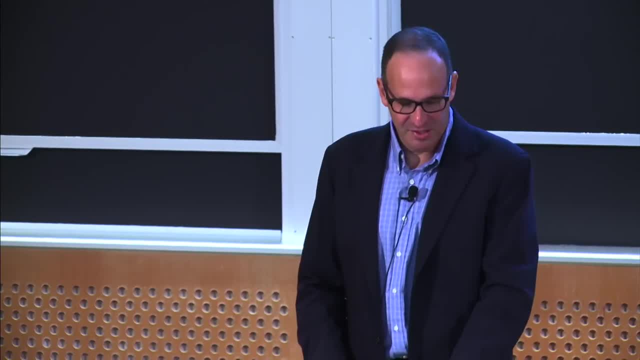 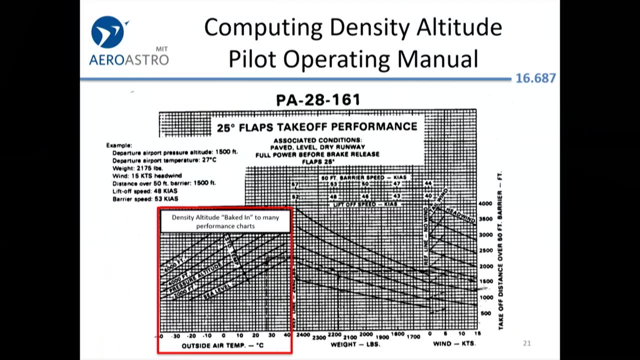 all winter time And it'll climb better than the book. most of the numbers in the book, OK. The density altitude is often just kind of baked into the performance chart. So here is. pipers normally take off with no flaps, But if you want to get off the ground really quickly, 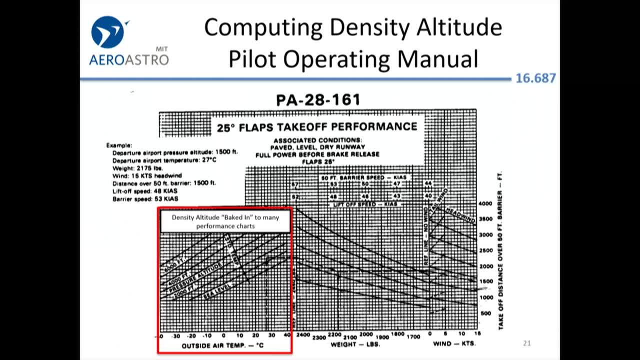 like taking off over grass or mud or something. you can put down the flaps and try to have less time on the ground and not be going so fast over the ground. Your ground roll will be shortened, Anyway. so here they don't actually. 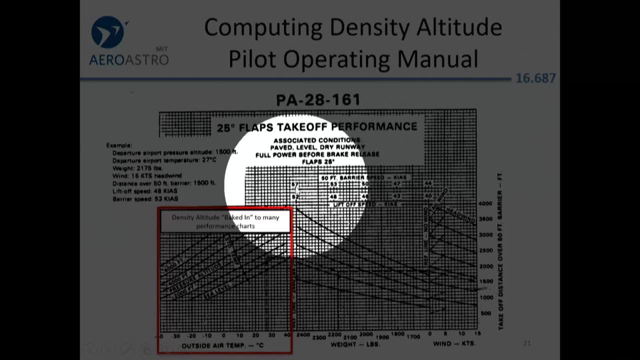 ask you to ever calculate the density altitude, They just say, OK, it's almost 30 degrees outside And it looks like we're up here at about 1,500 feet. So we'll start here on the performance chart, These people are virtuous. 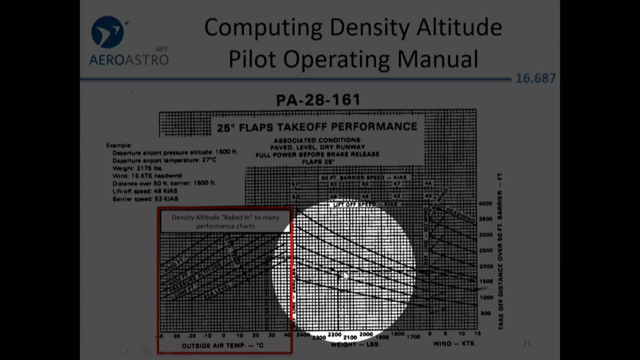 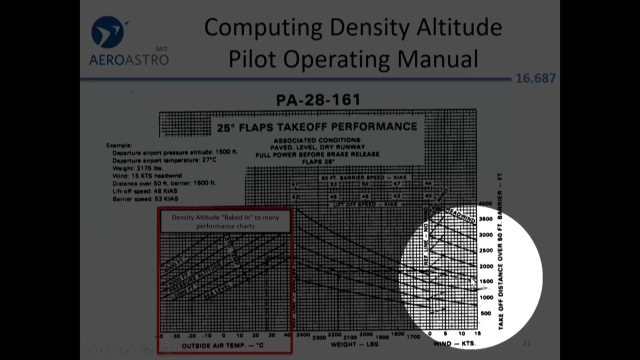 They only weigh 20.. They're 175 total. So we come down a little bit And we can go over here And we find that it's going to take- is there a wind here? 15 knots of headwind. So we come down this graph. 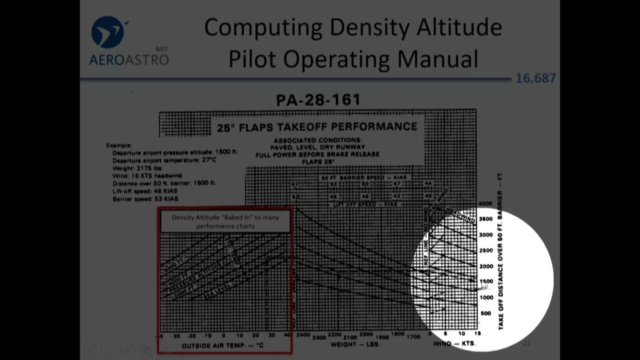 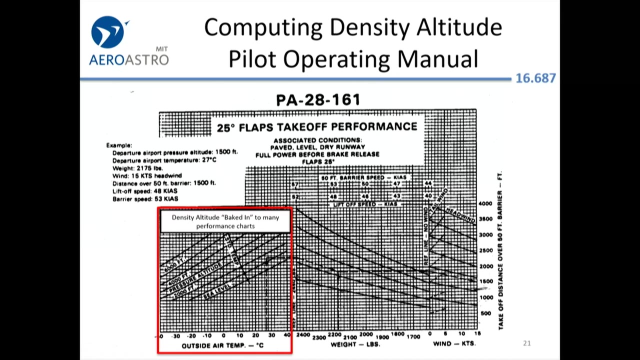 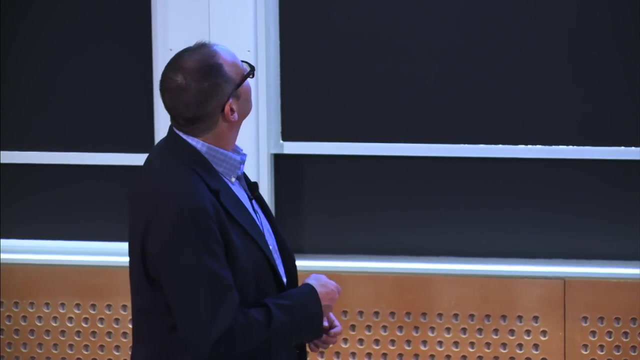 And we find that it'll take us 1,500 feet to take off over a 50-foot obstacle. Fair enough, So anyway, we never figured out what the density altitude was. It was just something that affected where we started on the chart. 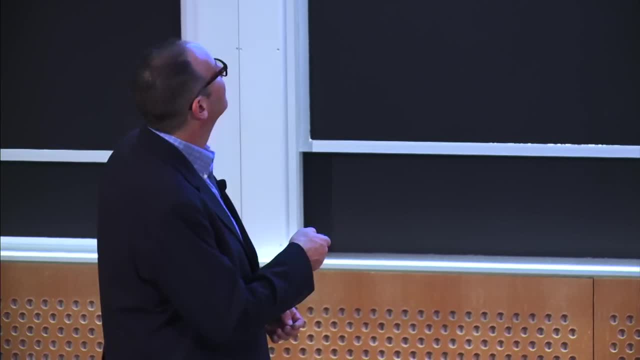 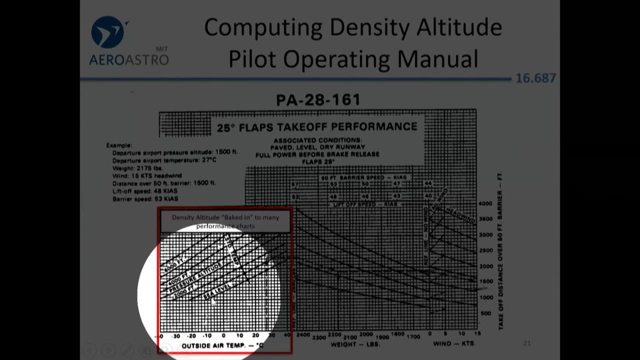 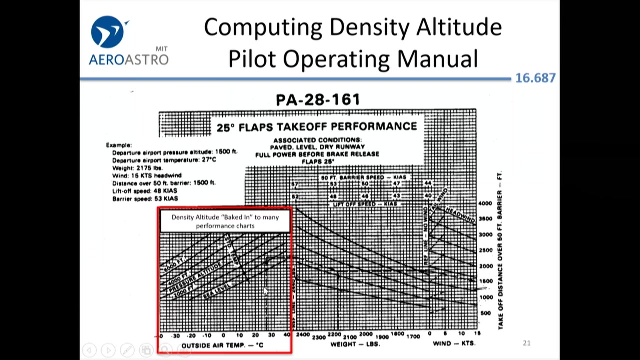 I guess maybe it's implicit in here. I think it is implicit, right, Because we're starting up high. Maybe somebody who's smarter can figure this out. Yeah, so sea level at zero. Yeah, I think we can pull it out of those graphs. 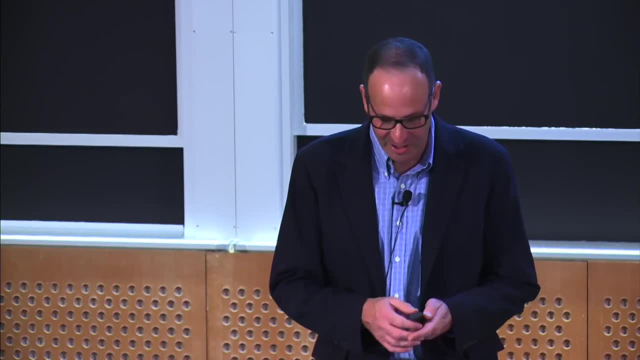 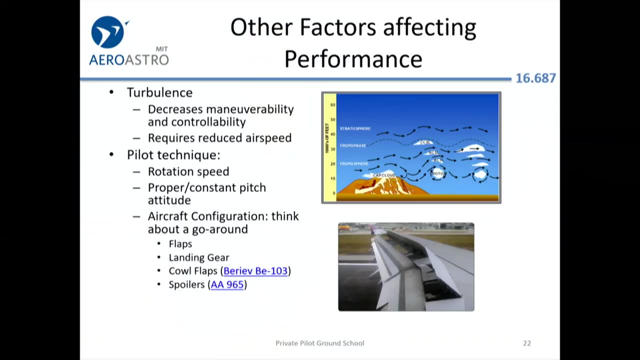 But nobody would, because what you're really interested in is the number of how long you're going to be on the runway. All right, You'll have to slow down if you're in turbulence. So if you plan for some kind of flight, a certain amount of time, 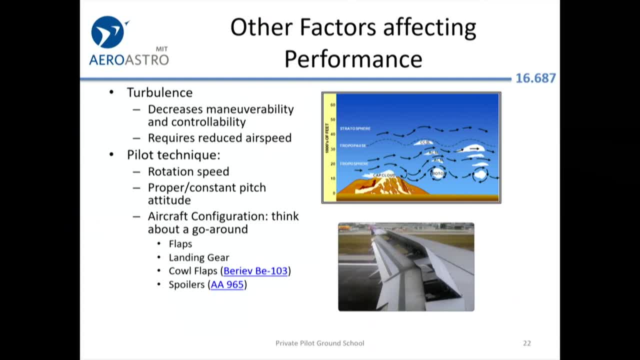 and it's going to be very bumpy. remember we talked about maneuvering speed. Depending on your weight, you'll have to slow down to avoid bending the aircraft. Or you know, turbulence is severe enough to bend the air craft is extremely rare. 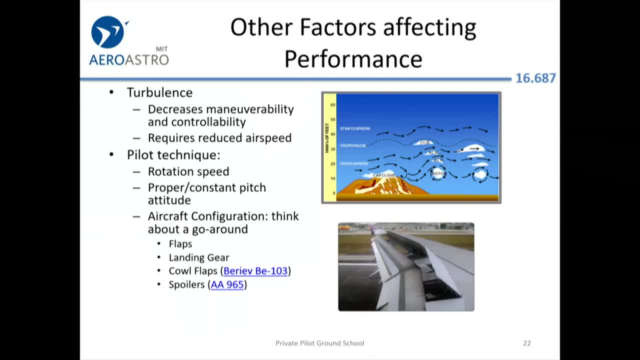 But turbulence that's sufficient to make you and your passengers unhappy is a lot more common, And in both cases you pull way back on the speed. So in the Pilatus, for example, you'll pull back to 150 knots from 200 knots. 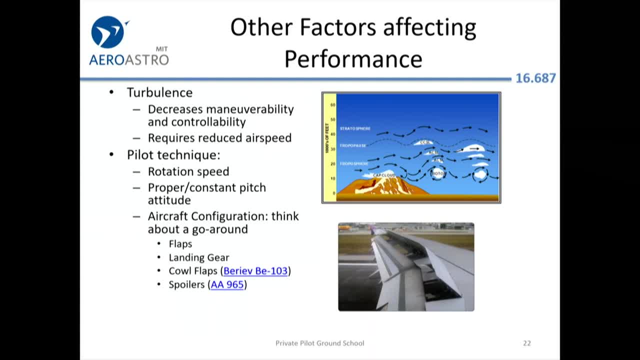 In the Cirrus you might pull back from 130 down to 100. And in a helicopter you'll pull back from 110 knots to maybe 70.. OK, Pilot tech Technique. So all the book numbers depend on the pilot. 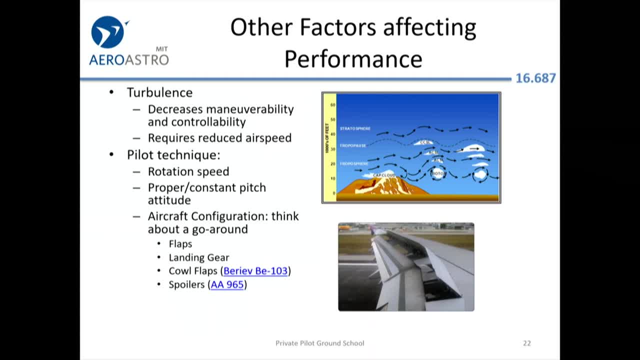 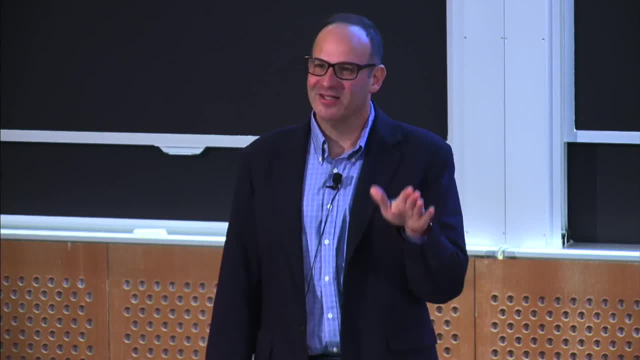 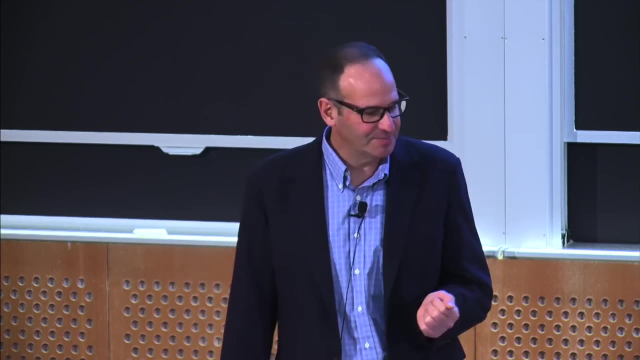 doing what the book says. So think about clearing an obstacle at the end of the runway. That's, depending on the pilot, rotating within a couple of knots of the specified rotation speed, getting the gear and the flaps retracted if they've been deployed. 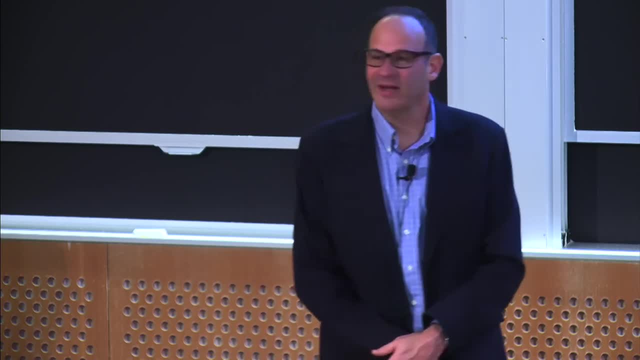 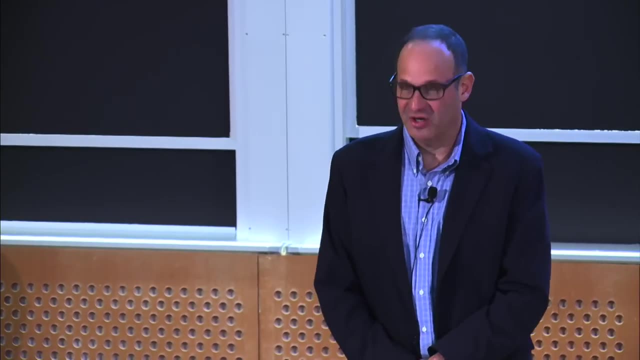 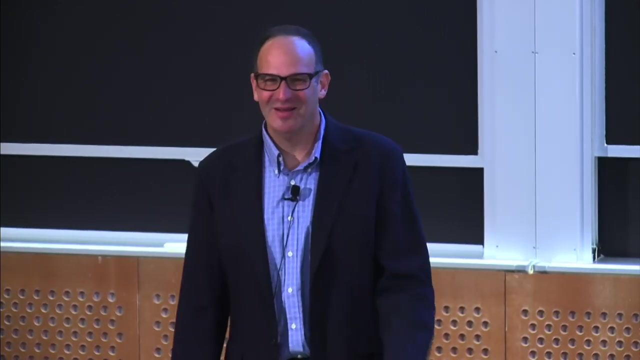 or if the gear are retractable at the recommended air speed and just generally, Having the pitch, attitude and the air speeds where the manufacturer tested the aircraft And think about a go around, You might say, well, anybody can do that. You're rolling down the runway at Hanscom Field. It's a mile and a half long. You're fresh, So that performance is. you're probably going to come pretty close to the book performance. But think about doing a go around. You've just done a two-hour flight. You were trying to land at the airport somehow. 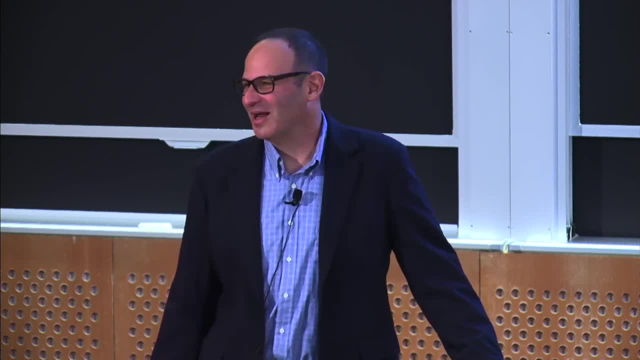 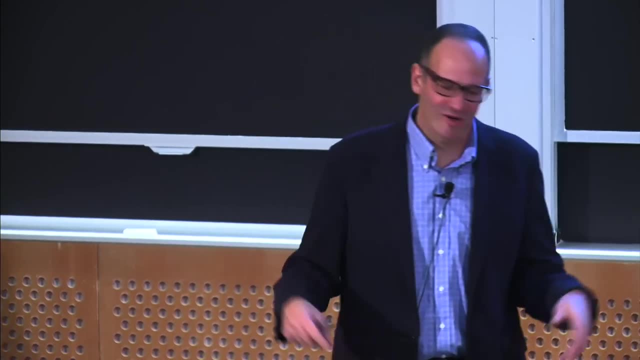 Either There was somebody else on the runway Or you didn't get the approach just right, So you decided you're going to go around and try again. At that point you've got to reconfigure the airplane: change the flap configuration, change the gear configuration. 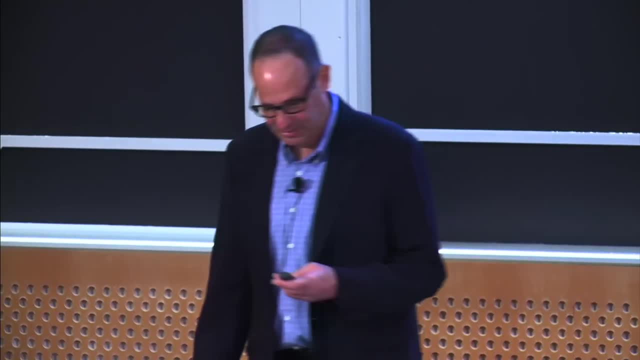 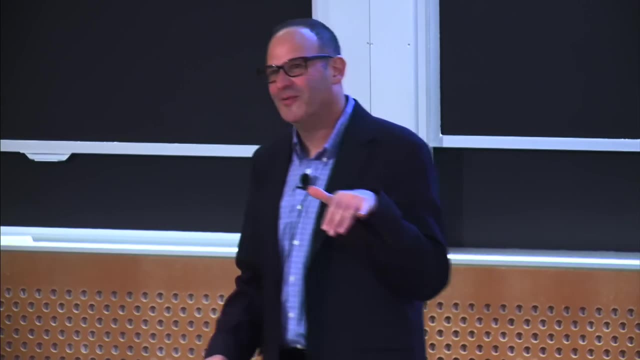 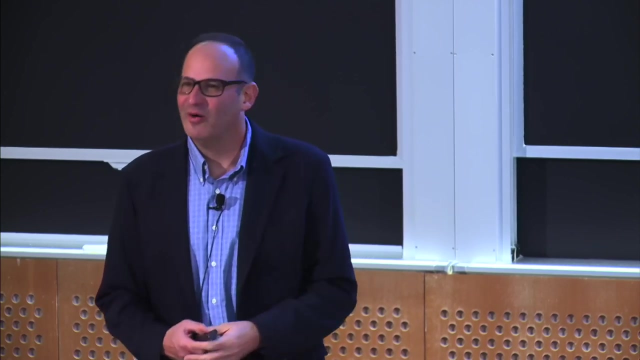 There's a couple interesting incidents that have happened Like. one of them was unfortunately not very interesting for the people involved, But there was an American Airlines flight that got disoriented in Colombia in the clouds And the terrain warning system said terrain, terrain. 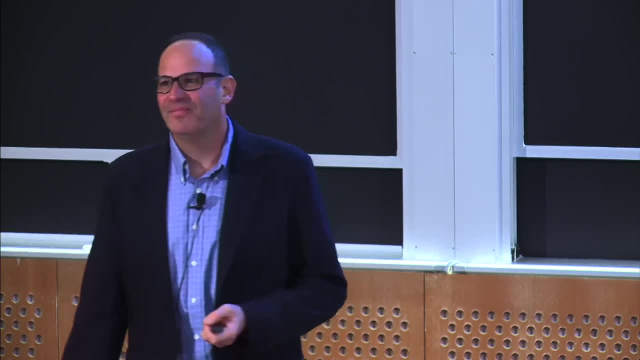 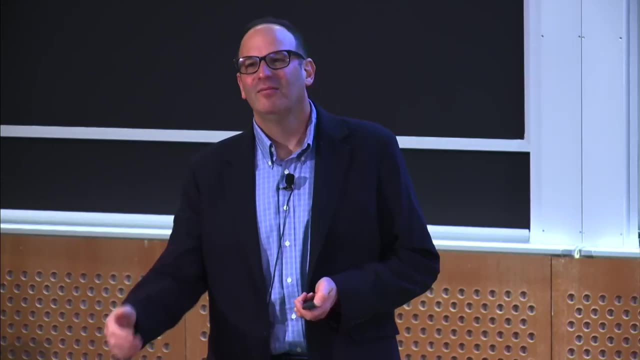 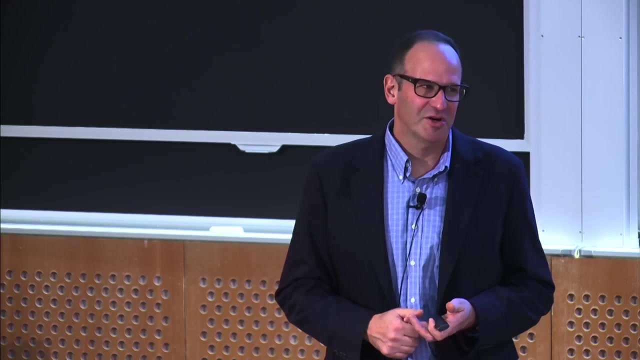 pull up, pull up, And so they advanced the thrust levers. You can follow that link and read about it. They advanced the thrust levers and had maximum power, But they neglected to. they had the spoilers deployed for a descent. They didn't retract the spoilers. 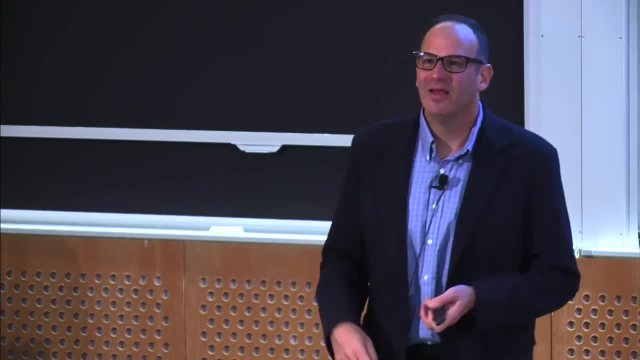 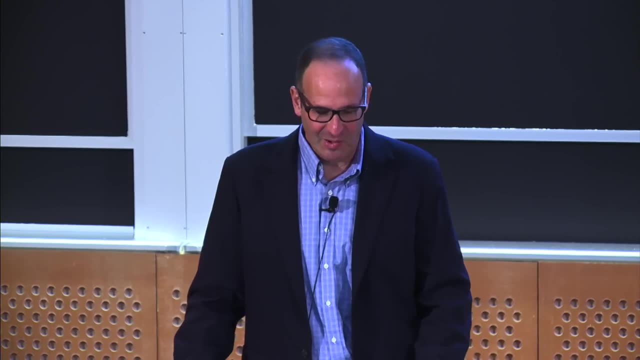 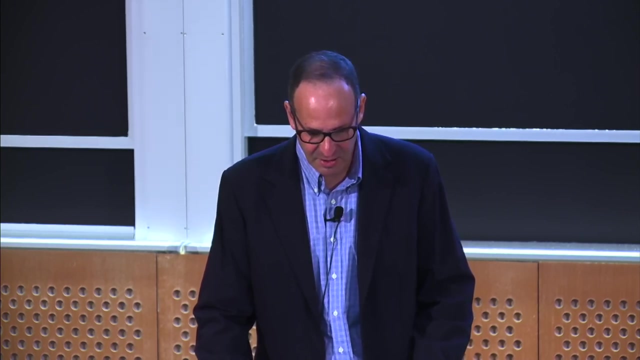 So the airplane was climbing, but not nearly as well as it would have without the spoilers retracted. So that's an example where you know, in a critical situation or a fatigue situation, you may not. I wish I could get this. 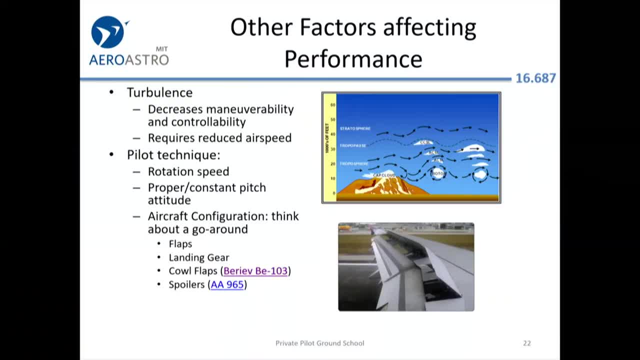 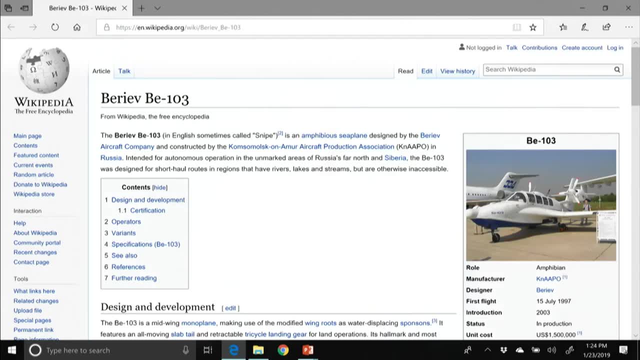 I don't know if I can move this onto the screen. I want to show you a picture of this crazy airplane that I flew, Ta-da. Look at that Russian seaplane. It's got two Cirrus engines in there. I don't know. 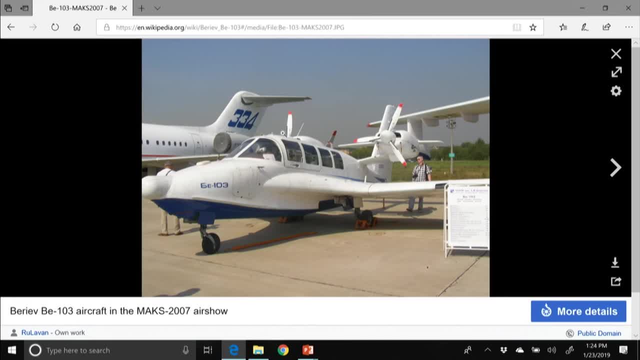 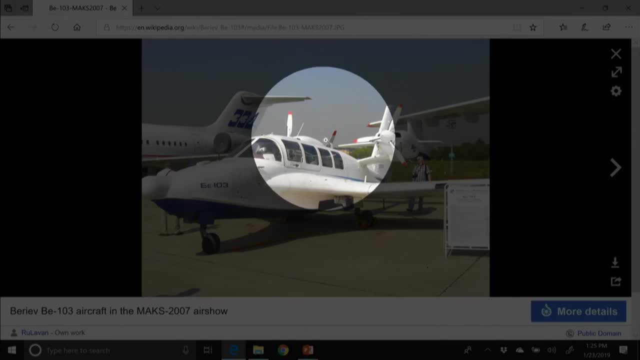 I don't even see the second engine. Well, there it is. You can see that propeller over there. So sorry, There's one propeller sticking up, There's the other one, So it's got two Cirrus engines, 200 horsepower each mounted. 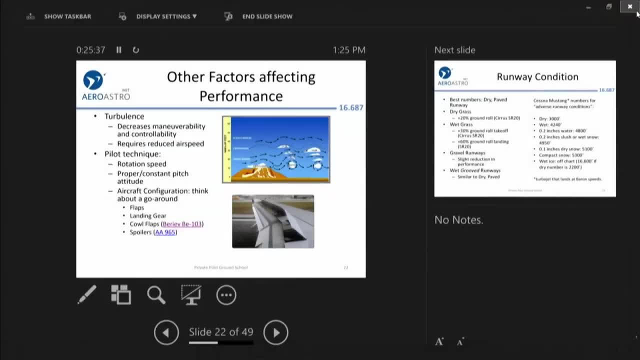 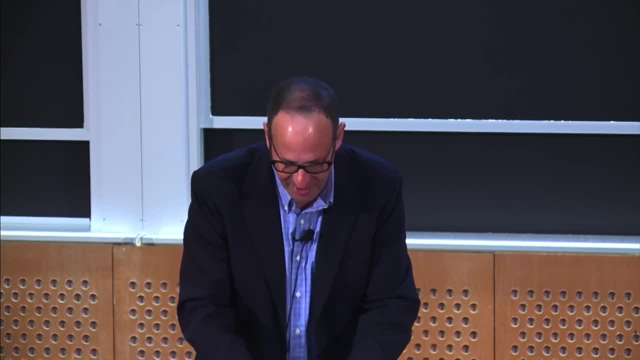 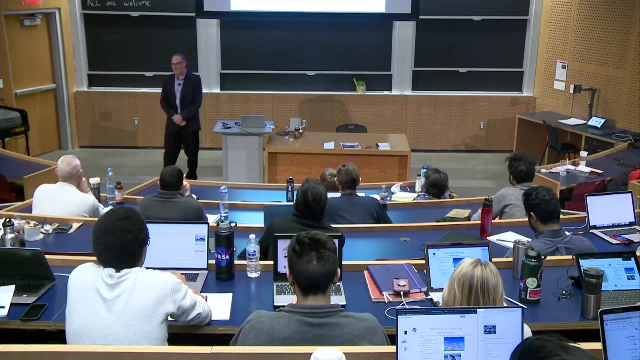 on pods. And if you say, like, how can the airplane climb after an engine failure on one little Cirrus engine when it has, I don't know, I think it could seat seven people, the answer is it really can't. So I tested that airplane out. Because I thought it was cool And I went flying with an airline captain And piston twins aren't really required to demonstrate any kind of climb performance For jets. there are certain minimums On one engine. it has to be able to still climb. 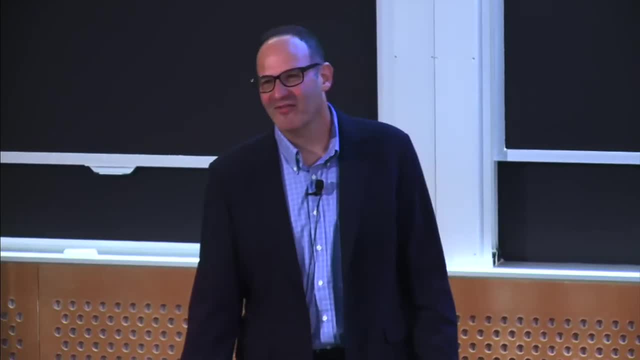 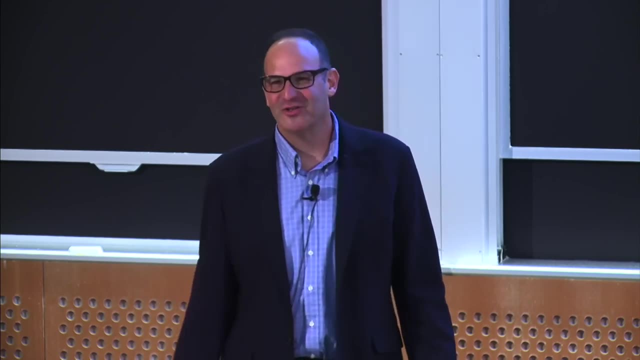 750 feet per minute or something. But for these piston twins the FAA says you should know that you're buying a pig anyway And if you care, go and get yourself a turbine Or don't load everybody in there. But anyway, this Beria thing, it could not climb on one engine. 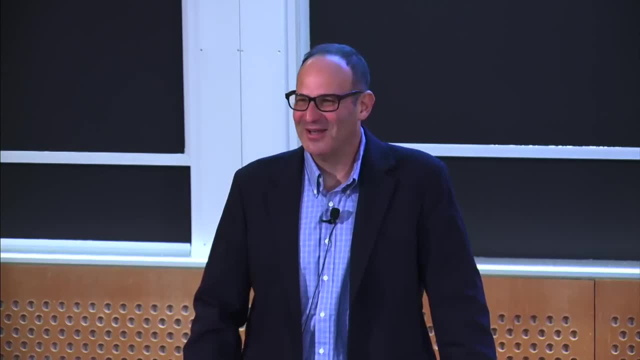 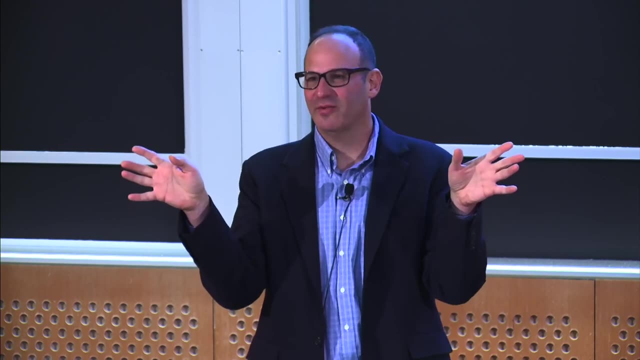 On one engine. We couldn't even maintain altitude on one engine And it turned out that we'd forgotten to close the cowl flaps. It had these extra openings for cooling to provide extra cooling at high power settings, And if you don't close them, there's extra drag. And that extra drag was enough to turn what should have been 150 foot climb rate or something into a 150 foot sink rate or something. So that's another thing that can affect performance. OK, And this really affects your planning: whether you can take off, whether you can land. 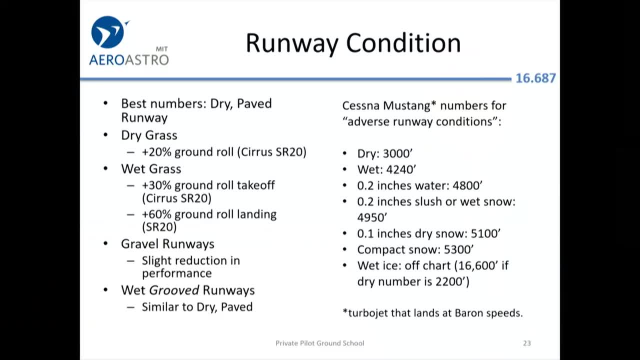 how much weight you can put in there. So, for example, if it's dry grass, you need a longer runway than if it's paved. Alternatively, you can take off at a lower weight. If it's wet grass, you need a lot more room to land. and yet 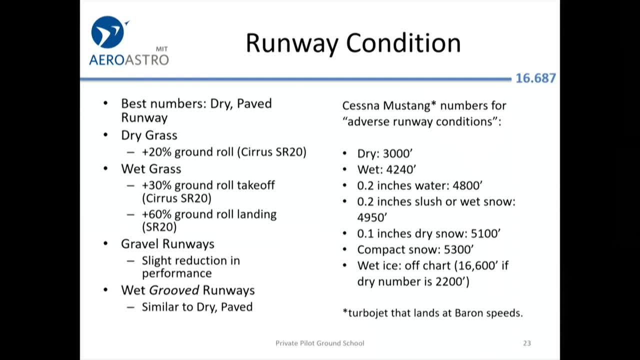 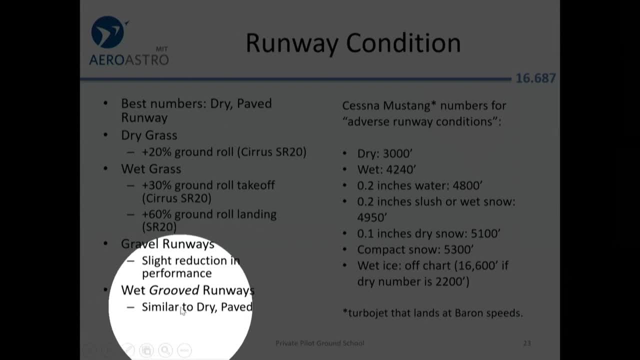 more room to take off At the airline. If the runway was grooved- which almost all bigger US airports have, these grooved runways- we didn't make any adjustments, Didn't matter how heavy the rain was, It didn't matter how long it had been raining. 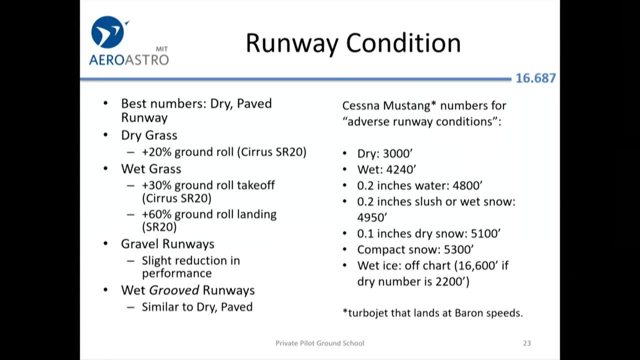 We just assumed it was going to perform exactly the same as if it were dry. If it's not a grooved runway, though, and water can sit on the runway, it can have a big effect on performance, So here are some numbers that I pulled. 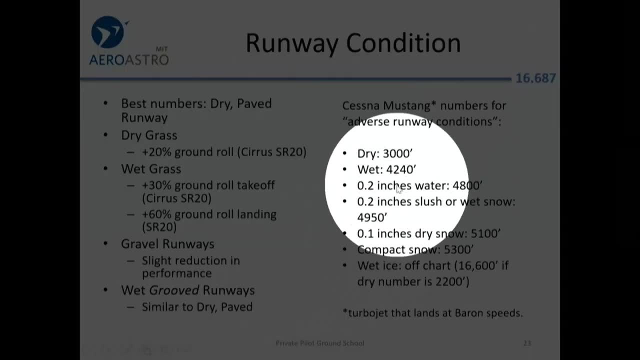 I'm type rated in the Cessna Mustang, which is an interesting little business jet. It lands at about the same speed. It's a Beechcraft Baron, So it's a great beginner jet Anyway. so in conditions where you need 3,000 feet of runway, 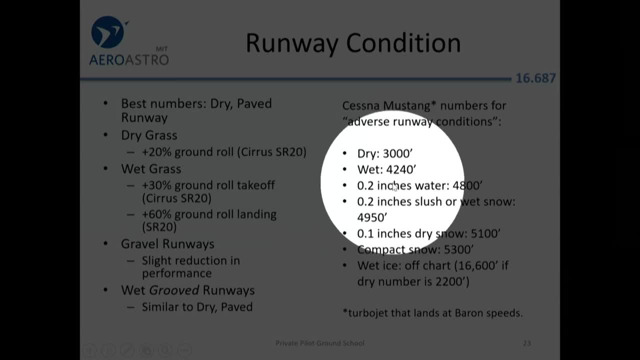 that's up at pretty high altitude. You're going to need 4240,. Cessna says if it's wet, If water is actually standing on it. I think 0.1 inches of water was even more. You'll need yet more runway. 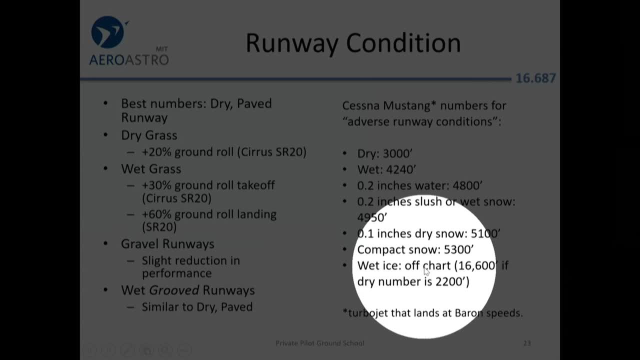 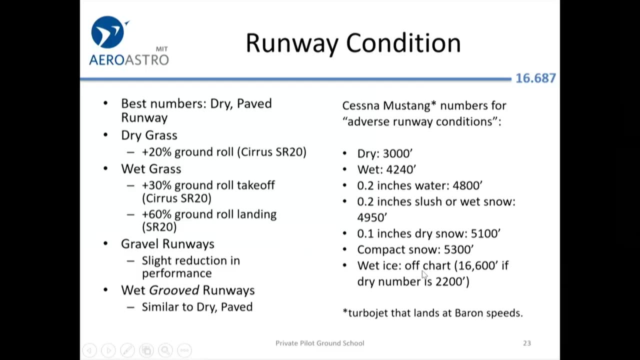 If it's snow a little bit more Wet ice. it was just off the chart, But if you started at 2,200 feet of dry runway you would need 16,600 feet. So actually oftentimes when the surface is contaminated, 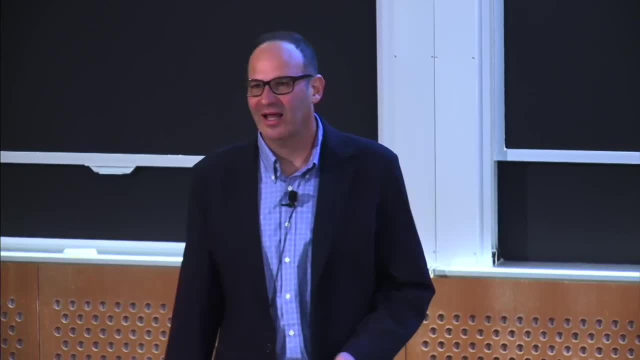 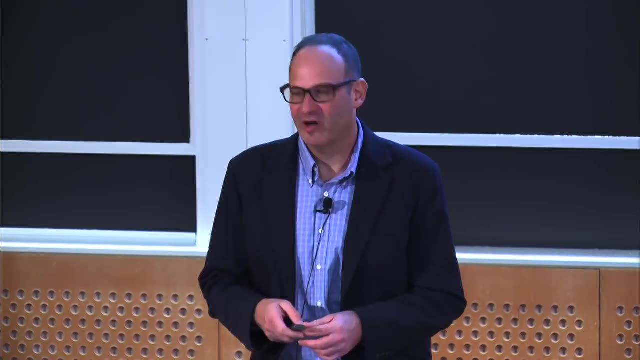 that's one reason why even fairly small business jets may need a long runway, like at Logan or at Hanscom Field. Even an airport like Nashua, which has 6,000 feet, may not be enough if they're reporting that there's snow on the runway. 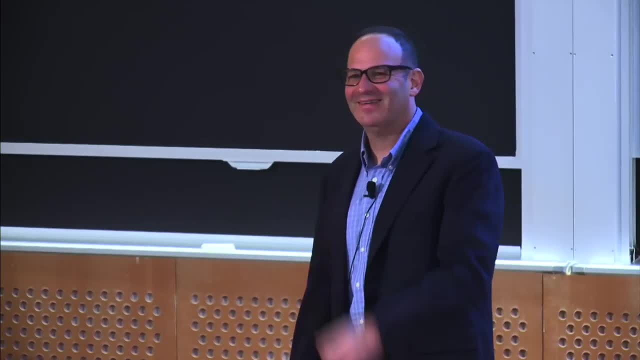 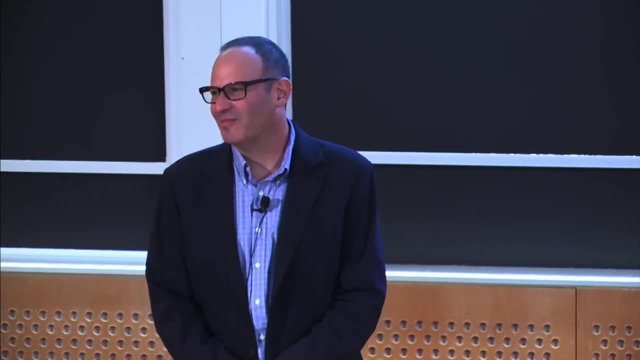 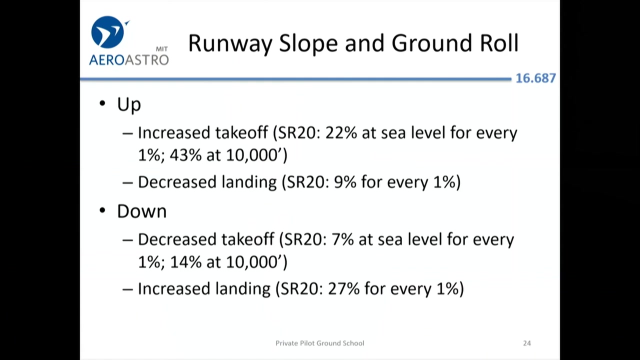 OK, what about slope? So going downhill is obviously a lot easier than going uphill And you can see here- and also stopping going uphill is a lot easier. So here are some numbers from the Cirrus book- that every one degree of slope increases your takeoff run. 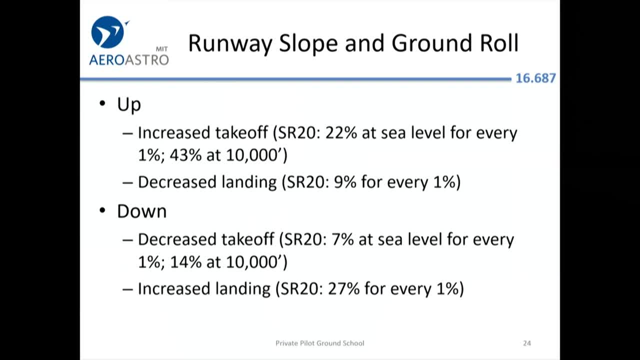 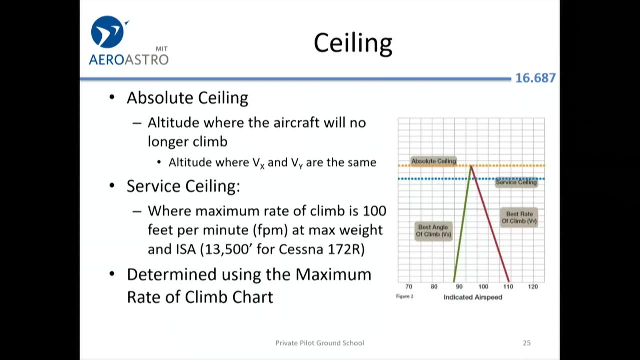 by 22% at sea level, for example, And you also get a 9% reduction in the landing distance. OK ceiling- The service ceiling of the aircraft- is a little bit below Absolute ceiling. That's where the FAA says the plane will. 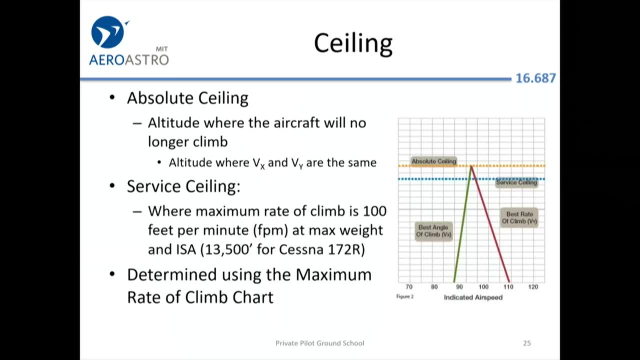 climb 100 feet per minute, or the manufacturer has demonstrated to the FAA that the airplane could, at least when it was brand new, make 100 feet per minute in climb rate. So that's at 13,500 feet for a 172 Cessna. 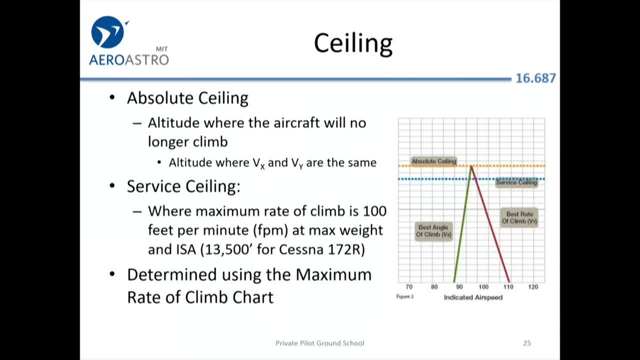 And I think that's pretty typical for these normally aspirated four-seaters. Somewhere around there is where it'll stop climbing The Cirrus. there's a limitation in there that says maximum operating altitude. The altitude is 17,500 feet. I think that's more regulatory, because you can't take the Cirrus up into the flight levels. It would need extra equipment to go up above 18,000 feet maybe. I don't think it's really practical to get up to 17,500 feet at maximum gross weight. 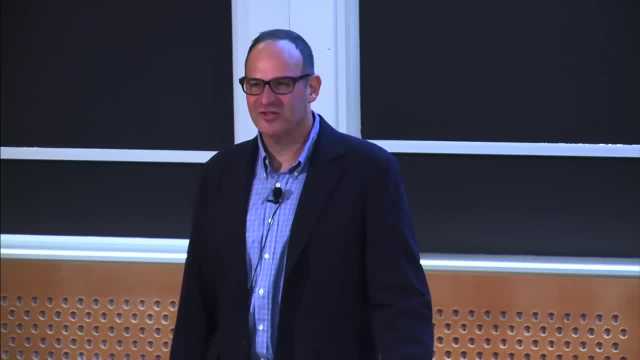 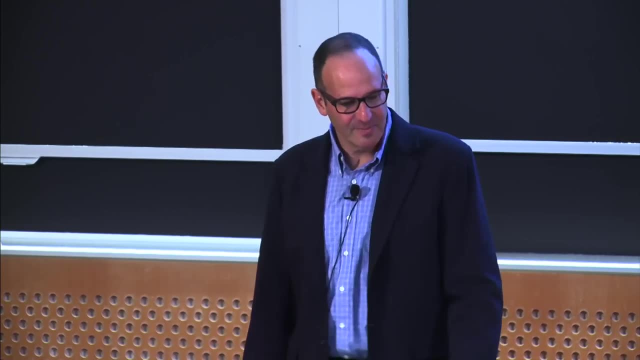 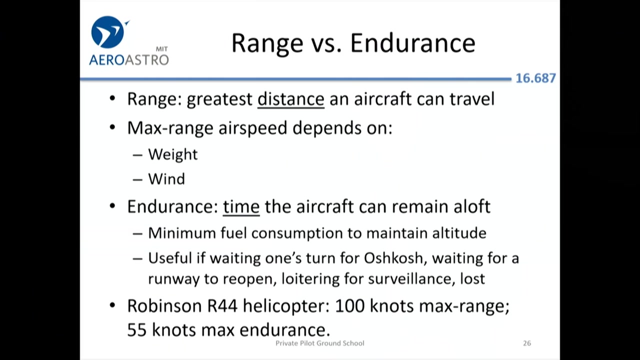 in a standard atmosphere. I've gotten it to about 13,000 feet out west in the summer, so that is more like being at 15,000 feet, But it was barely climbing. OK Range versus endurance. So we're going to get back into the power and drag curves here. 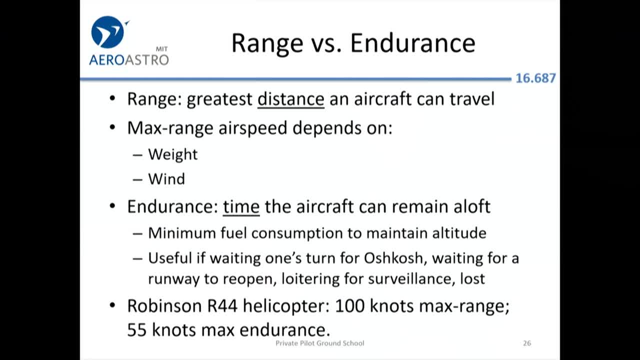 The max range airspeed is going to depend on the wind. like I said earlier, If you have 100-knot headwind, then you have to go faster than 100 knots in order to go anywhere, If you want to loiter for some reason. 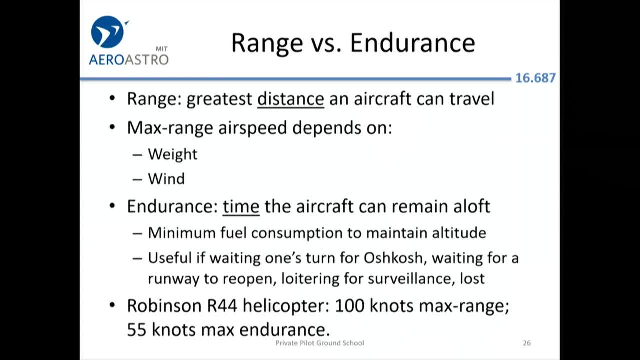 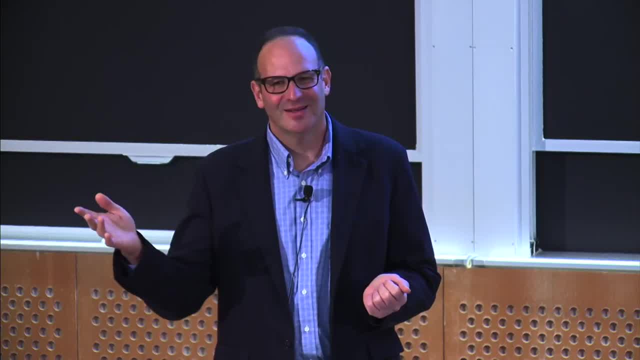 this year at Oshkosh was a nightmare for people who didn't go IFR. They had a lot of marginal IFR weather so for the first couple of days when people were arriving there were these short windows of just an hour or two. 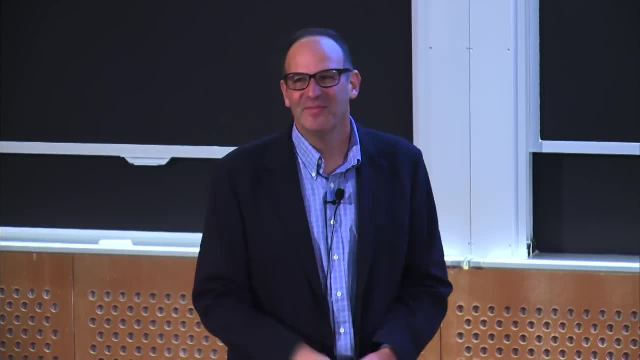 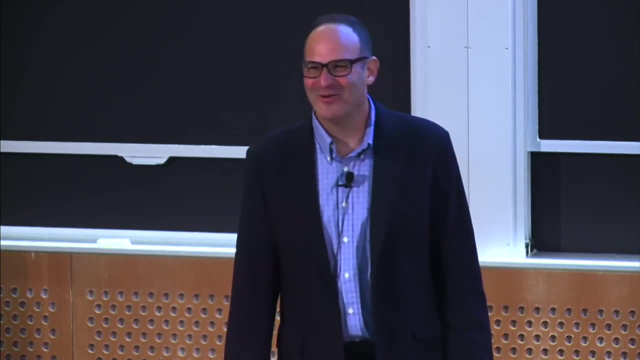 when people could really get in legally- the VFR home builder types- So they were just holding. People were literally holding for three hours and then finally had to give up and go and refuel somewhere. But if you're in that situation, you want to set your speed to whatever the minimum fuel consumption speed is, And it can be quite different. The Robinson R44 manual talks about 100 knots for max range. I believe that's assuming a 10-knot headwind, Since usually we're suffering with a headwind more often. 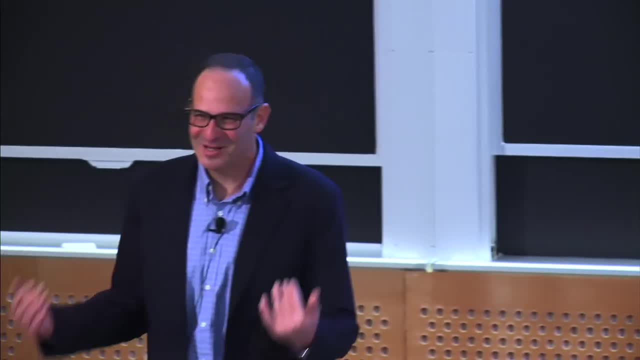 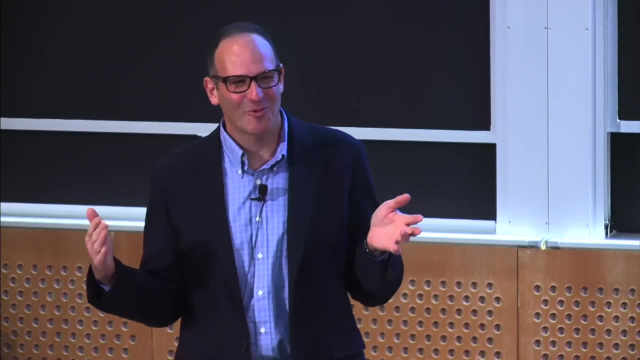 than with a tailwind. And you might say: how is that possible? How is it possible to have a headwind unless God hates you? How is it possible to have a headwind more than half the time? If you think about it, Richard, do you know the answer? I do. What is it So? here's the question. You're going to fly 100 knots to an airport In zero wind. how long does it take to fly? You have an airplane that flies 100 miles an hour. How long does it take to fly a round trip? Trick question: 100 miles apart, 100 mile an hour, airplane, No wind, How long does a round trip take? OK, Let's say you have a 50-knot headwind. It's exactly on your nose. You're going to get 50 knots headwind on the way out. 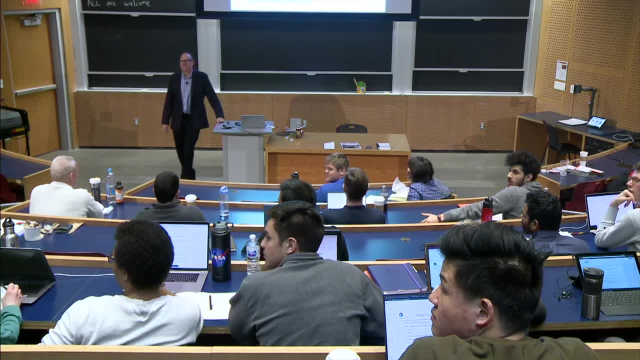 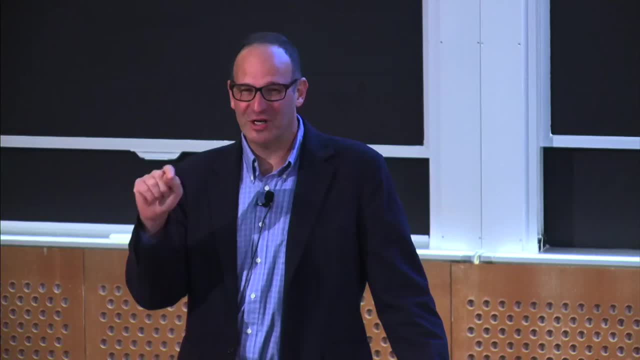 and a 50-knot tailwind on the way back. How long does it take? Two hours Wrong, Work it out. Well, that's one aspect. You're going to spend more of your time. as Richard's saying, It's going to take you two hours to get there in one direction. And then it won't take you zero time to get back. So you're spending more of your time in the headwind than in the tailwind. But there's something even worse. I saw this the other day in the Cirrus. There was about a 70-knot wind. that was actually. 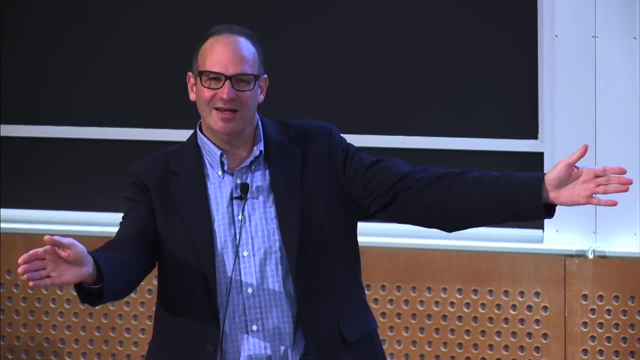 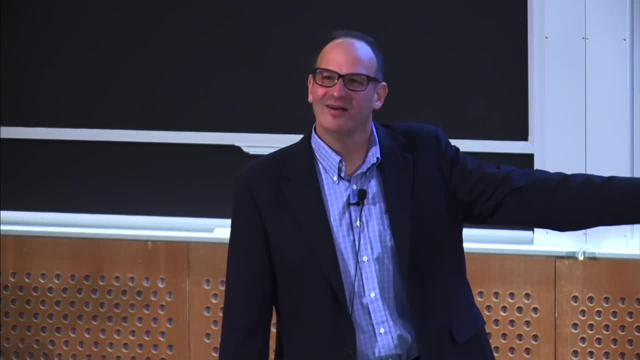 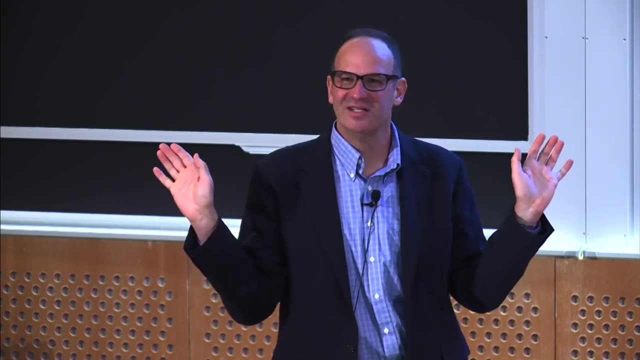 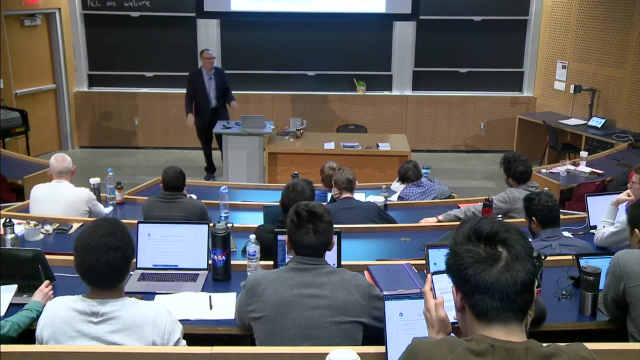 So even a wind that is directly a beam wind, 90 degrees off, there's actually the majority of the 360-degree circle of wind directions. the majority of that is subtracting from your performance and has at least some headwind component. Sound crazy. 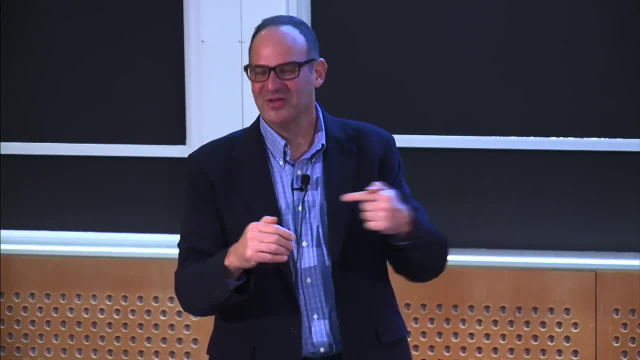 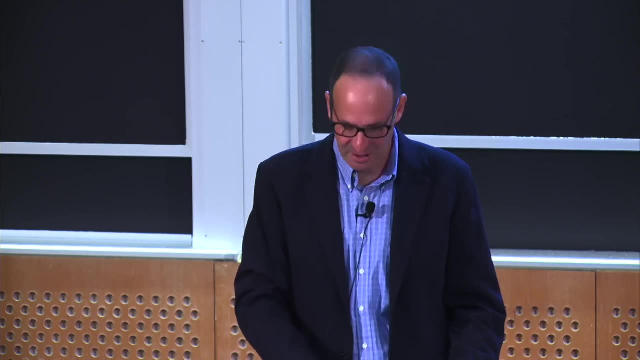 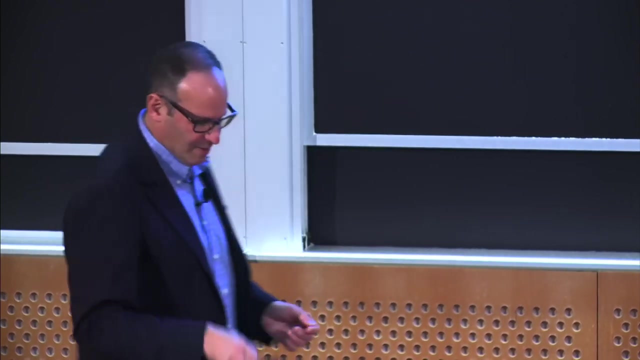 Think about it. yeah, So if you're going 100 miles and there's also this 100-knot sidewind, you're having to spend quite a bit of your energy continuing to steer into that sidewind. OK, here is a power and drag curve for an RV6A. 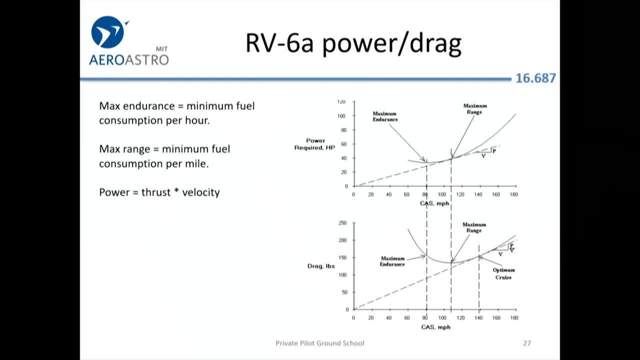 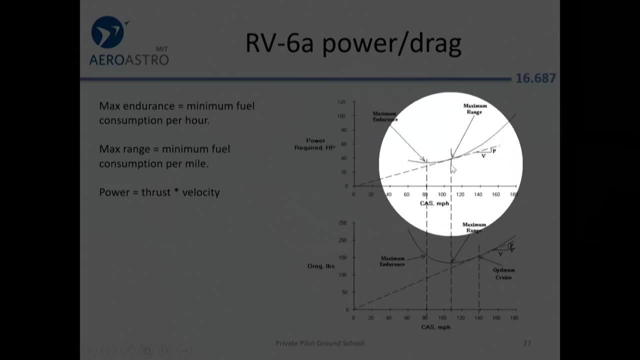 The experimental guys are, in this case, more aggressive about producing charts. So if you actually care about where you're going, you want to be a little bit up the power-required curve. You want to find out where it's tangent to one of these lines. 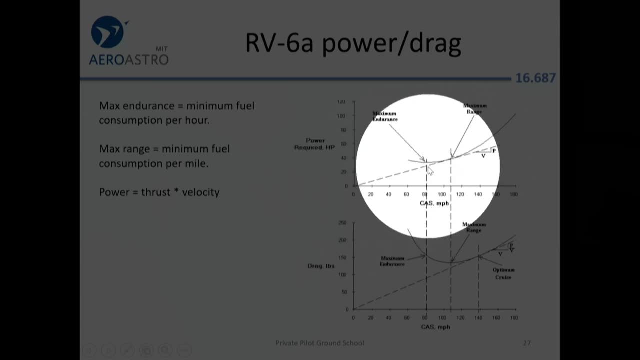 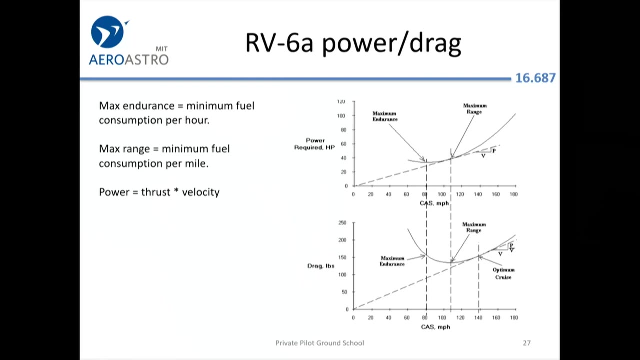 going back to zero, And if all you care about is maximum endurance, you just want to be at the point where the curve is at its bare minimum, because then you're consuming the least power and, in theory, burning the least amount of fuel. 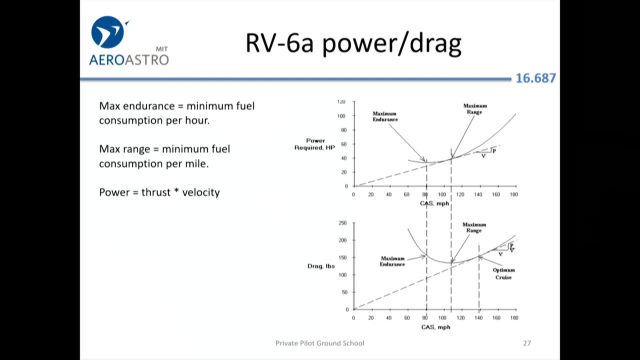 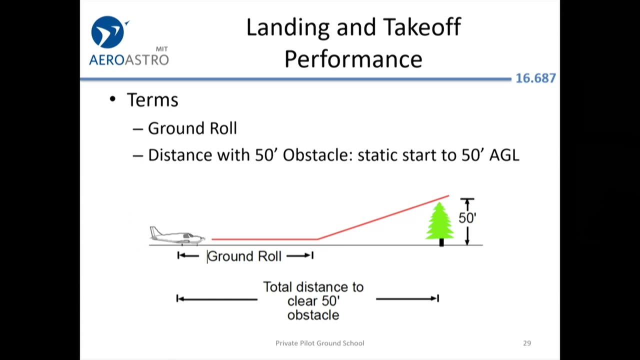 Does that make sense? All right, the terms ground roll these performance charts in the book that you get with the airplane. they will assume a static start. So that means you're holding the brakes, you slam the power forward, you let off the brakes. 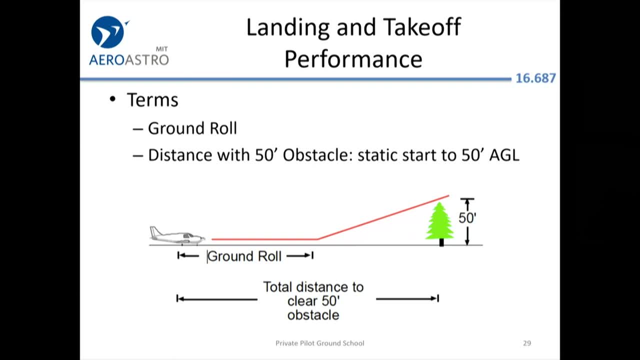 and you're going to get the book numbers because there's no acceleration time for the engine. And actually that's how jets are supposed to take off too, But you probably remember from your commercial flights that's not really how it happens. 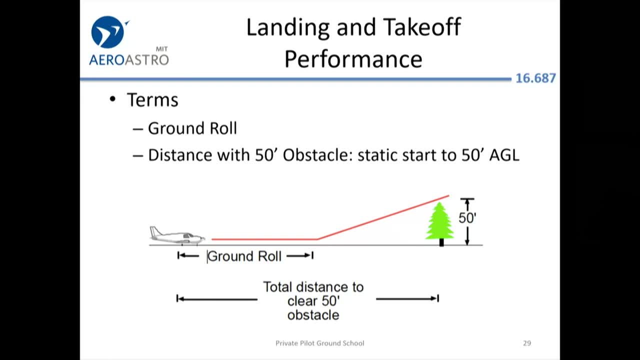 The pilots don't hold the brakes spend. it takes maybe 10 seconds for a really heavy jet engine to spool up to full power. They don't just sit there holding the brakes on the engines at the max and everything screaming and the airplane shaking. 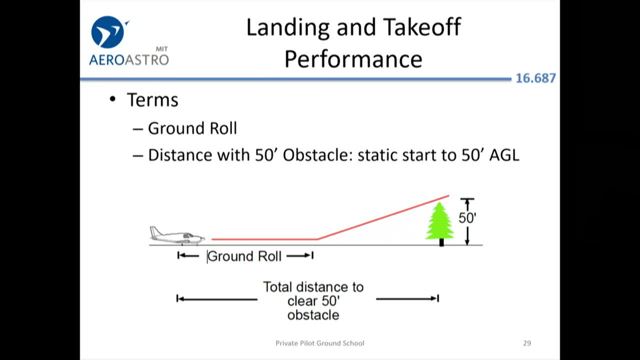 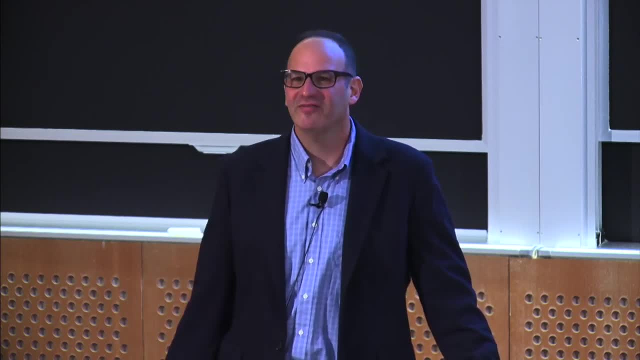 because it's just uncomfortable. So they usually cheat. Technically they're not really supposed to do it because at that point you're test pilots, You don't really have any data for a rolling takeoff. But again it would be kind of unnerving. 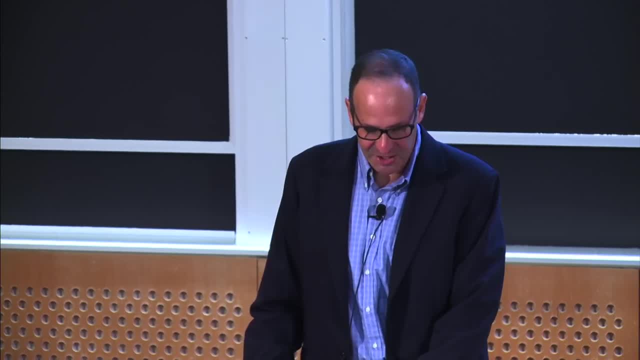 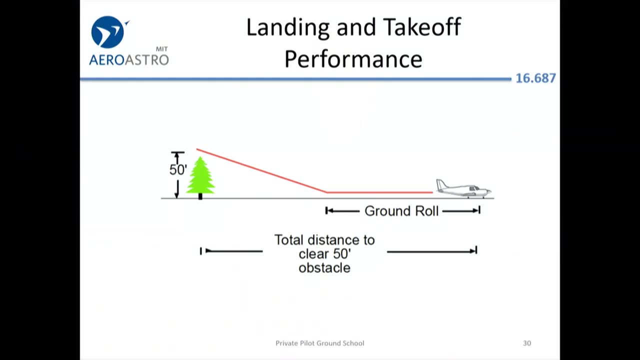 It would be unnerving for passengers, I think, if they were sitting there with the airplane straining against the brakes. OK, same deal here: Ground roll and the total distance to clear the 50-foot obstacle. This is what I was telling you about the other day. 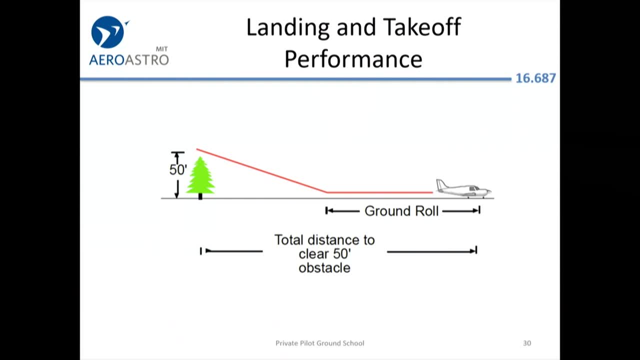 with the Cirrus hero who wanted to go to, I think about 2,500 feet of runway. Actually, we had to subtract some. I think it was 2,700 minus 400.. He had about 2,300 feet of runway. 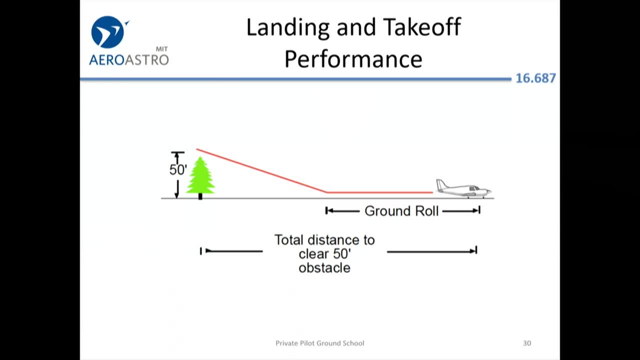 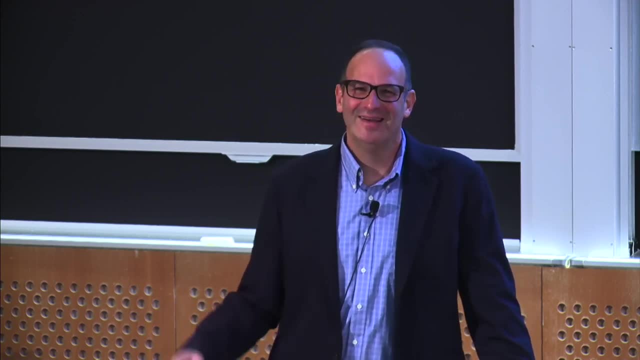 and he wanted to go there in the Cirrus, which takes 2,100 feet. Another guy actually wanted to go to. there's a private air park in Falmouth, Massachusetts, where you can have a house right next to the runway. 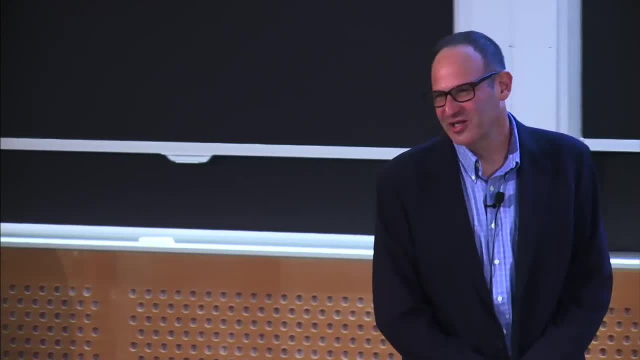 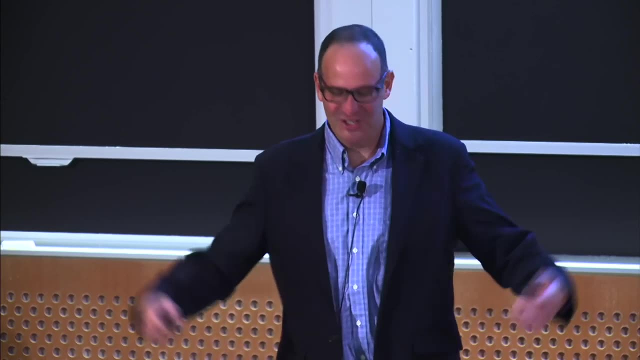 and keep the airplane in your garage, And that airport's only 2,300 feet long. And another East Coast Aero Club guy. I was handing the airplane over to him and he had this huge friend with him. This guy was like a NFL linebacker. 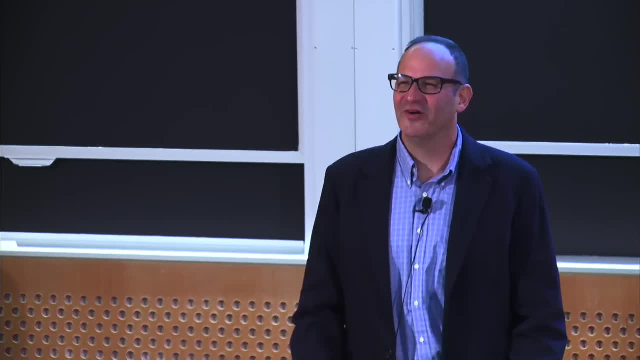 So it was just the two of them, but big, And he wanted also it full topped off on fuel, So they were going to be right at gross weight. I said where are you going? He said Falmouth. I said 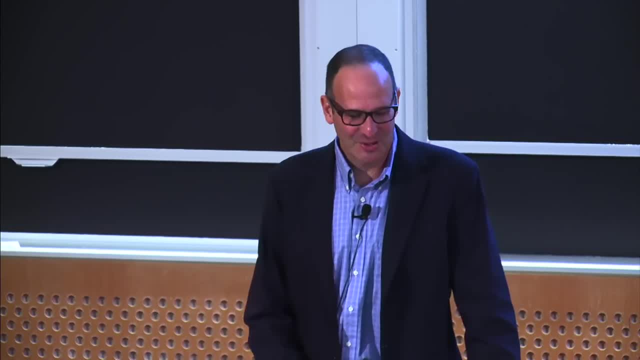 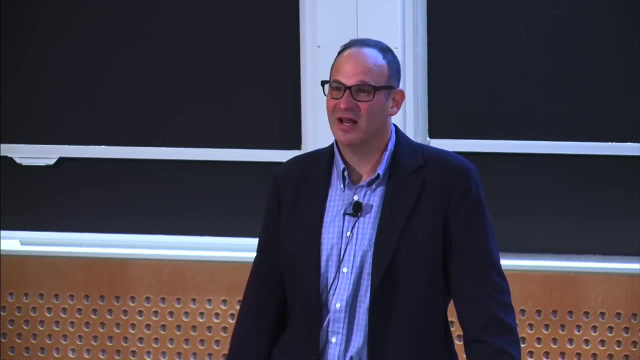 And he'd just gotten his private pilot certificate a few months earlier. This guy was not commercial IFR rated like the other And I said, look, if you do everything perfect, you're going to use up 92% of that runway. 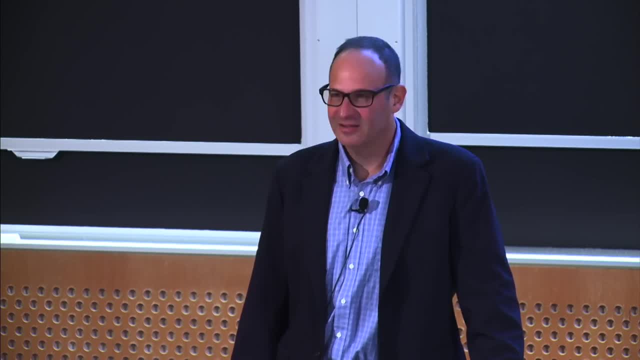 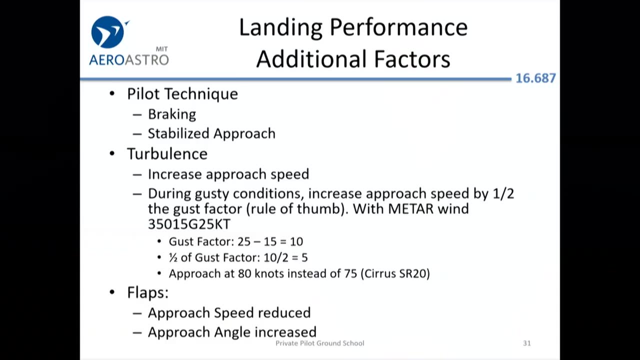 because it's hemmed in by these obstacles, So don't do it. So he did end up going to Hyannis. I think All right landing technique can actually affect the performance. So they talked about it. They talk about, like an average pilot, the book numbers. 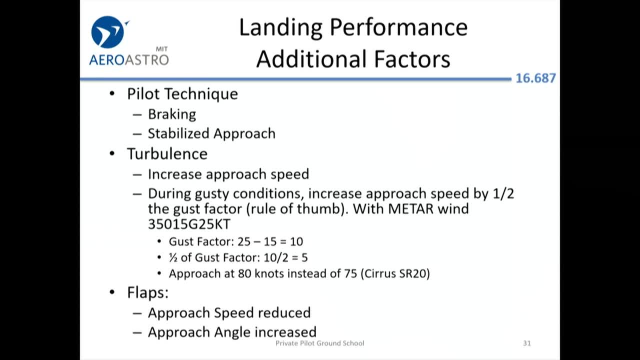 they're predicated on extremely aggressive braking like right to the point where you would flat spot the tires. So don't count on getting those book numbers unless you're willing to be more aggressive than probably you would want to be. And actually I'll tell you a story about my airline days. 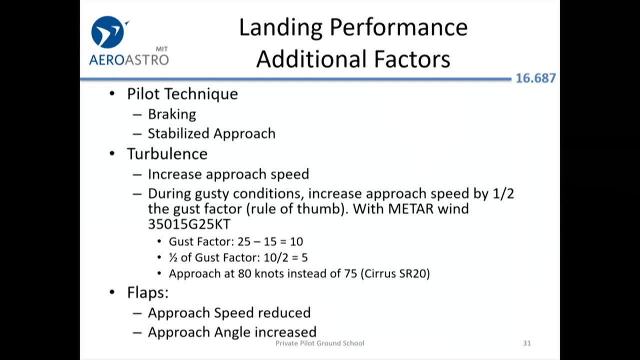 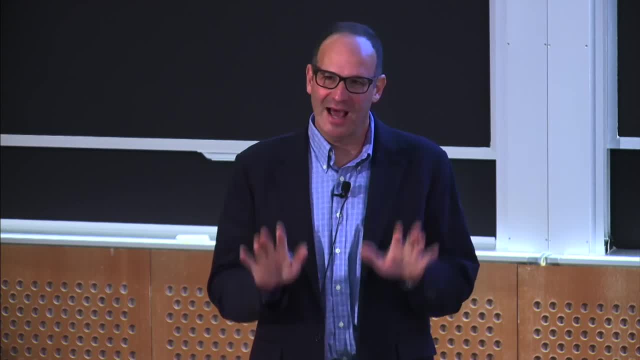 I did a visual approach in the LaGuardia And with jets it's not conventional to try to do the really greaser landings that you would do in a little airplane Because you need to get the airplane down and the spoilers to pop up. The jets are very efficient gliders. They don't have a big prop in front And when you pull the power back on a piston aircraft it really slows down dramatically because the prop has a lot of air resistance. None of that's going for you with the jet, which is more 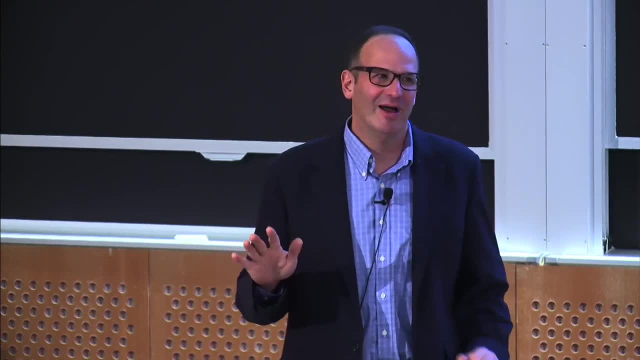 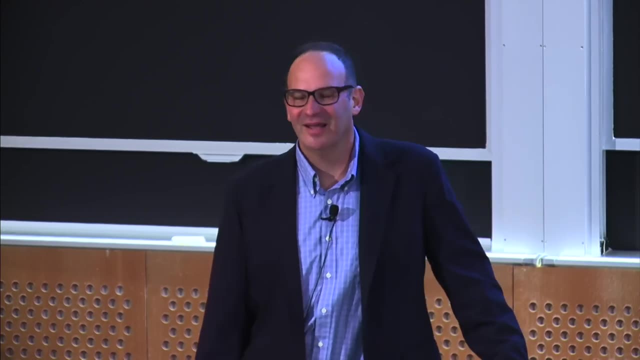 efficient to begin with. So basically the task of an airline pilot is really to slam it on And that way the spoilers pop up And then the brakes start really working effectively And you turn off the runway in LaGuardia before you go into the room. 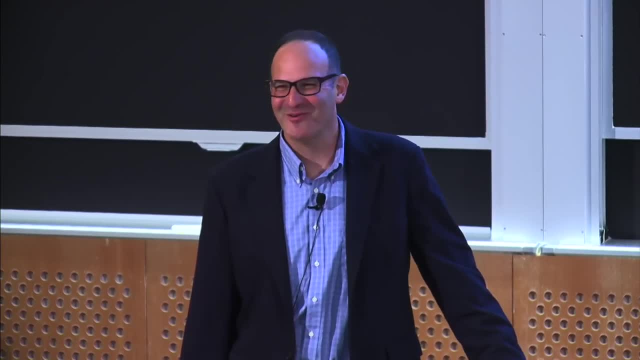 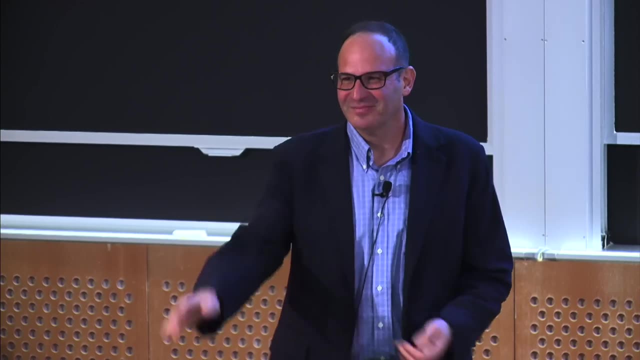 And that's where you land, on the river. So I landed like a Cirrus because it was my first month on the job And I chewed up probably 1,500 feet of runway before the airplane touched down And I applied fairly gentle braking and thrust reverse. 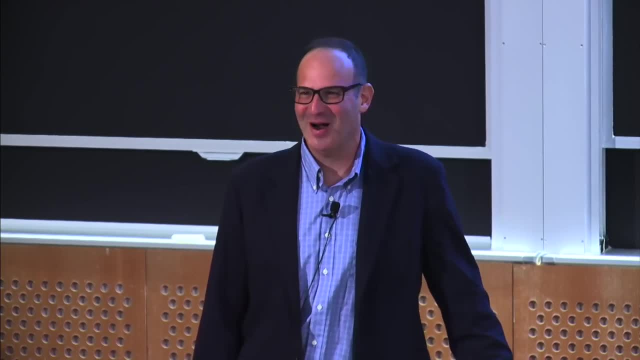 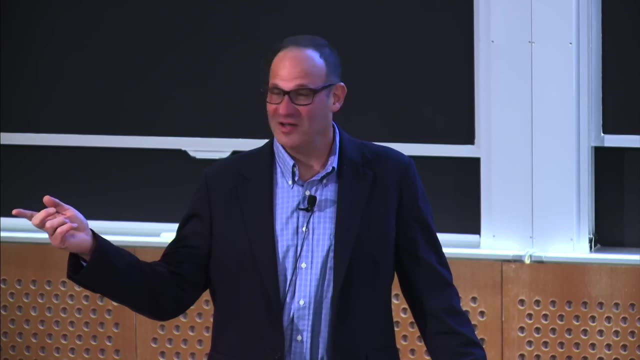 and turned off after about 5,000 feet of runway And the captain's like that sucked. I'm going to show you how it's done. on the next leg We did LaGuardia to Charlotte, North Carolina. Who else did that leg? 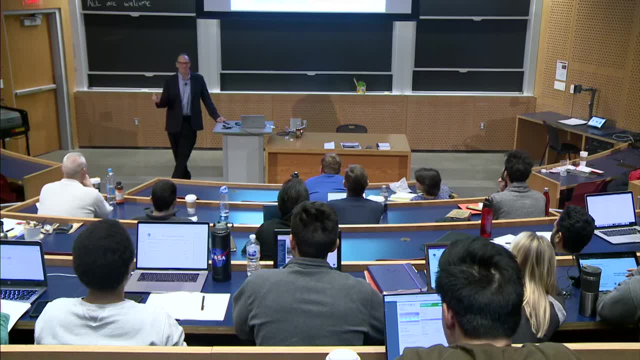 Sully Sully Captain. Sully, Sully, Sully. So he dumped his passengers into a filthy, cold river And they called him a hero. I got my passengers to Charlotte warm and dry, And where was my medal? 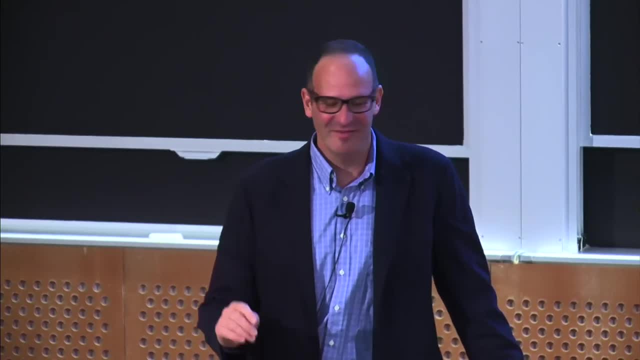 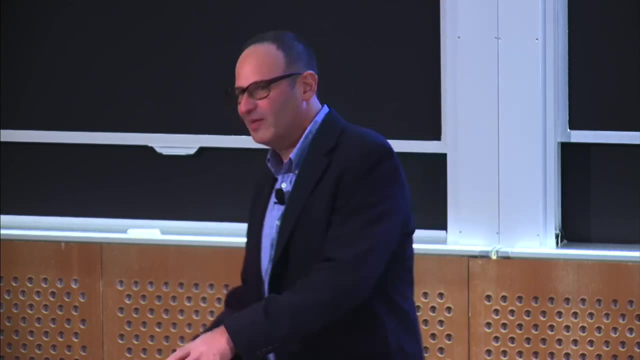 Where was my fame? Nowhere, All right. So life is unfair. You've learned that, Anyway. so the captain takes this one Air traffic control lines us up, Instead of the visual approach where you're doing everything by eye and following another aircraft. 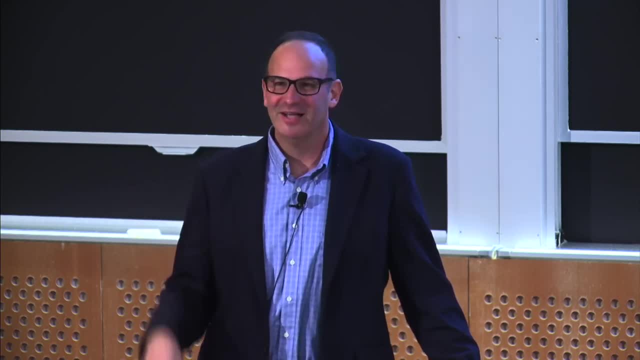 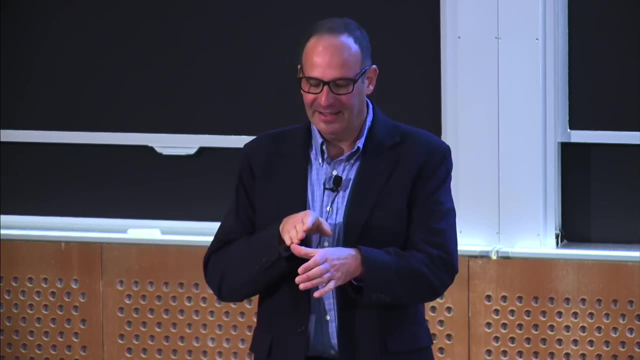 and you can't use any of the fancy automation. we were lined up 10 or 15 miles out for straight in approach to this angle. This is the old runway at Charlotte And all the captain had to do was on autopilot. All he had to do was tweak the thrust levers. 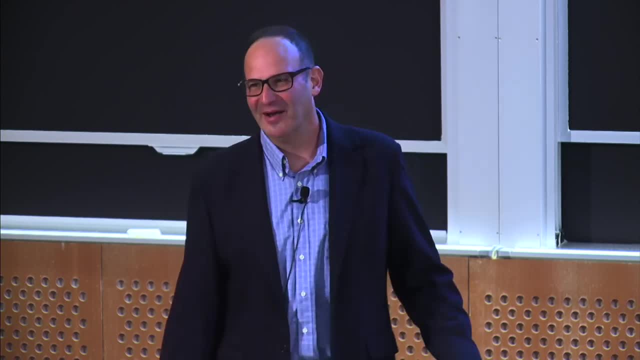 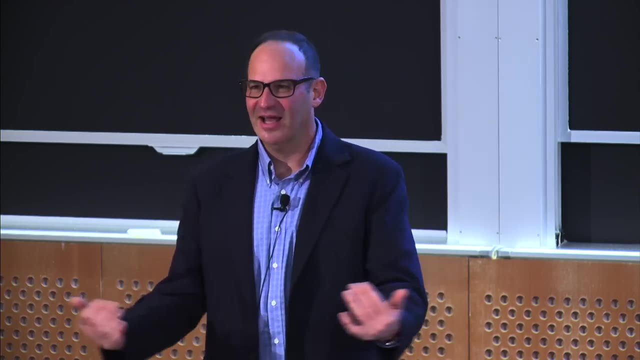 for the perfect airspeed. The autopilot's flying. He disconnects the autopilot a couple hundred feet above the ground. Now he's hand flying, All he has to do. the CRJ doesn't have the 50-seater, doesn't have any leading edge devices. 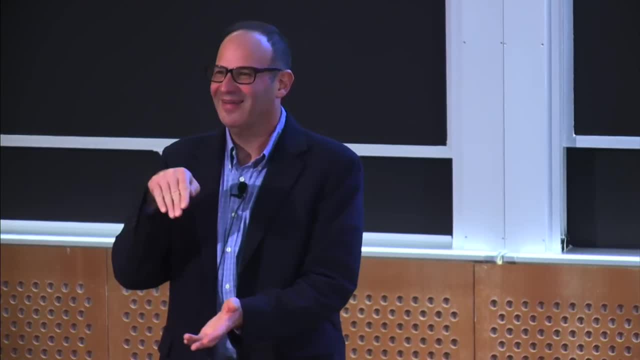 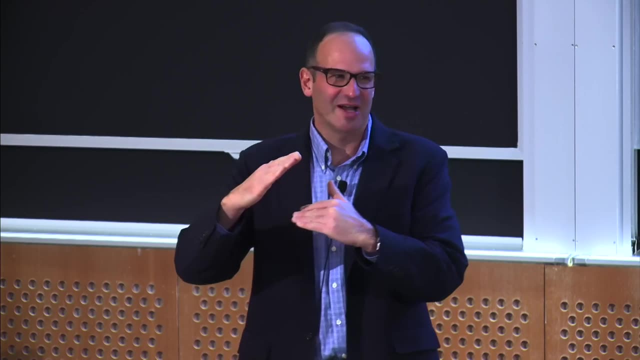 So it has to be pointed down a bit like a lawn dart. It's not that different from landing a Cirrus, But it's unconventional for an airliner. The airliners, you notice they usually because of the leading edge devices. 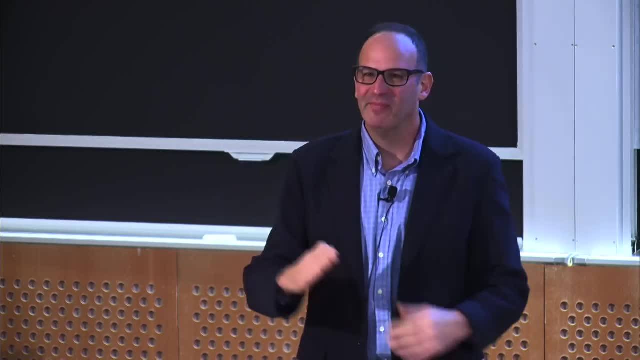 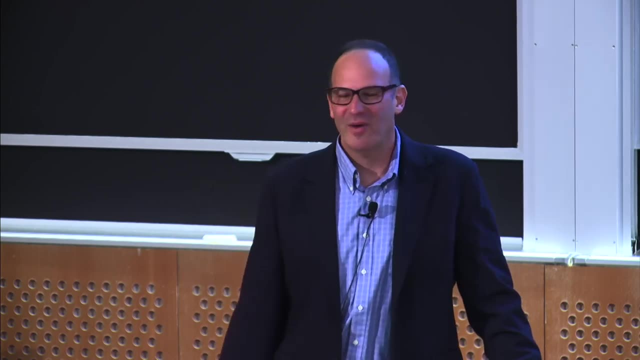 even when they're going 120 knots or so they can be kind of nose up And they still fly pretty well. So the airplane almost can be flown and it can auto land in some cases onto the runway by itself, with just a slight additional flare. at the end. The CRJ has to be kept nose down 145 knots faster than all but the very biggest jets, And then it has to be flared from minus 5 to maybe plus 5 or plus 7 at the end. 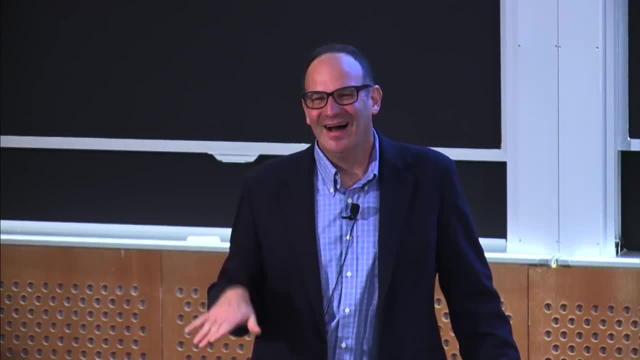 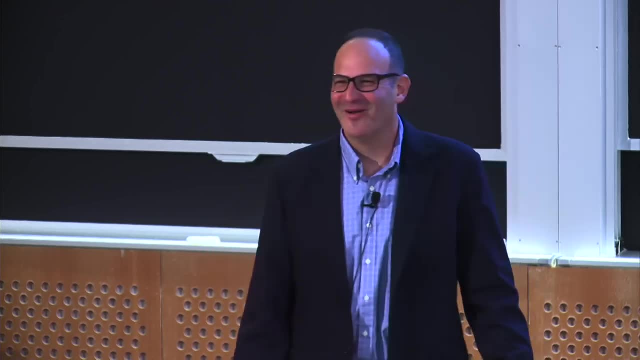 So the captain, after telling me what a bad job I had done, he flared about 5 feet too high And the airplane just sailed over 4,500 feet of runway, I think, before it finally touched down, And he slammed on the brakes: maximum thrust, reverse. 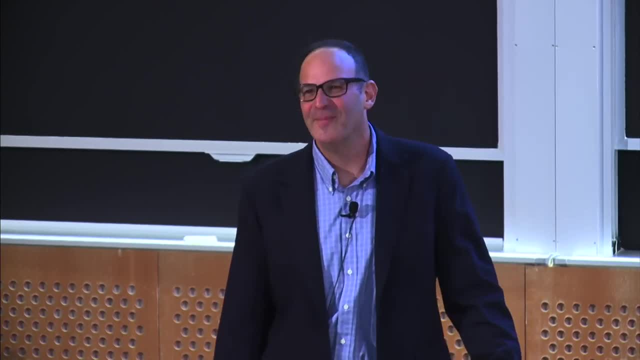 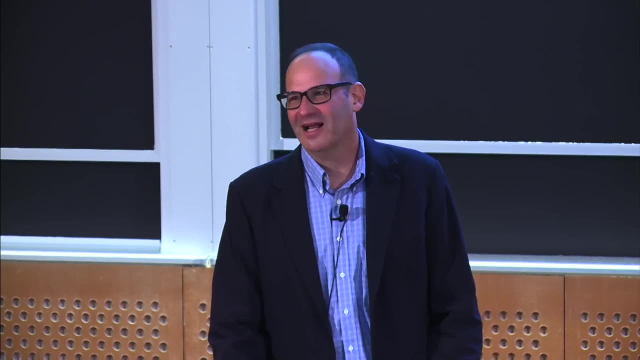 We barely made it off. I think we made it off after 7,200 feet of runway, So it would have been, I think, in the water in LaGuardia. So that's the kind of thing where you can't. that's why these safety margins are. 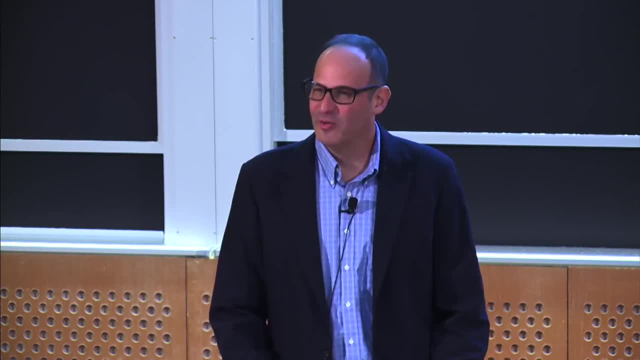 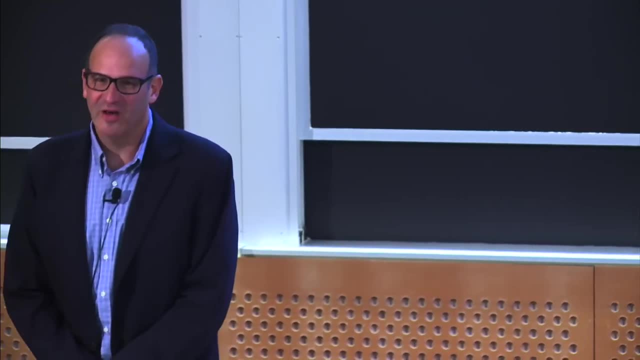 good to build into your own flying Because You know the book number said the airplane would land a lot shorter than that. Also, in a jet there's really not a good go around technique. Once you're below 50 feet you're. 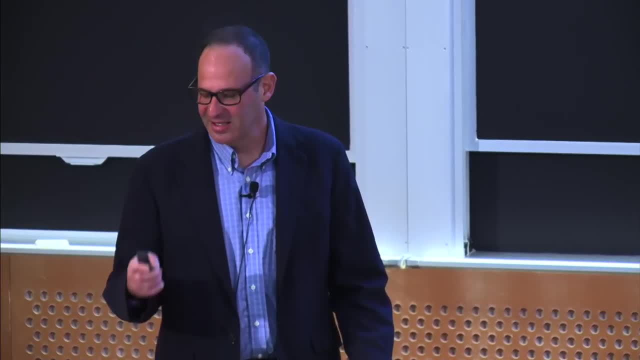 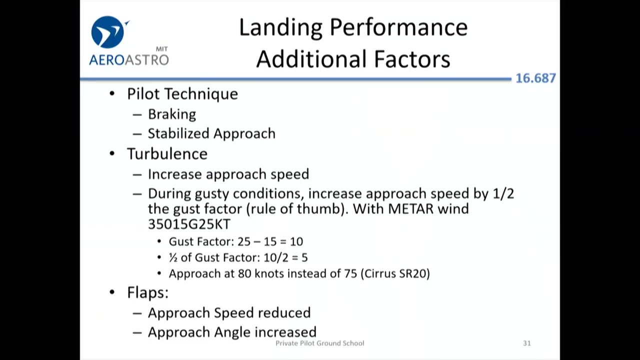 not supposed to try to add power and go around because it takes a while to spool the engines up. All right, In turbulence you usually will increase your approach speed, which means you're going to chew up more runway. You're supposed to add half the gust factor as a rule of thumb. 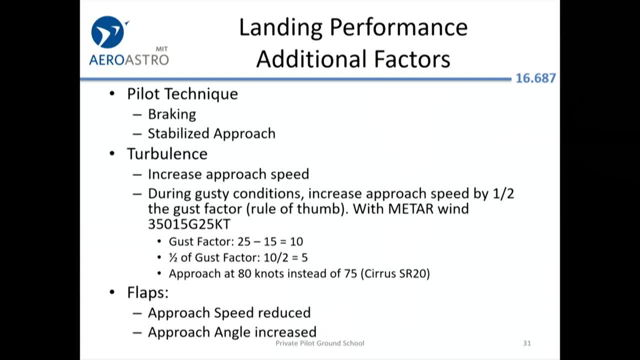 So if the wind is 15, gusting 25, you're going to speed up your approach by 5 knots. And I got the numbers here for the Cirrus: 75 is kind of a good overall number, And then you'll beef it up to 80.. 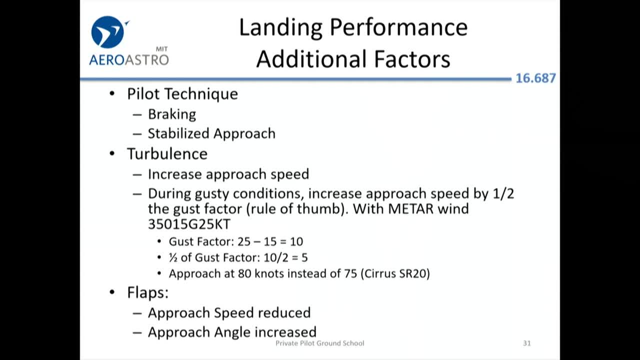 But that means, unless it really is a headwind, when you're landing you're going to chew up a little more runway than expected. OK, Flaps, as Tina mentioned, they enable you to keep your approach speed low while having a nice steep approach angle. 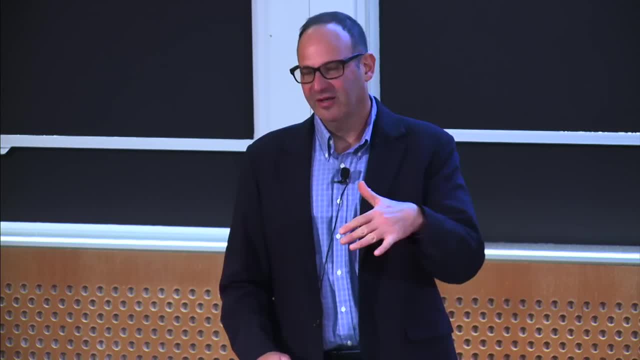 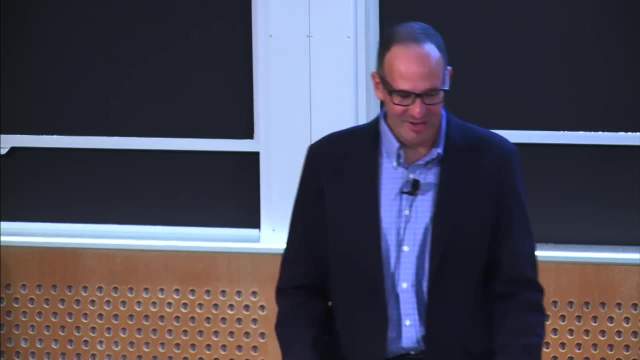 So that's good for getting over trees and stuff. If you're in an aerobatic airplane or something else that doesn't have flaps, you can actually slip and kind of go sideways down towards the runway and get over the obstacles, But it's a lot easier just to put the flaps down. 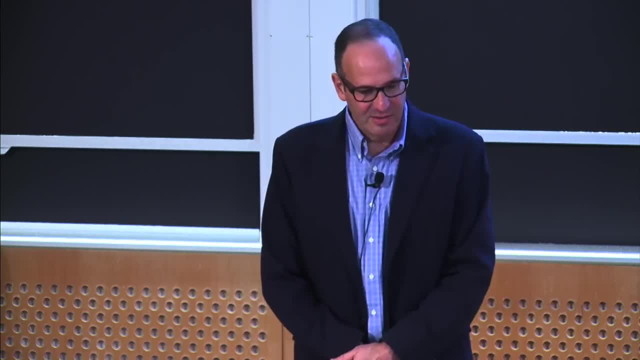 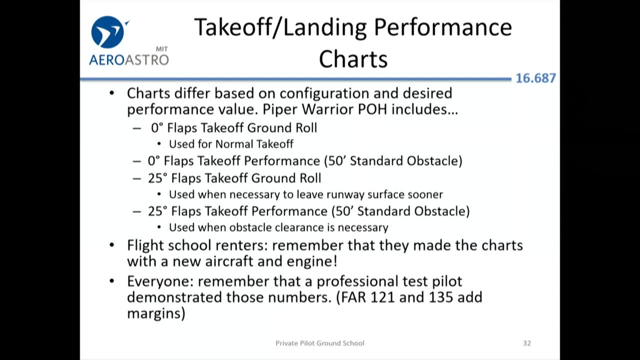 OK, The charts come in all kinds of variations. in the POH, especially for the bigger airplanes, You'll have 10 charts that look identical, except for a couple of numbers, like the exact flap position, whether the anti-icing is on or off. 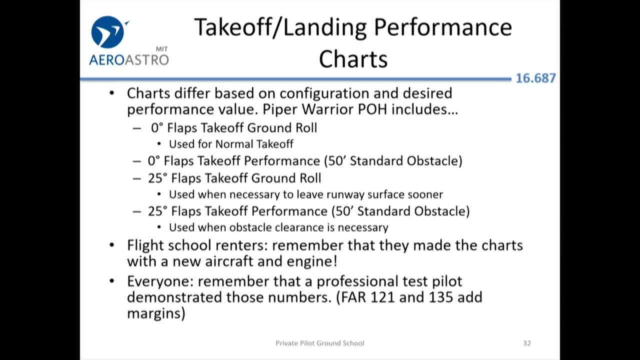 The Piper Warrior POH is a lot simpler, And that's some of the charts we're going to cover, in addition to some of the anonymous airplane charts that the FAA gives you with the test. So one thing to remember if you're a renter. 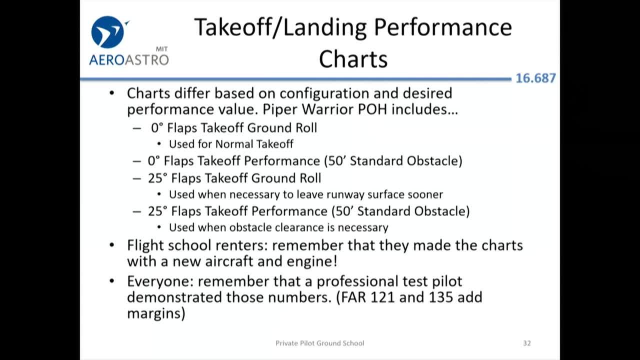 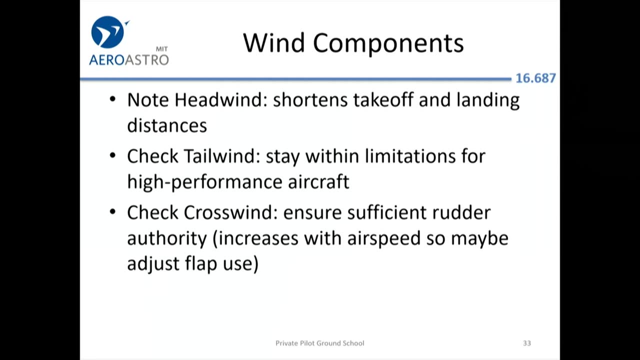 in addition to the fact that you want to build in maybe some charter and airline minimums into your flying, is that all those numbers were with the brand new airplane that was perfectly straight and had a perfect engine. OK, So wind components, You're going to get shorter takeoff and landing distances. 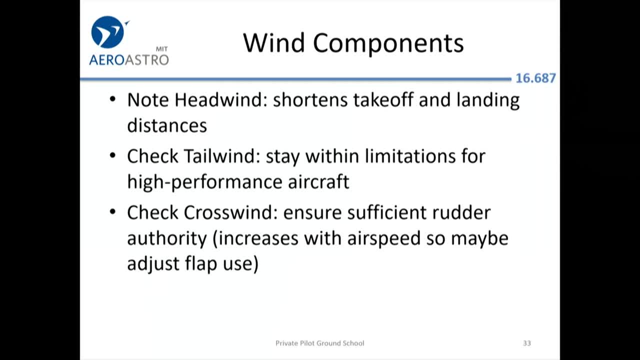 with a headwind, A tailwind. actually, it may not be legal to operate a high-performance aircraft on a runway with a tailwind of more than a certain amount. I think for the CRJ it was 10 knots. We just simply could not land with a 10-knot tailwind. 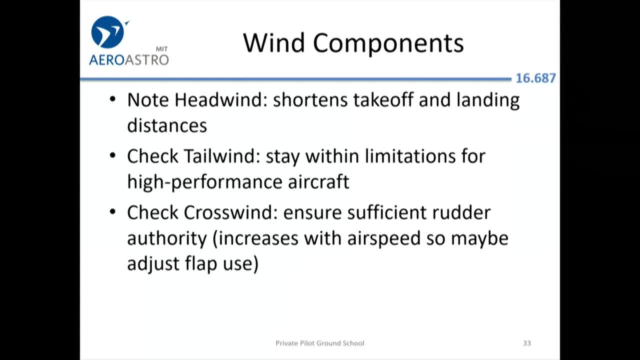 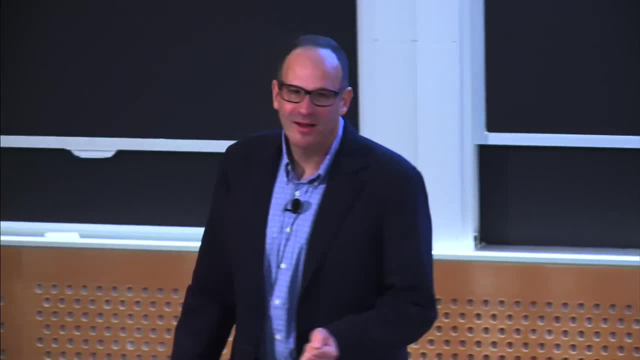 or more than a 10-knot tailwind. Crosswind is a little bit different. You'll get a max demonstrated crosswind Crosswind component in the manual, So it'll tell you. a test pilot managed to hold this airplane straight on the runway with full flaps. 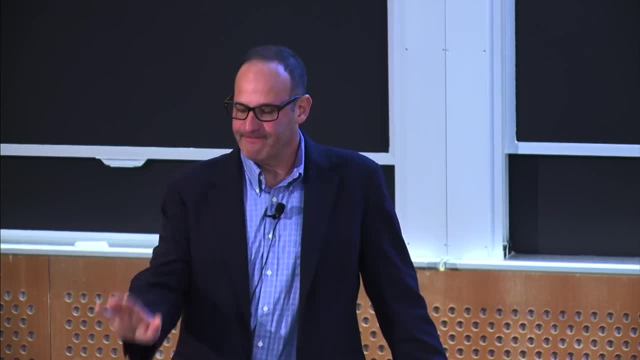 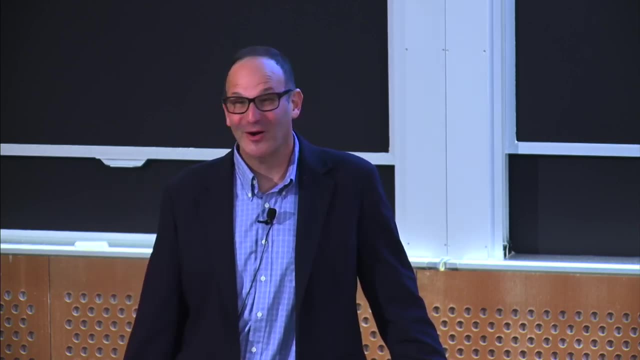 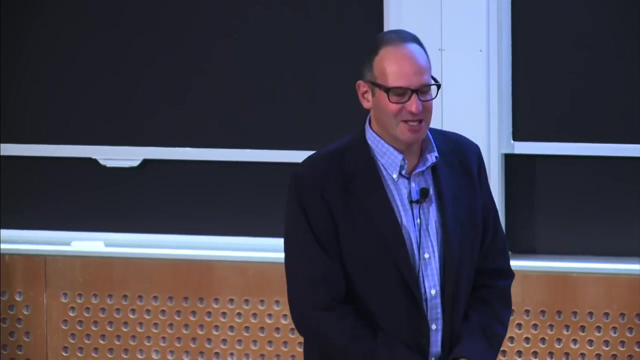 or whatever the normal landing configuration is. and there was enough rudder to land with a 15-knot crosswind, So that's max demonstrated. It's not a limitation, So you may, if it is, it'll say this is a limitation. 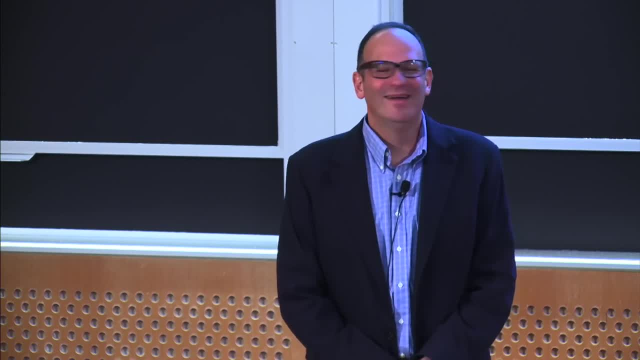 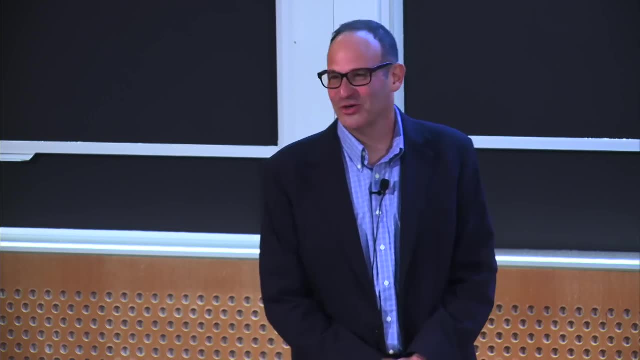 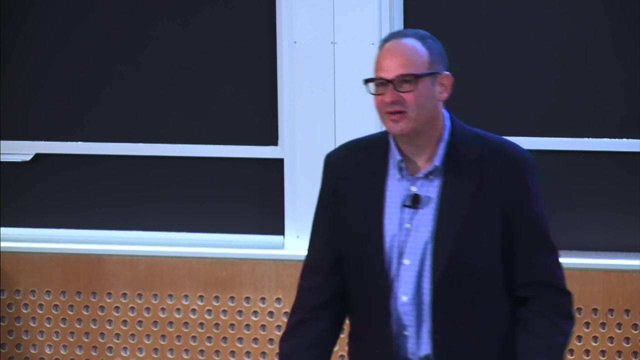 But max demonstrated just means a test pilot did it. It'll probably work for you too If you manipulate the controls in the same way, And beyond that you can't be sure. So one thing that people will do is they will adjust the flap amount to have a reduced use of flaps. 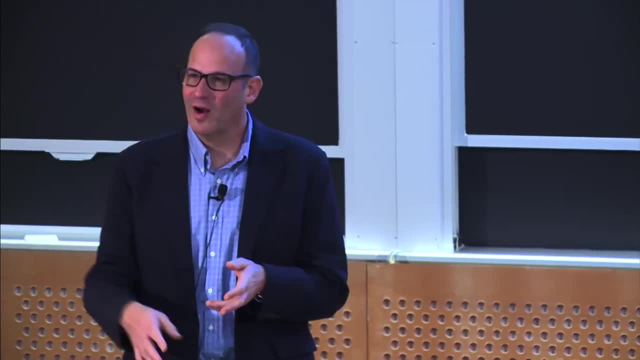 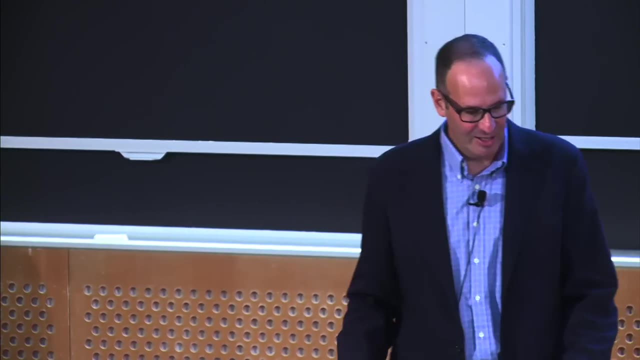 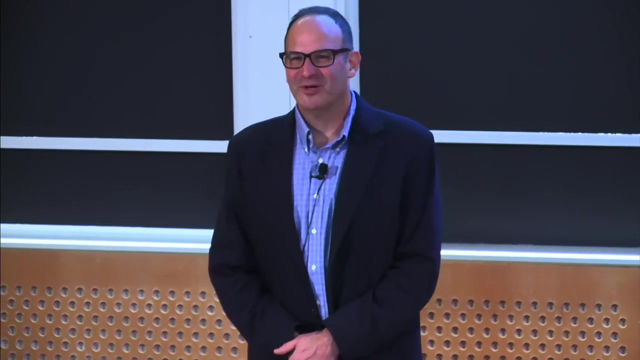 in a heavy crosswind That keeps the airspeed up, You will chew up more runway, But when the wheels actually touch the ground, the wheels provide a little bit of stabilization and help keep you from getting blown away. You're going to see tomorrow Dojo from the Brazilian Air Force. 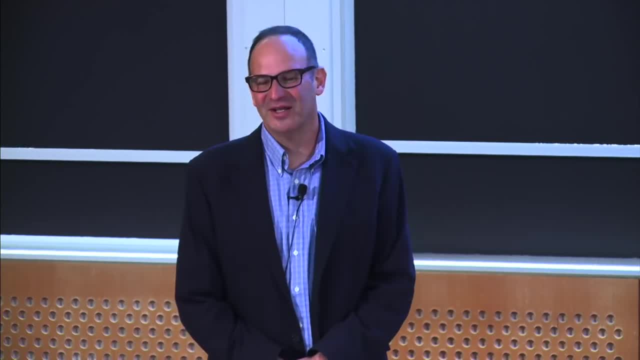 is going to tell you about testing the various airplanes, but especially the Super Tucano, in very heavy crosswinds. Down there in South America they have some pretty heavy winds. I think they went to Chile to do that. I could be wrong. 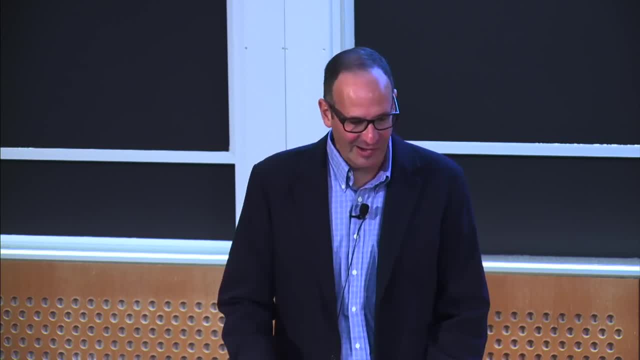 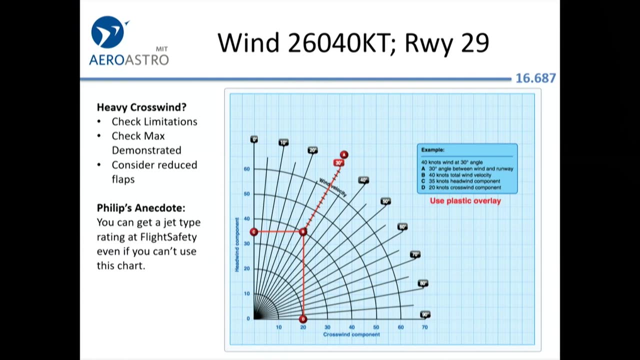 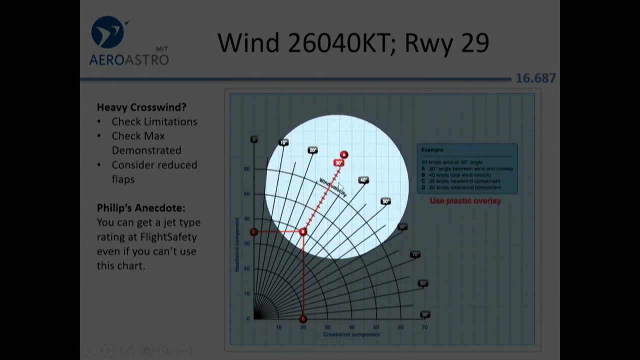 Or maybe it was just right next to the Andes in Brazil, OK, crosswind chart. So this here, This here shows you that if you have a 40 knot wind at a 30 degree angle, you go over here on the chart to the 30 degree line. 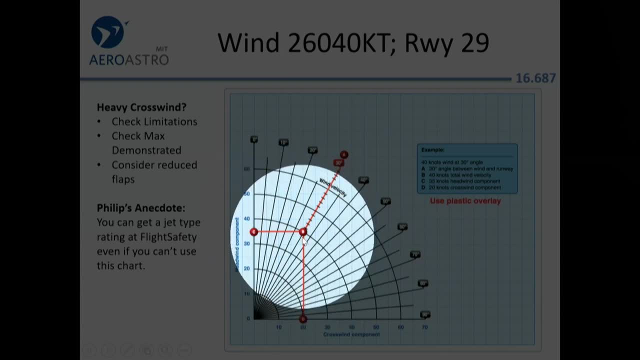 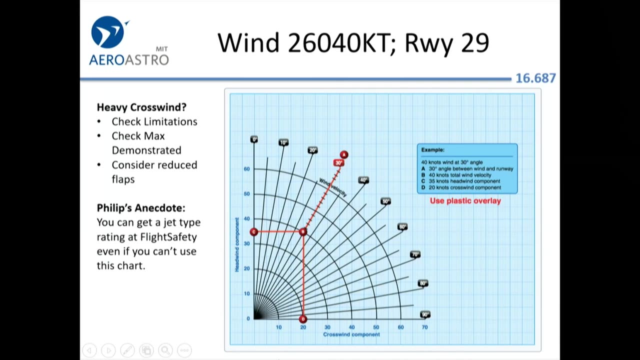 You use this 40 knot ring And then you can find that it's a 35 knot headwind And it's one knot crosswind. Does that make sense? I will tell you when I was getting a type rating for this Cessna Mustang. 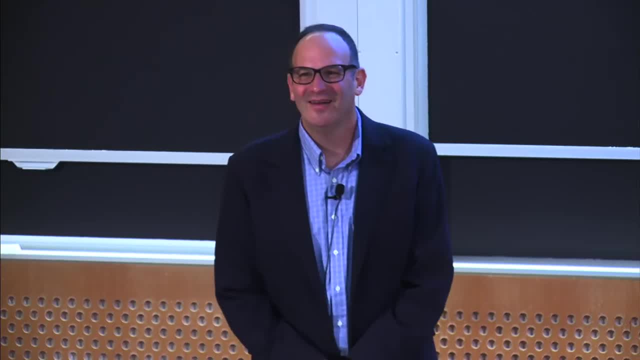 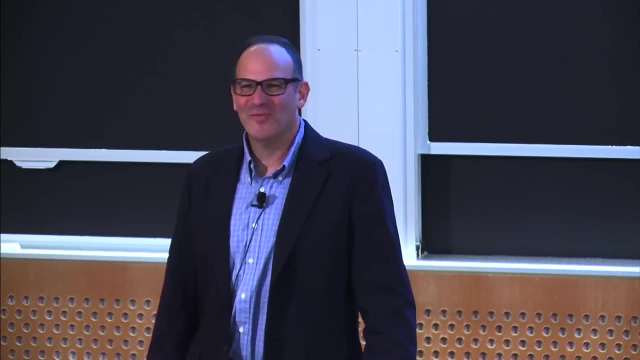 Safety. There were a couple Boeing 737 pilots there And they had no idea how to use this chart And they couldn't even give the right answers, Like if you said you're landing on runway 27.. And the wind's coming from 315.. 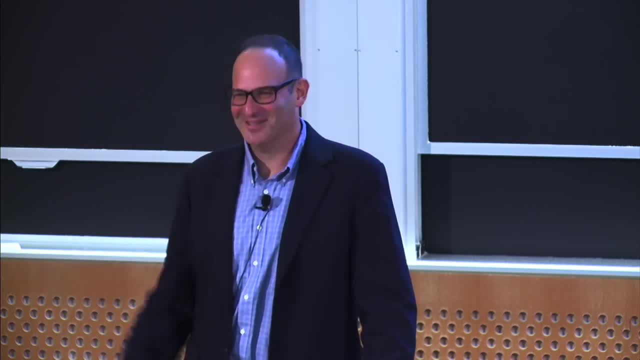 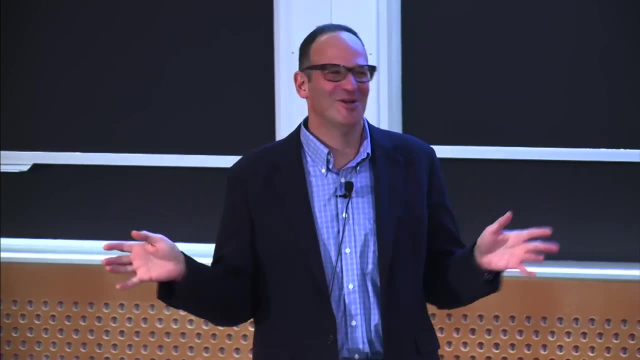 Is that a tailwind or a headwind? And they couldn't answer that question either. Basically, all they do is go from towered airport to towered airport. The tower tells them what runway to use. They were from the Philippines, So I guess it's not insanely windy there. 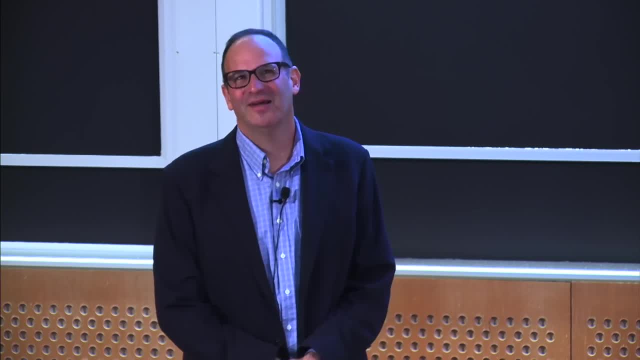 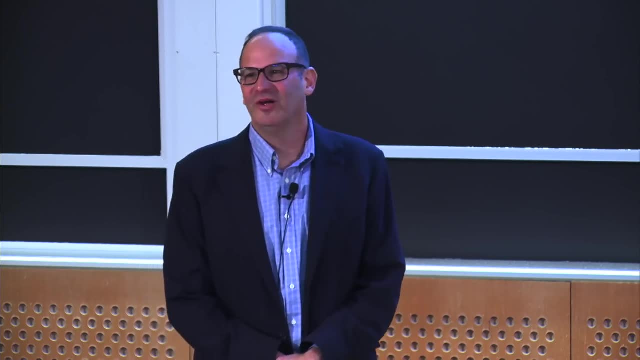 like it would be in Argentina. I once landed in Argentina, in Ushuaia, on a commercial airline flight And it was 50 knot, The wind was, I think, 35, gusting 50. And the pilots- I talked to them afterwards. 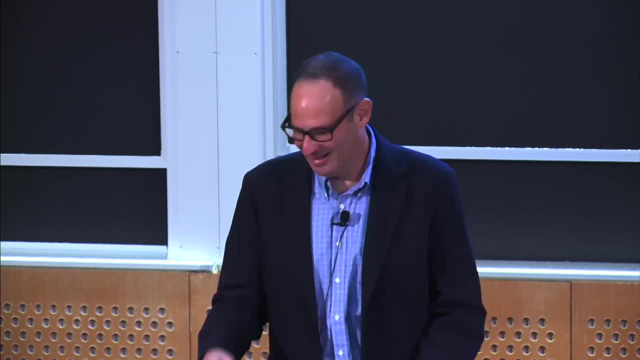 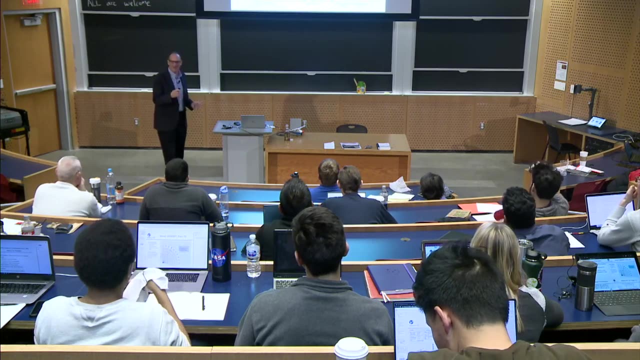 They said it was just a normal day, They wouldn't even bother talking about that. So anyway, these skills apparently rust. I'm sure those guys You know had used a chart like that at one point in their training. They did get their typewriting. 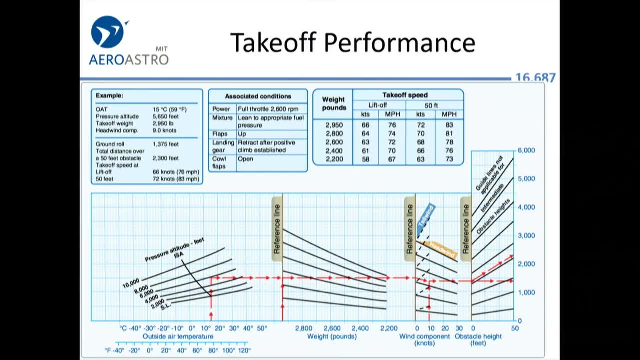 So the good news is you can get your typewriting without knowing how to use that. OK, here's one of the FAA charts. This is what they give you on the test. It's a lot easier to use than the POH. 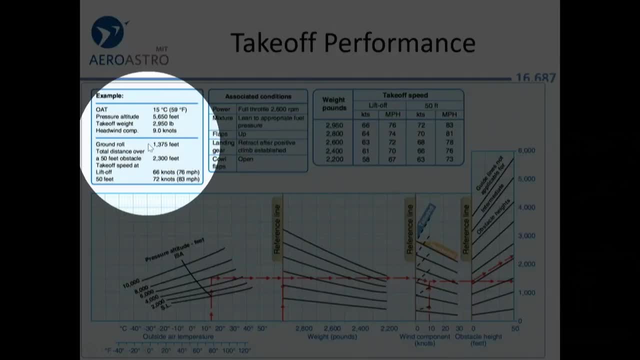 Here's a problem. they're giving you an example problem. Let's see, We're at somewhere in Colorado, apparently 5650 feet. We weigh 2,950 pounds in this airplane that they won't tell us what it is. 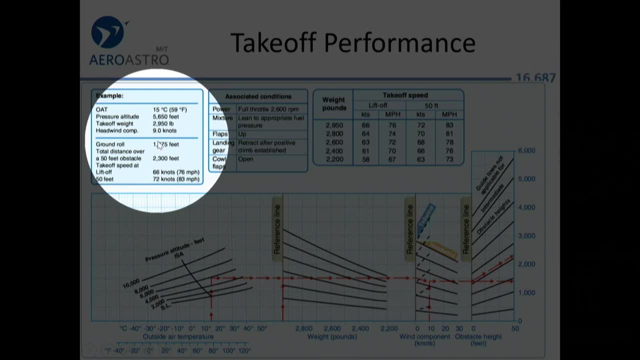 It's 9 knots Of headwind. Notice these associated conditions. These are really critical. And again, if they give you a choice of multiple charts, that's where the trick is. You know they're trying to get you to use the wrong chart. 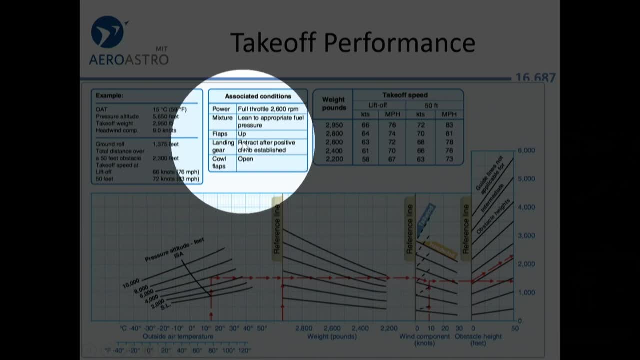 That's more on the ATP exam than on the private one. But yeah, see here, powerful throttle cowl flaps are open. This is some kind of more complicated plane that you've got the right mixture set even before you're going to take off for high altitude. 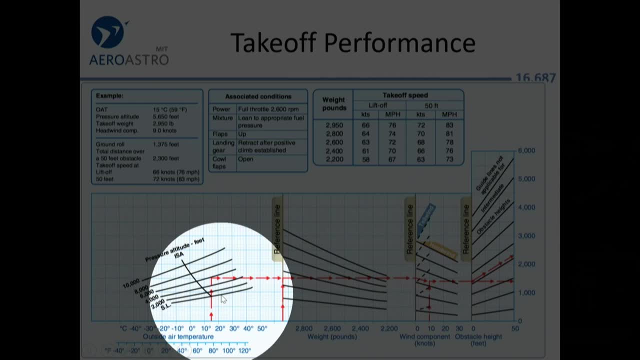 All right. So what do we got here? We got temperature of 15.. We go up to the pressure altitude pretty close to 6,000.. We come over here. We're apparently right at gross weight, so at least that's realistic. 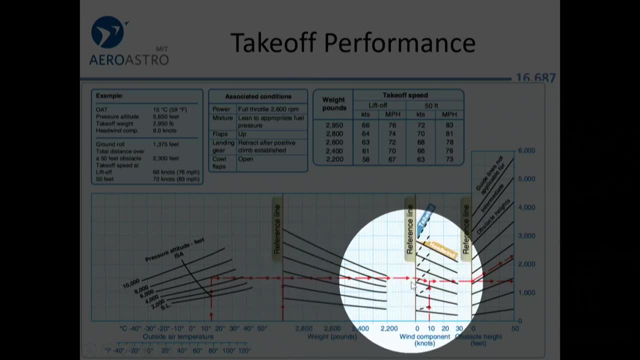 Most aircraft take off right at gross weight. for most flights There's 9 knots of wind, so that's going to subtract a little bit from our runway requirements. And here we can see: it's 1,500 feet, 1,500 feet. 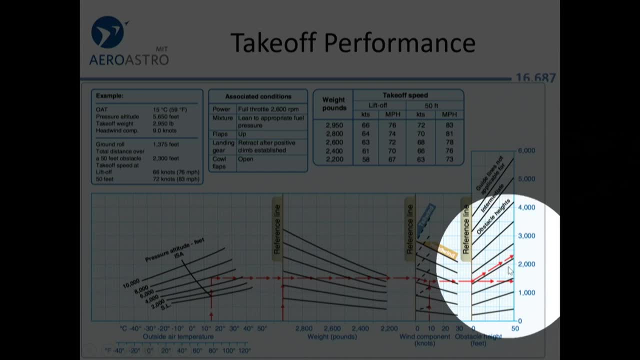 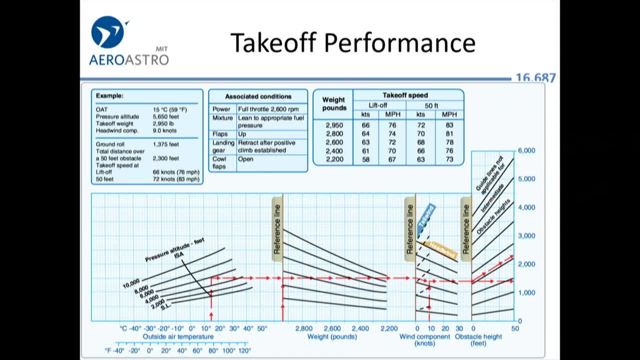 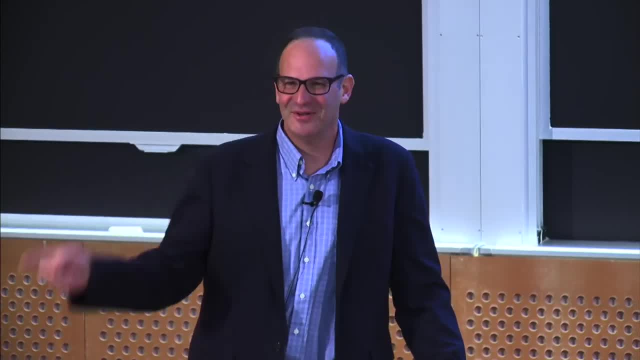 Yeah, 2,300 to clear the 50-foot obstacle. So these charts are not hard to use And in the real world, maybe in the FAA figure, they actually give you this example So you can see how it's done. 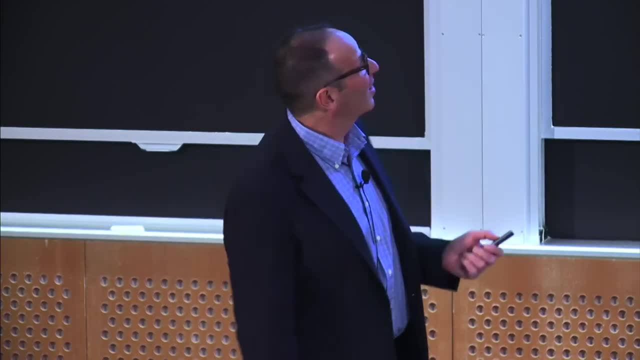 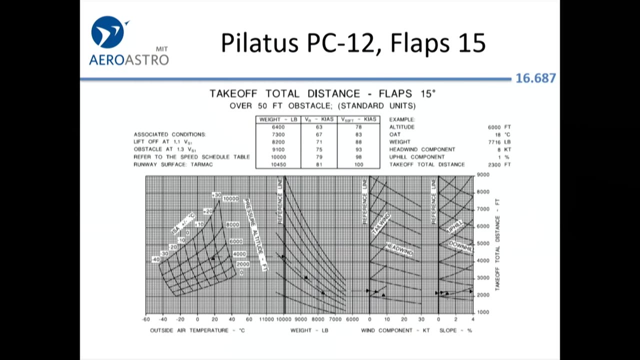 And then you just draw the lines in a different place, So they're not trying to trick you. Here's a chart for the Pilatus PC-12.. There's also apps to do it, which I'll show you a little bit later. 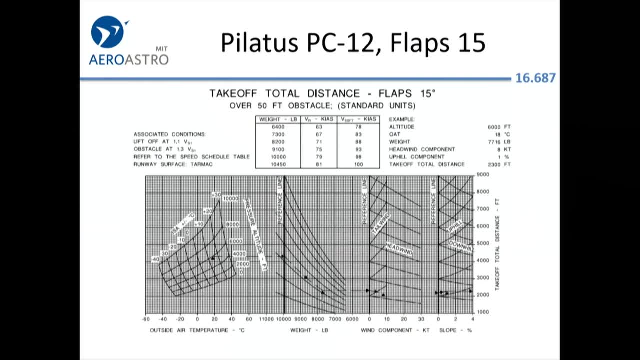 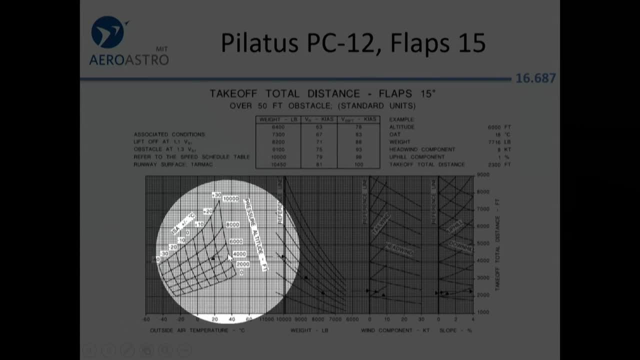 It's similar to that Piper chart we saw earlier, where you calculate the density altitude without realizing that you've calculated it. Yeah, so here you've got pressure, altitude and temperature And you're implicitly calculating density altitude. Then you go over to weight. 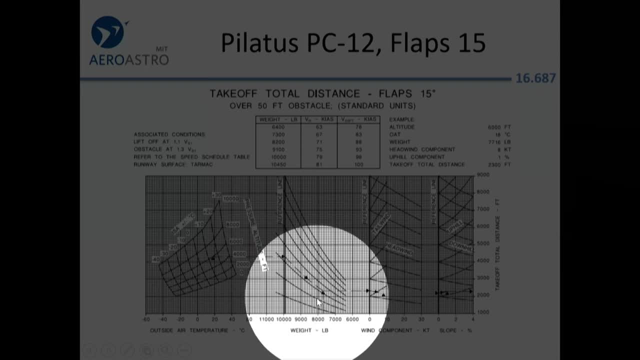 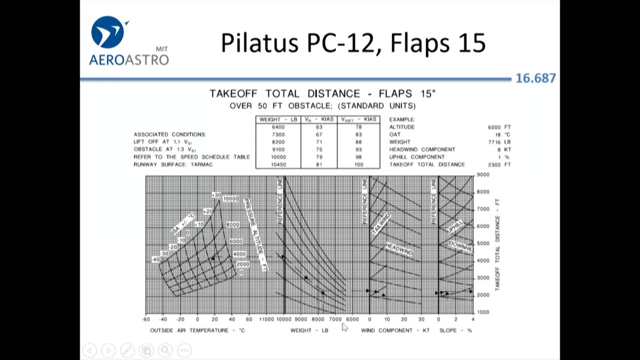 Look at this one, The Pilatus guys. I think they are having some fun here. They're saying: you're taking off at 7,000 pounds, So you're missing almost 3,000 pounds of people in bags. You paid all this money for this airplane. 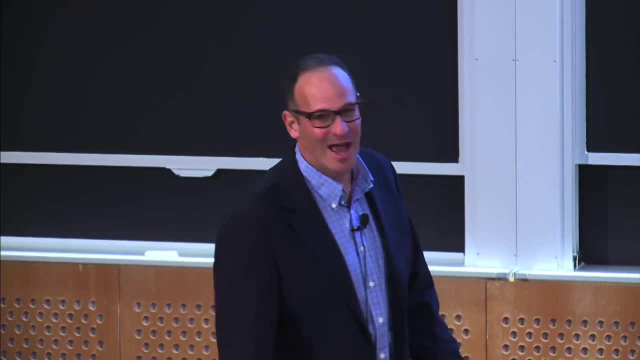 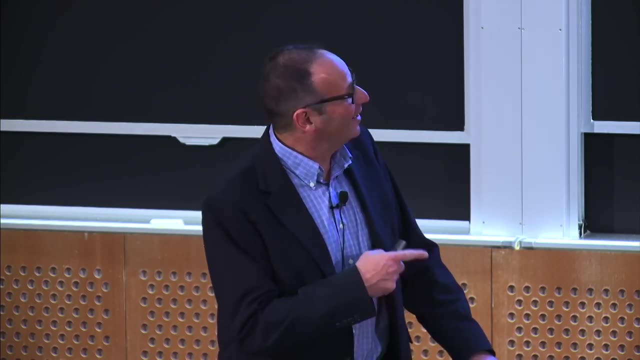 and you're barely using it. So I don't think that happens too often, unless you just dropped everybody off at an airport with no fuel and you're repositioning, Anyway. so they got the headwind, They got uphill and downhill, all baked in this nice chart. 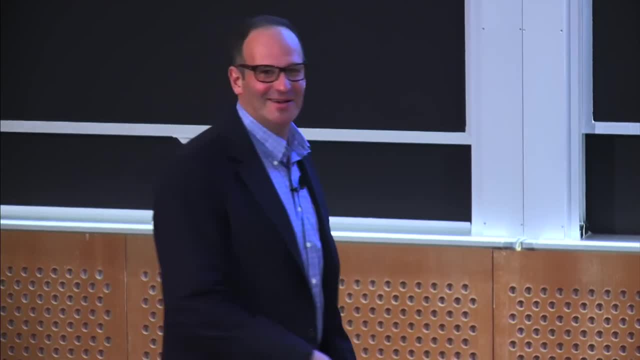 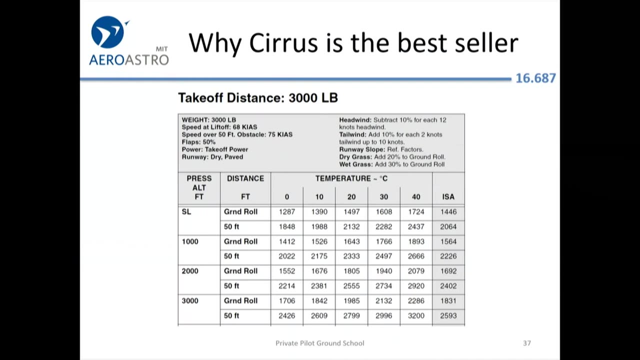 You can get all these good numbers. This is why Cirrus is better, Why they're the best seller. They just say: look, here's this table. There's a few corrections that you can use if you want to, up there in the upper right for headwind, tailwind grass. 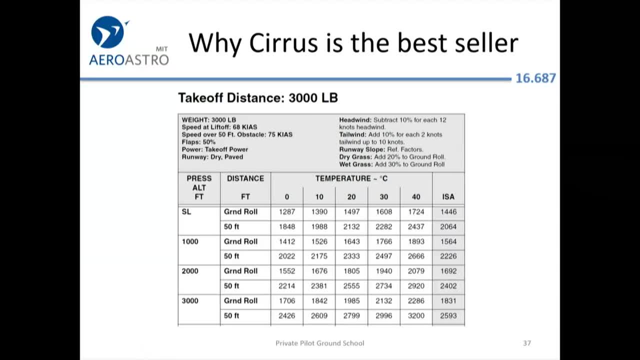 But basically they make the usual case very simple of a level runway, a paved runway. It's always more conservative to go more. You don't have to interpolate, You can just say: well, it's 25 degrees, so I'll use the 30-degree number. 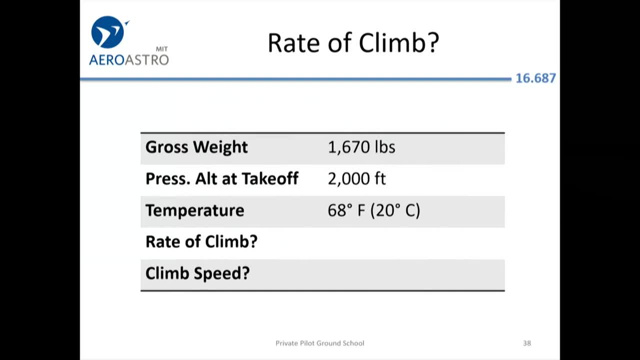 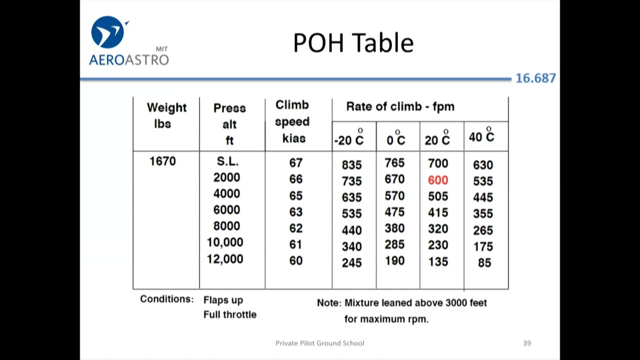 OK, what is the rate of climb? here We're at a gross weight of 1,670 pounds. It's 2,000 feet. How do we figure that out? This is one of the FAA example tables And it's as simple as finding the right row in the table. 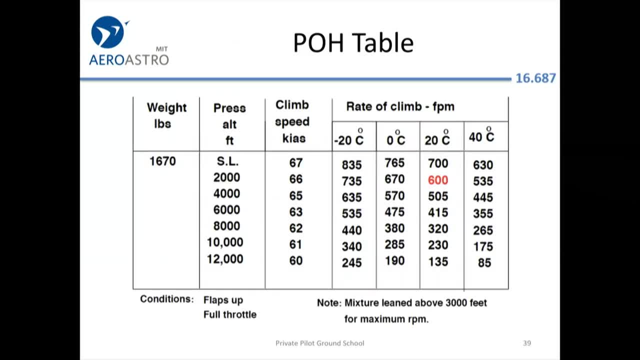 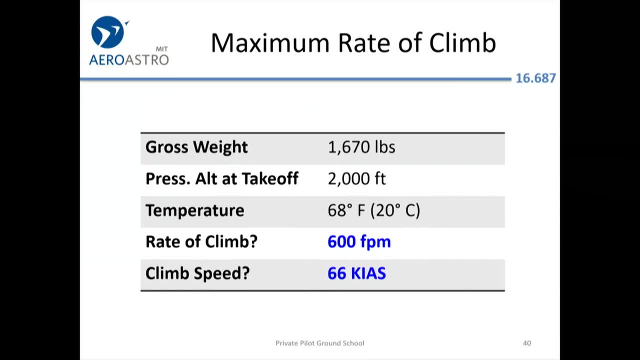 row and column in the table. Oh, actually I have a look here. So they're saying the mixture has to be lean. to get these numbers, The flaps have to be up, You've got to be at full throttle. OK, same deal. 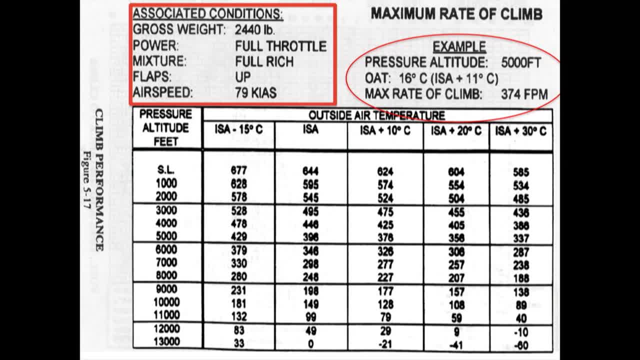 Max rate of climb. I forget if this is a. This might be a Piper chart, But you can see that associated conditions up there in the top left. That's absolutely critical. You know the gross weight Cirrus, actually a lot of the performance numbers. in the Cirrus for cruise speed are at 2,600 pounds And you're flying along at 2,950, because you took off at 3,000.. You're wondering how come I'm not getting these numbers, But of course you know. 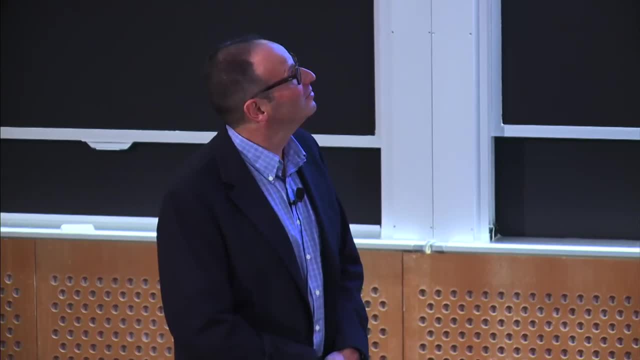 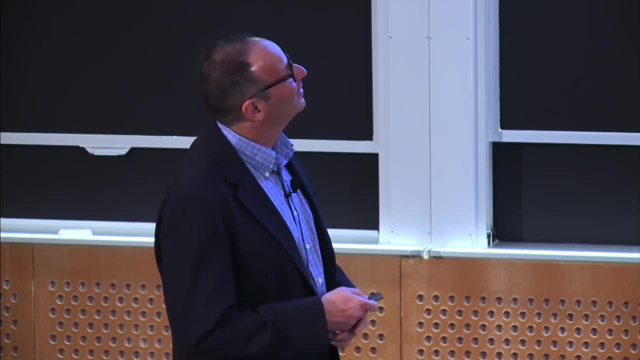 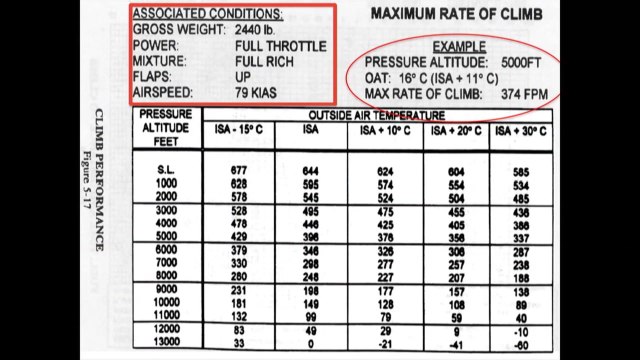 They're, They're being optimistic about, They're putting their airplane in the best light by positing some weight that probably doesn't exist in real life. All right, here they give us an example of 5,000 feet pressure altitude, OAT of 16 degrees, so iso plus 11,. 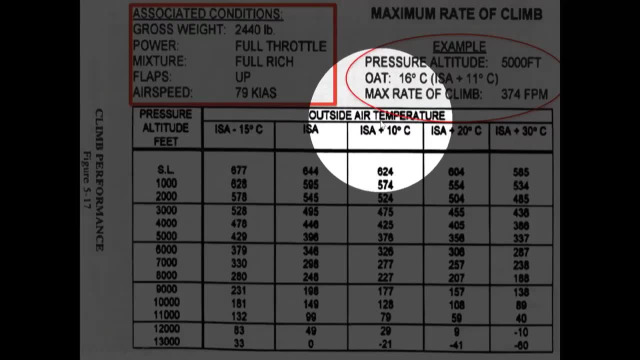 max rate of climb: 374.. So I guess, yeah, 5,000 feet. Here's iso plus 11. It says 376.. With some kind of an elaborate interpolation I guess you find that last couple of feet per minute that you subtract. 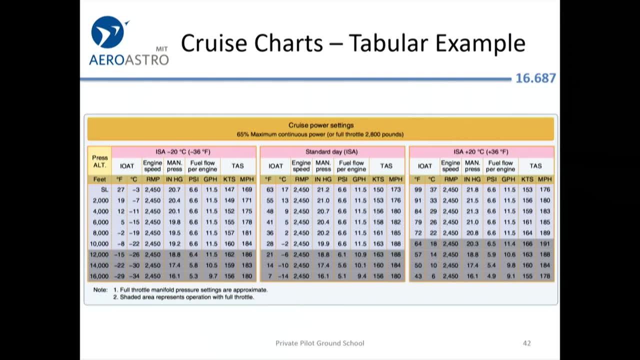 Here's cruise charts. I think again, this is from the FAA test supplement. They're just giving you a Remember. I told you it would be iso minus 20.. That's the chart on the left. The one in the middle is a standard day. 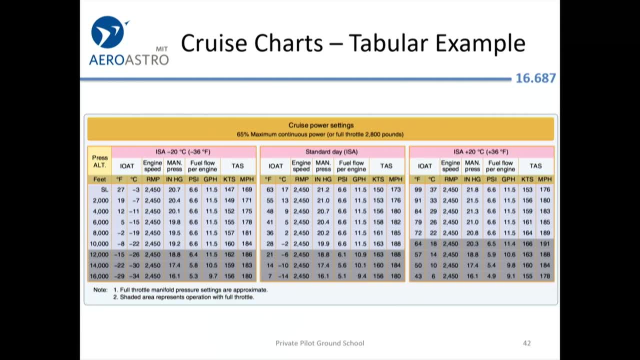 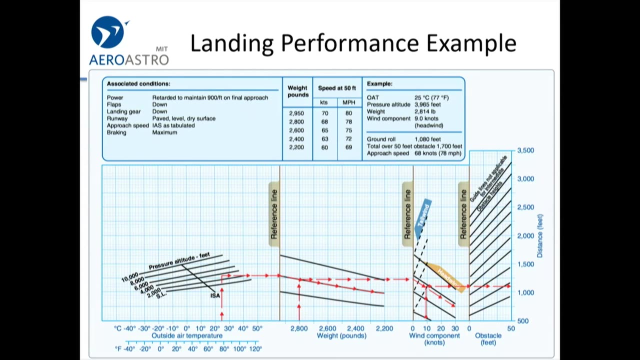 And on the right is a summer day, iso plus 20.. Notice that they'll give you fuel flow and the true air flow, True air speed, given various engine speed and manifold pressure settings. This looks like it's for a piston twin. OK, landing performance is pretty. similar kind of chart. 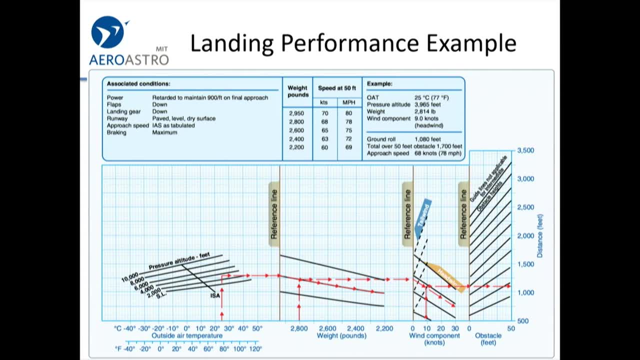 I'm not going to go through this exactly, but you can see they're giving you the worked example And you come up with: let's see, it's going to be about a little over 1,000 feet of ground roll and 1,700 feet, they claim, of. 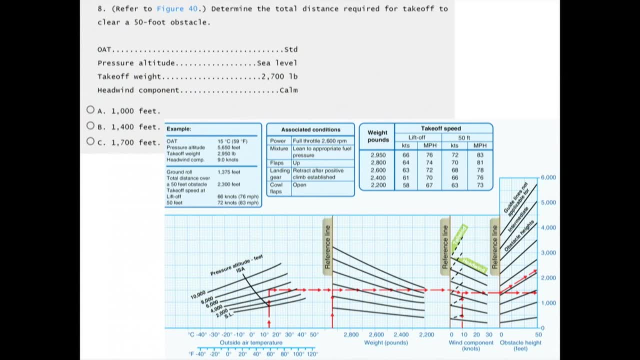 To clear a 50-foot obstacle. Here's an FAA question actually. So let's see: Determine the total distance required for takeoff to clear a 50-foot obstacle. Standard temperature, sea level. So actually this is testing you. 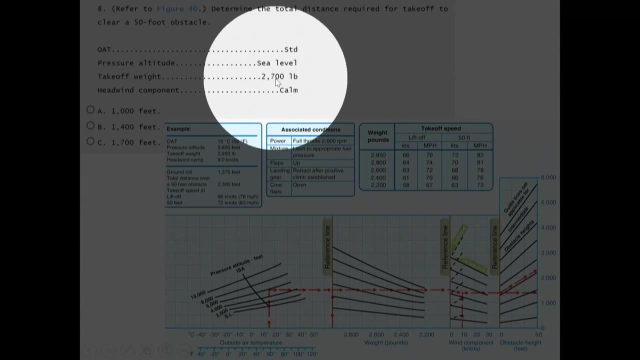 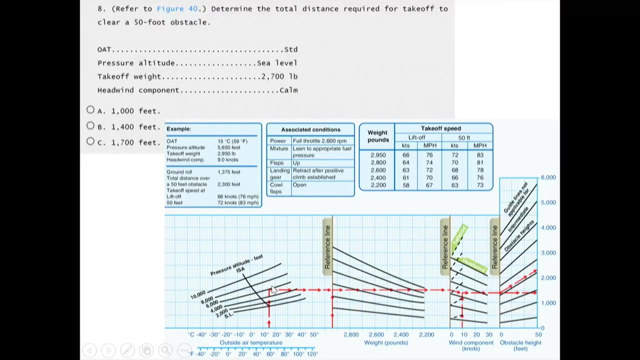 This is pretty advanced, right? They're saying it's the standard temperature at sea level, So you have to know that it's 15 degrees. We only weigh 26., 26., 26., 26., 26. 26.. 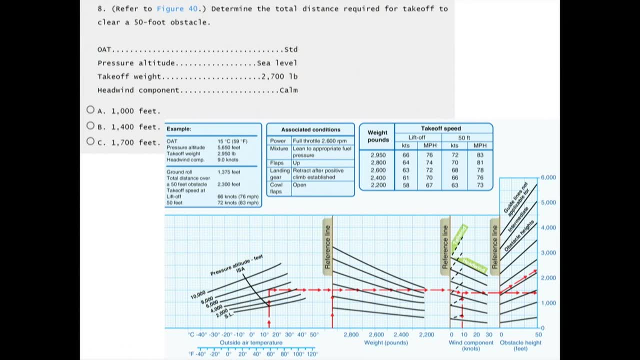 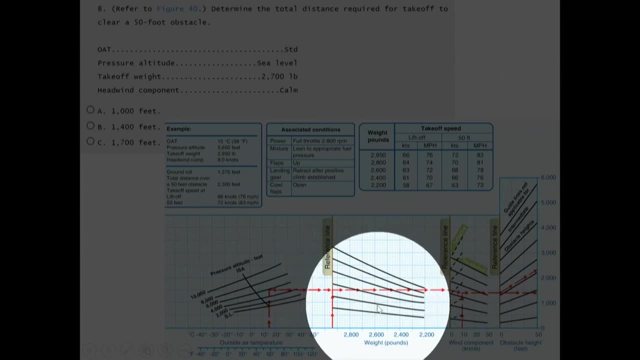 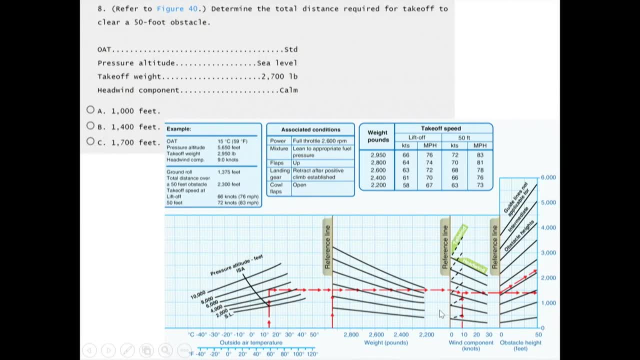 And the wind's calm, so we're not going to get any boost from the wind. So what do you guys think? Have any of you been able to kind of see what the most likely number is by following these? Somebody says A, Let's see. 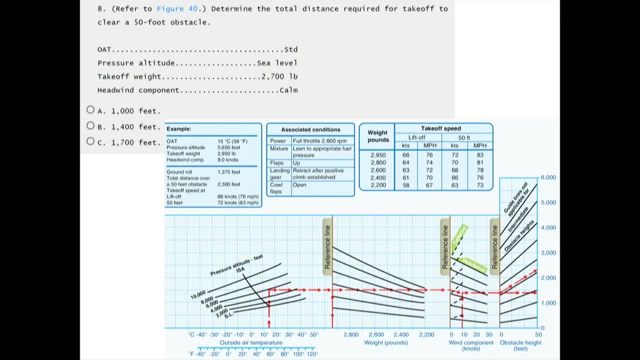 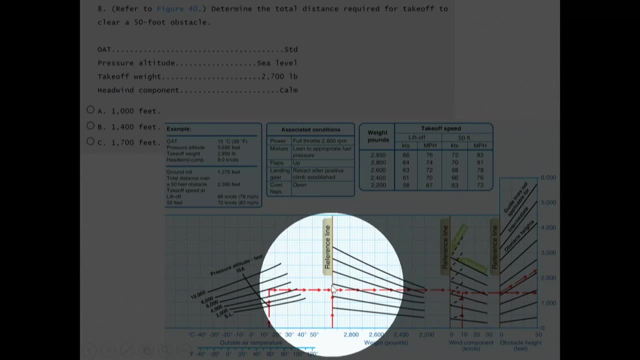 It's a little bit lighter. That kind of makes sense. But on the other hand the wind's calm. So we didn't get that reduction from the wind, Let's see. So if we came down here, it's going to start from sea level. 15 degrees come over here. 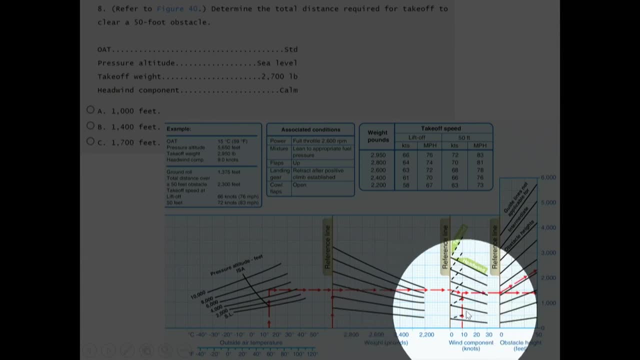 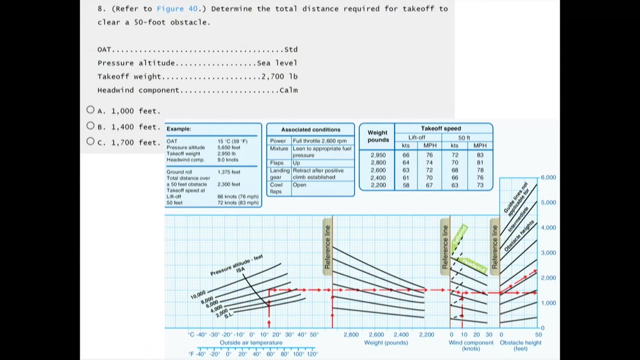 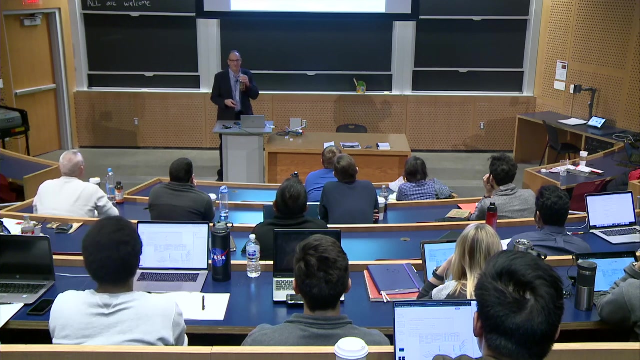 come down here over a 50-foot obstacle And then we have to go up. Anybody want to revise their estimate? We heard A last time. It seems a little short to clear the 50-foot obstacle. I agree with you that you'd be well off the ground. 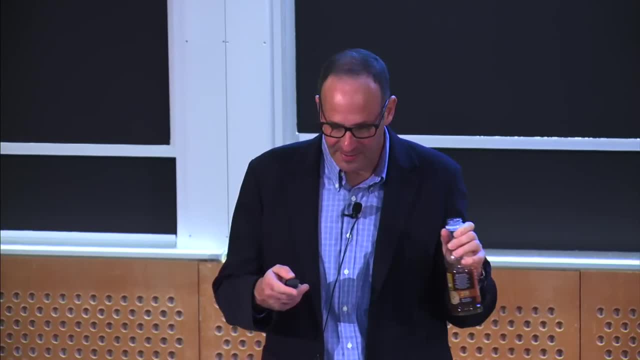 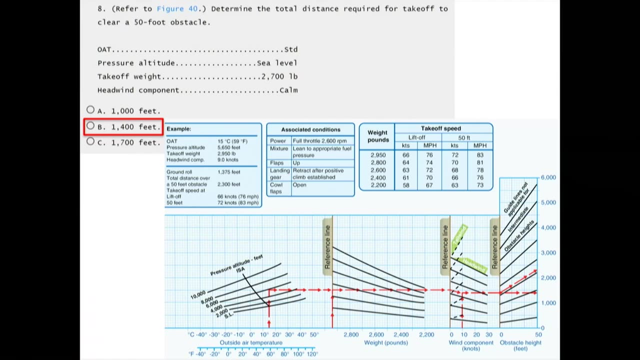 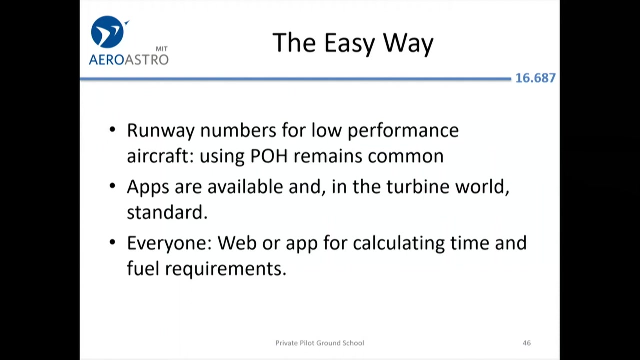 by 1,000 feet Ta-da. All right. Obviously, if you have a pencil and a little more time to do that, it's easier. All right. That's kind of the hard way. Let's look at the easy way. 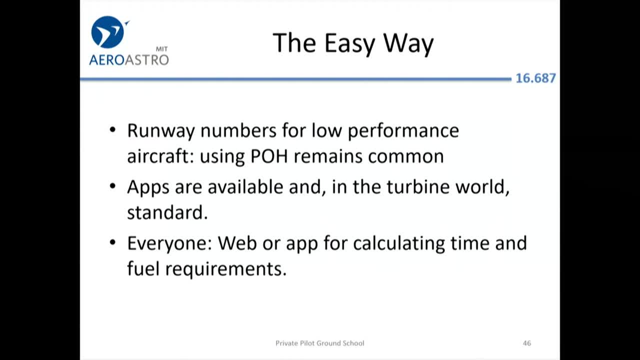 Getting the runway numbers for low-performance aircraft. it actually remains pretty common to just use the POH. People aren't usually in a situation where they have to worry about it. If you're going from Hanscom Field to Martha's Vineyard and back, both airports are big enough for a Boeing. 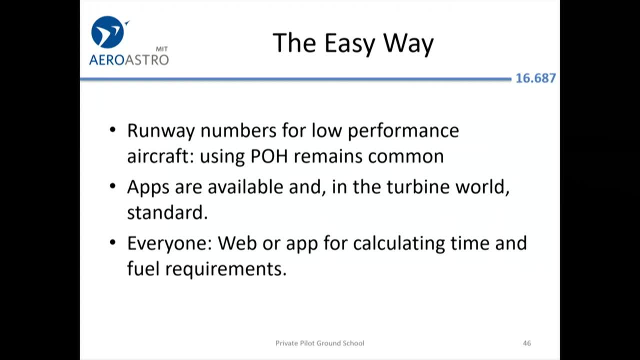 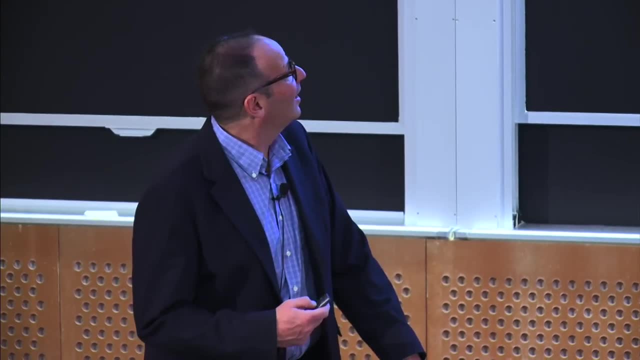 And you're not going to be carefully calculating these numbers unless you really don't have much else to do. Apps, though, are available even for low-performance aircraft, and they're very useful if you're going into tighter airports and you might have to worry about that. 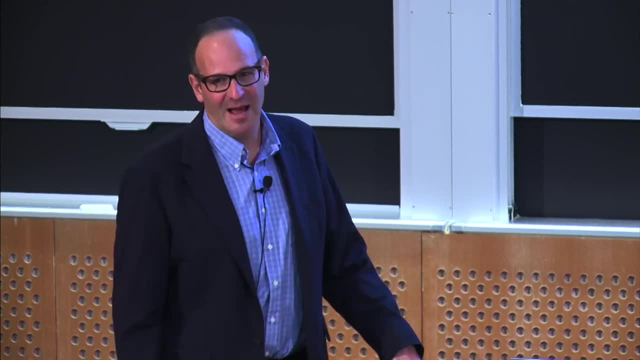 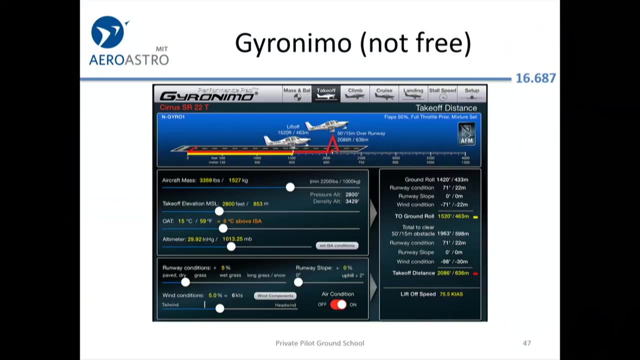 The time and fuel stuff is everywhere on the web and the apps, But the actual runway numbers are a little bit less common. Let me show you a couple things. Here's Gyronimo, So they sell these for different aircraft. This is just off their website. 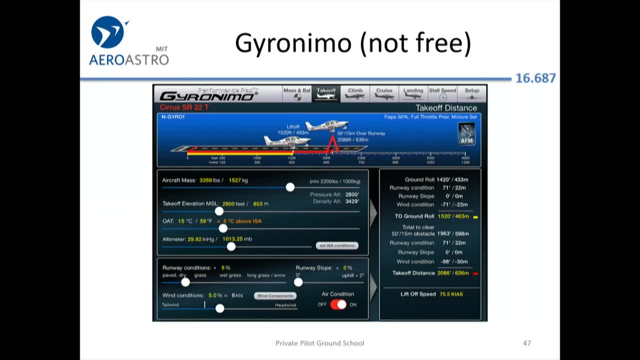 And for an SR-22, you can see, you put in the top right, the bottom left And they must be European because they say aircraft mass 3359.. And you've got your temperature, your takeoff elevation, your altimeter, runway conditions. 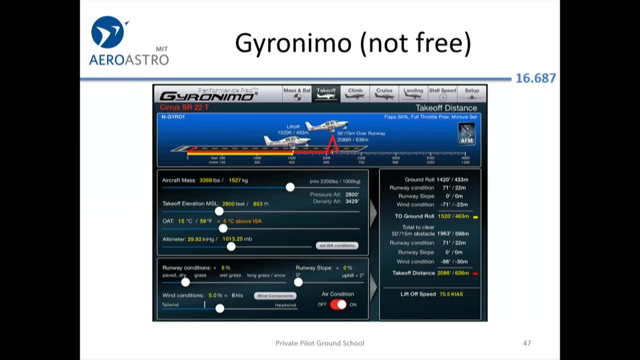 I don't know what that plus 5% is. Maybe they're saying: oh, I don't know if that's between, Is it half grass and half paved? Anyway, you can put in everything relevant and it's going to tell you how much ground roll. 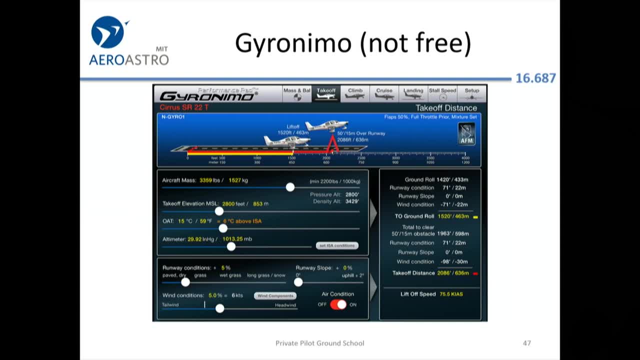 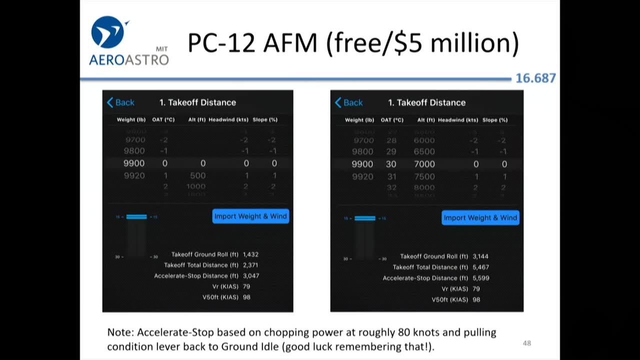 and how much takeoff distance. So that's pretty slick. It's a lot easier than relying on the POH. The calculator for the Pilatus is free, That's the good news. And here, same deal. You put in your weight the temperature. 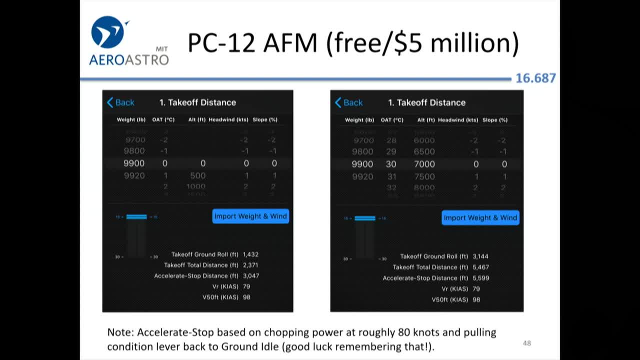 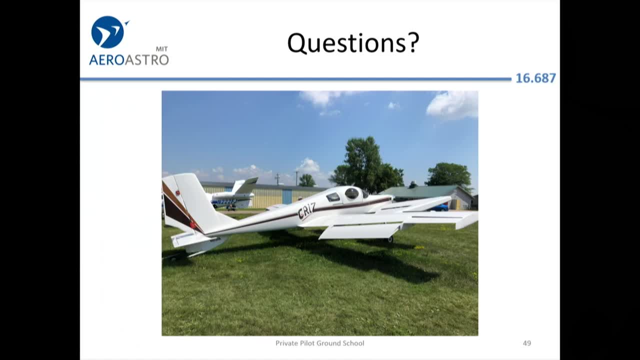 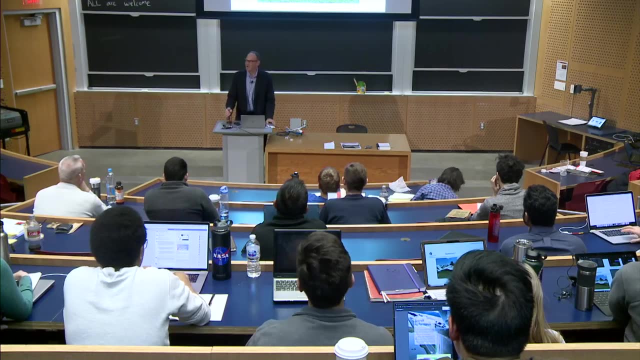 if there's any headwind, the airport elevation and you get the numbers All right. So we can try to get the dock camera working for a demo in a minute here, But in the meantime, first of all, are there questions? 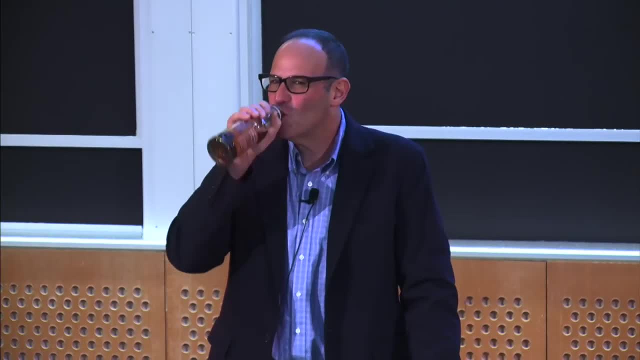 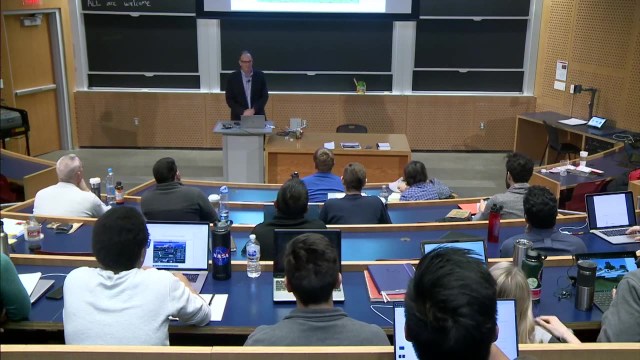 And secondly, what is this aircraft and what's it designed for? Question about the test. Would it be able to print it out, though? Print what out, The test, like they say for this FLAS, because it's online right. 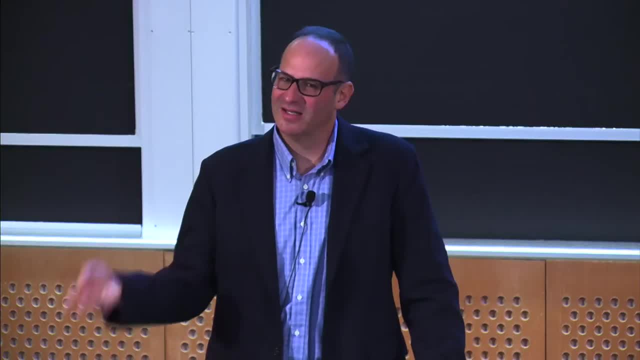 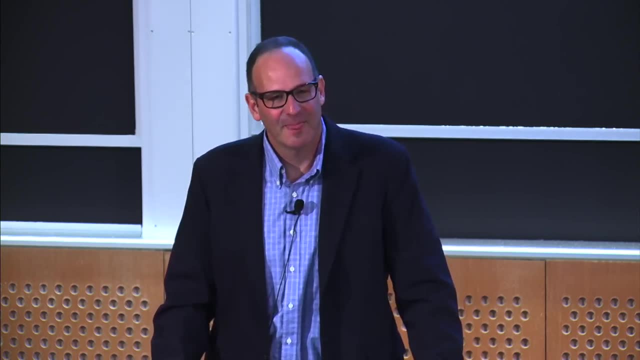 Yeah, Well, you can print out the test supplement. That's public, It's in our Dropbox and also the FAA makes this chart supplement public, so you can see all the figures that you're going to see before the test- I think actually when you're done with your test. 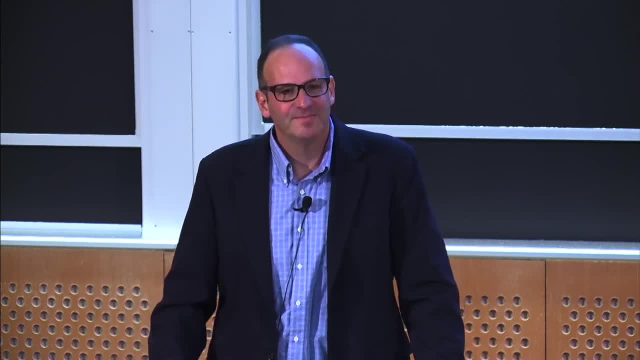 I think you can print out all the questions and it'll show you what you got right. OK, I just feel like, for the graphs, this is going to be hard for me to do it. Oh yeah, Yeah, just print out the chart. 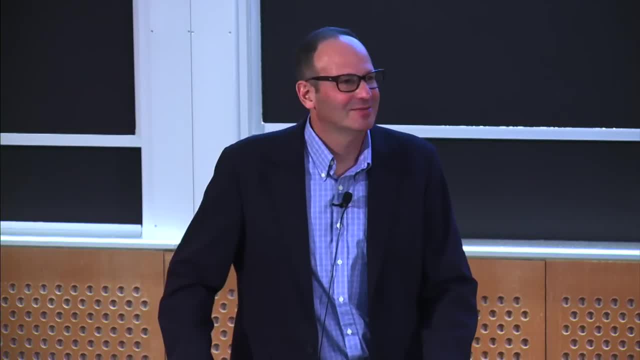 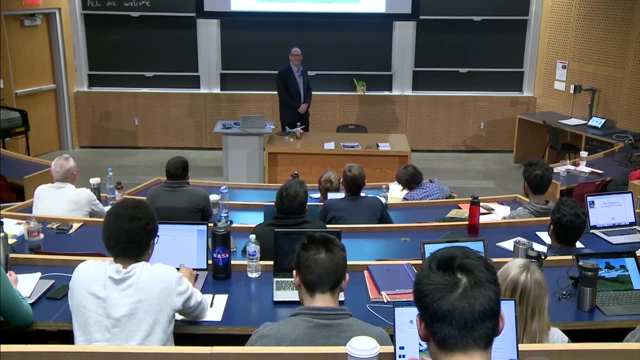 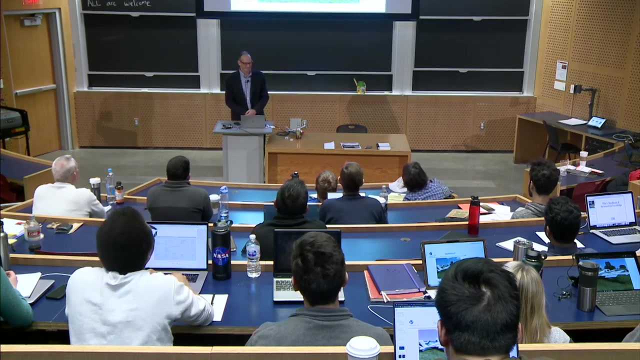 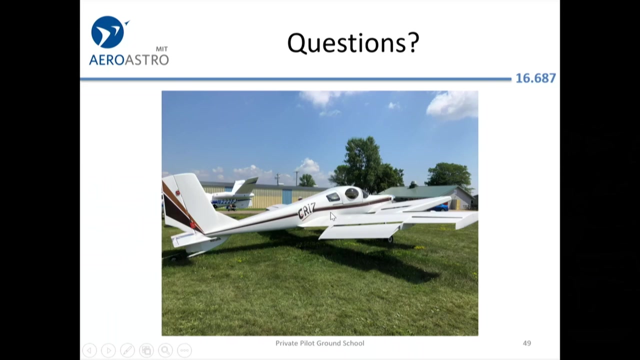 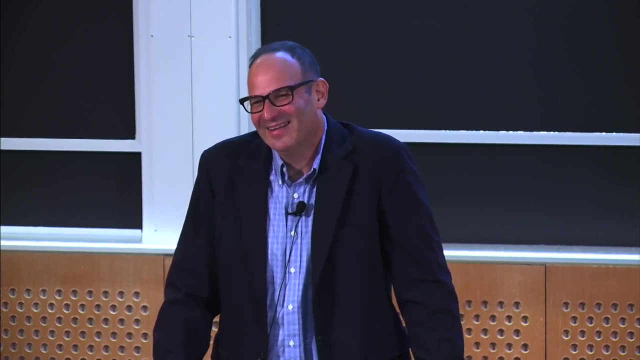 Yeah, print out, Sure, Print out the chart and supplement. Anybody have any brilliant ideas about this aircraft? It says GRIZ on it. That's a Burt Rutan design, the climate change denier, And this is a super short field airplane. 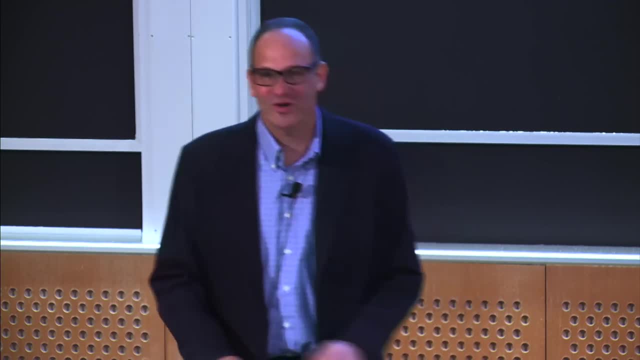 It actually doesn't land as short as you might think. I think it might be a four-seater, though, So I guess it is pretty darn short for a four-seater, but it has huge flaps And a lot of wing area. 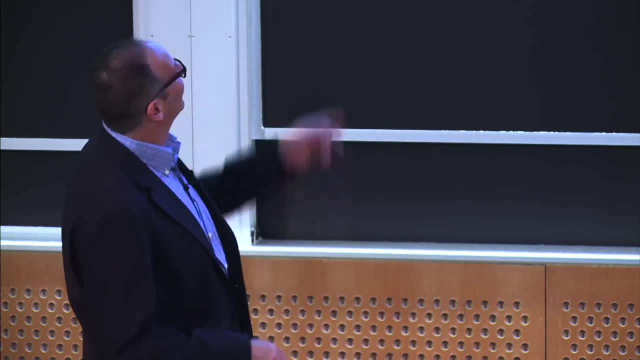 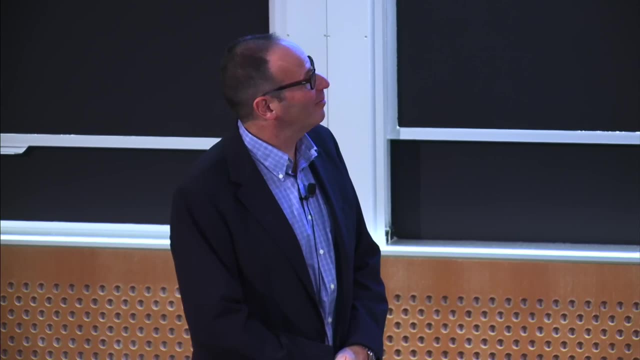 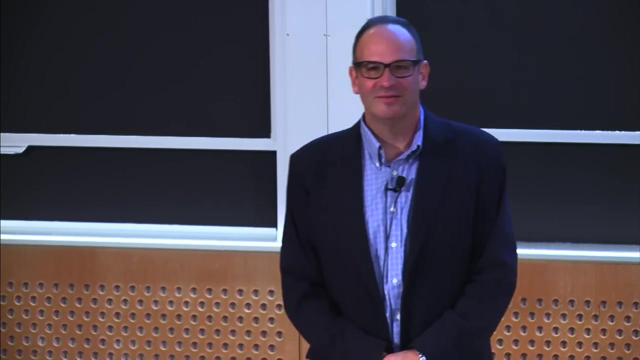 And it's got that. I think it has ordinary. yeah see, it has essentially three surfaces right, It's got kind of a helper wing or a canard out in front, the regular wing and then an ordinary conventional tail plane. 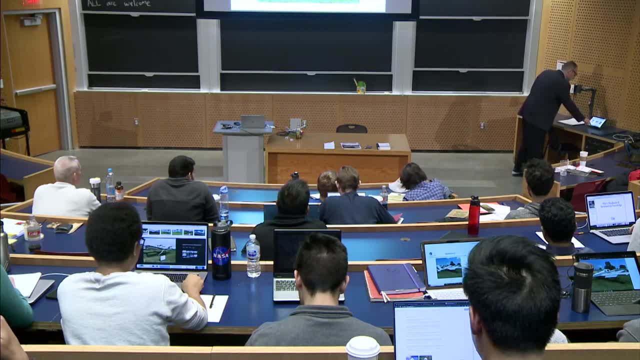 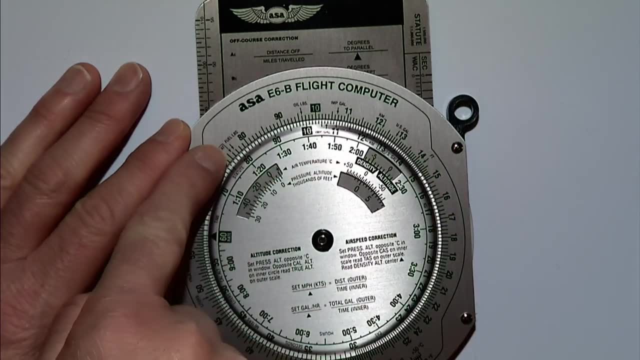 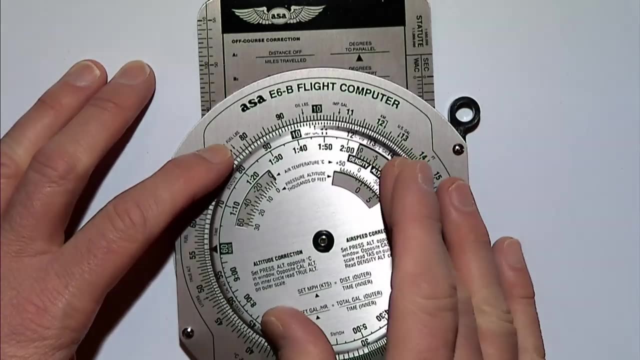 Let me see if I can get this dock camera working. All right, All right. So let's say we want to know how much fuel we're going to use. See that fuel pounds. there We can. where is that? Somewhere along here. 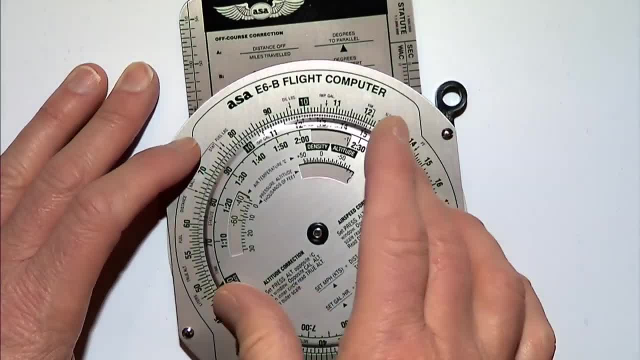 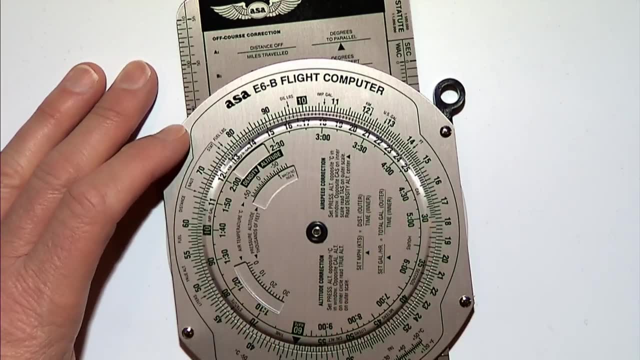 Well, actually I happen to know it's got to be somewhere where 10 pounds- Yeah, see, there's US gallons right there. So we line this up And you can tell this is designed for piston folks, Because their idea of fuel weight is 6 pounds per gallon. 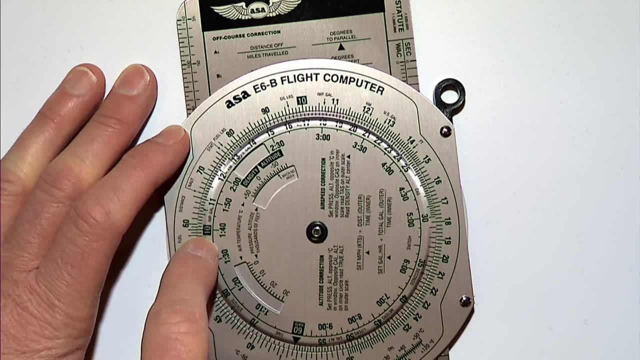 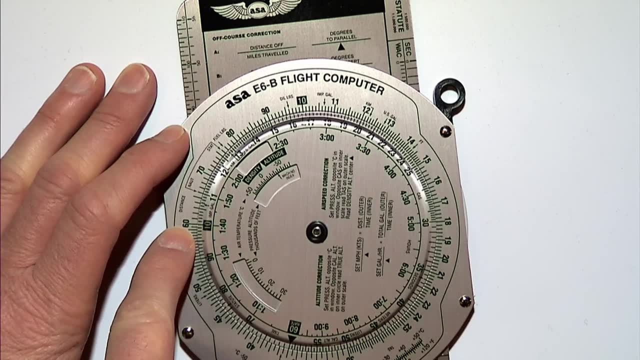 And jet fuel weight is 6.7.. But at this point now we've got our handy slide rule, So we know if we load on, for example, 10 gallons of fuel, it's going to be 60 pounds. And if we load on, you know, the Cirrus holds 56 gallons. 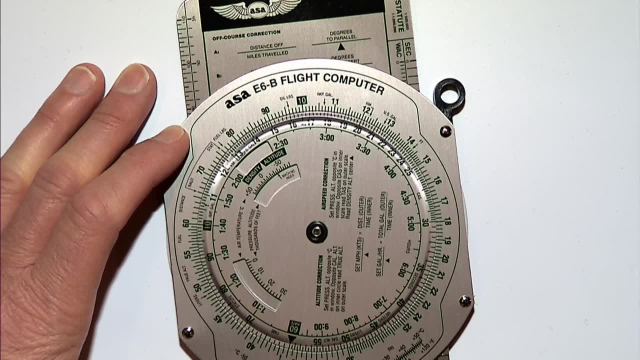 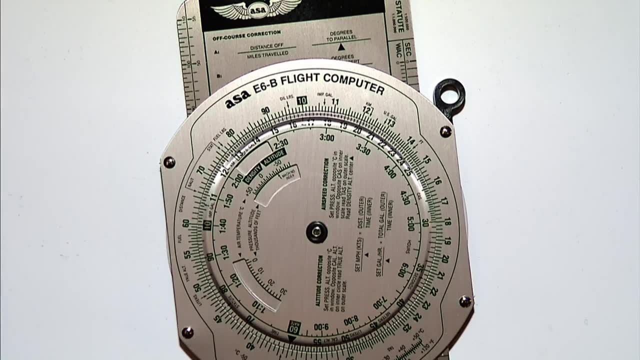 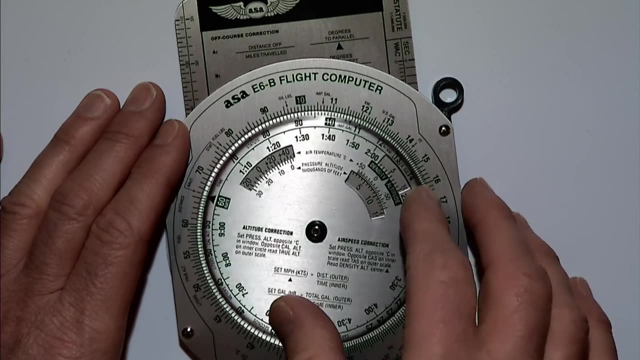 That's going to weigh 300 and looks like 345.. Oh, sorry, Sorry. 335 gallons, It's 335 pounds. More to the point, you can calculate density, altitude. So over here, for example, you can say the pressure altitude. 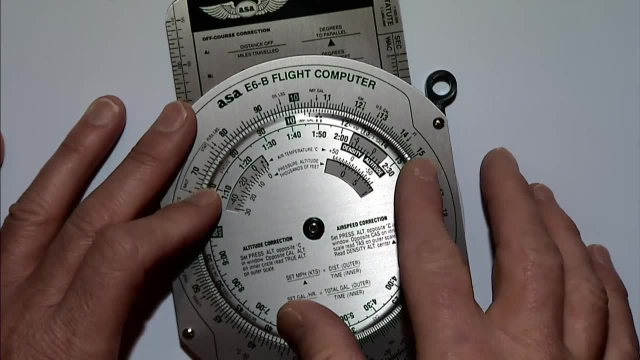 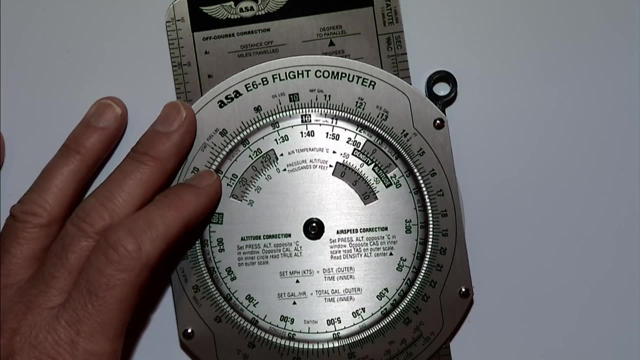 is, let's call it, sea level, And it's very hot, though It's plus 40 degrees. So now you see the density altitude up there is about 2,000 feet. Does that make sense? Does that make sense? 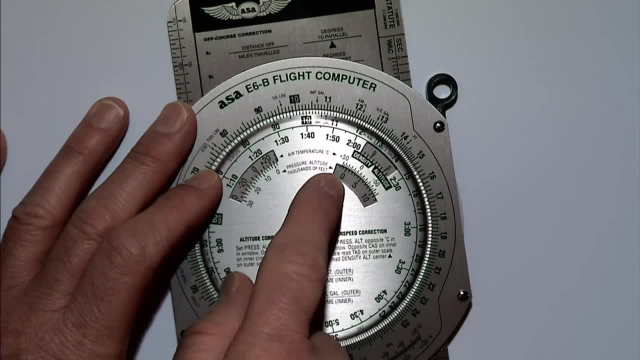 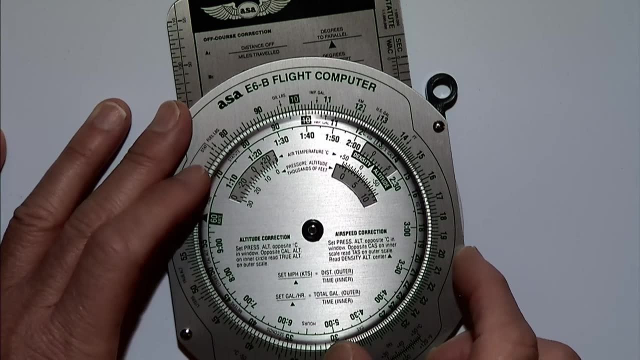 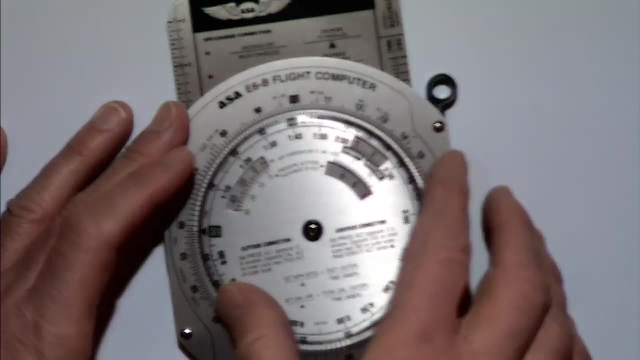 So you've set the pressure altitude at the bottom or inside this little window at 0. And then the density altitude gets read out here, after you line it up with the temperature. There's also something that you can do well, just with the basic rate. 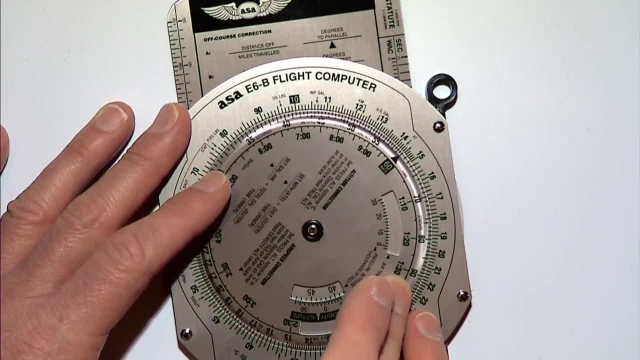 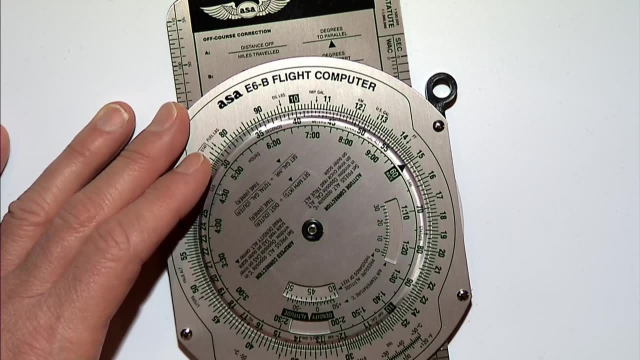 So let's say you decide that you're going to be going. This is more for performance planning. But let's say you're a Cirrus and you're going 150 knots. If you end up needing to go, let's say, 300 nautical miles, 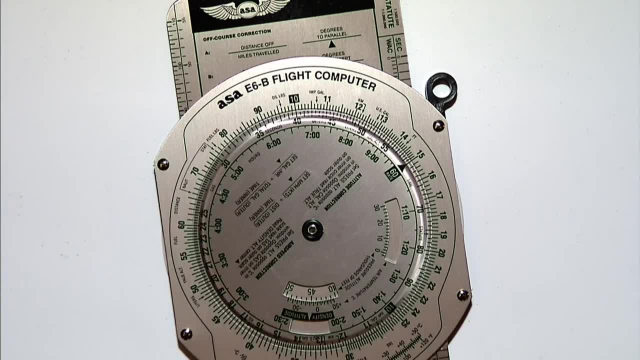 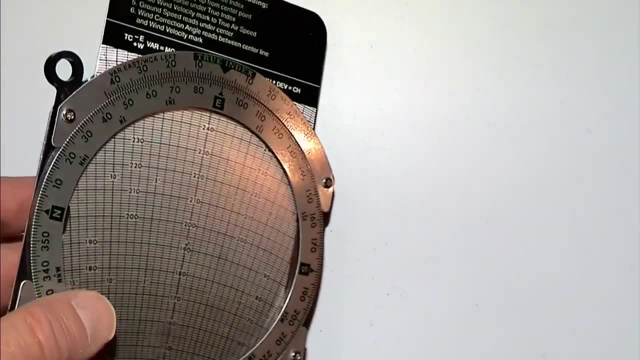 it tells you that'll take you two hours. Not too exciting, But the wind side is a little more exciting. I'll bring a pencil tomorrow for the flight planning talk And we can play around with wind vectors on there. But anyway, fortunately a lot of this stuff. 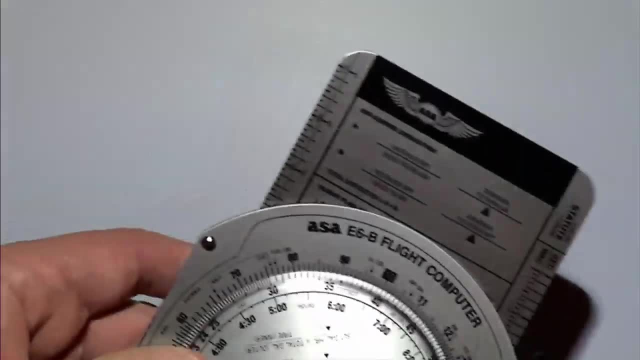 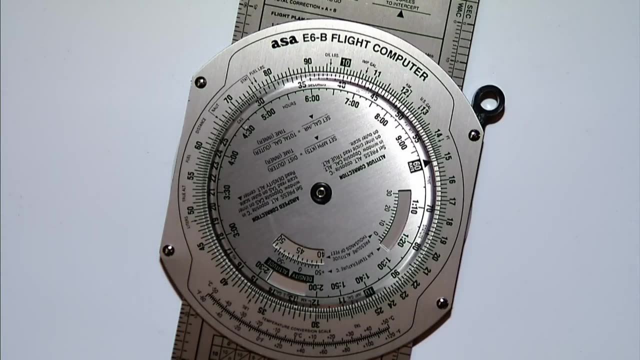 is explained in the book. You guys are free to come up and play around with it any time. There's temperature conversion Scale here on the bottom And it's a fun toy, Tina. anything else that we should cover here, Or should we segue? 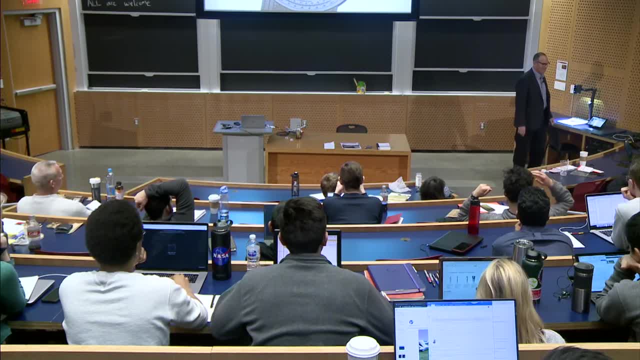 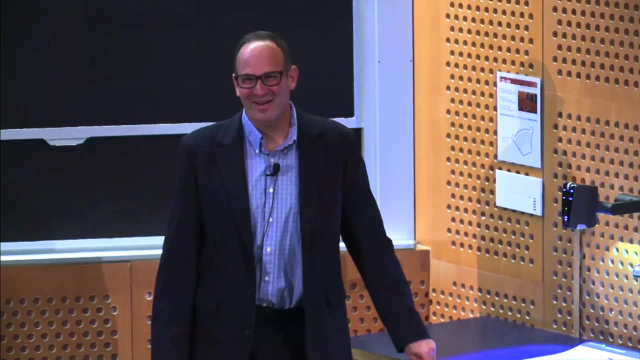 What's the next? So we're going to take questions and then do a short break and then weather data. OK, The next one's weather data. You'll need a break for that one. That's how you find out all this stuff. 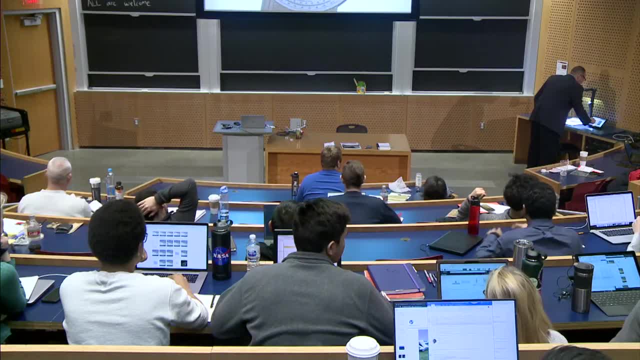 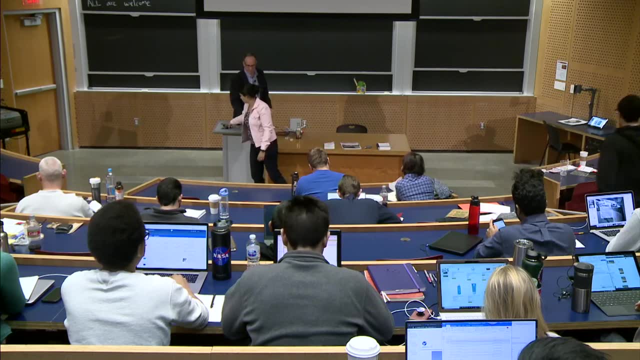 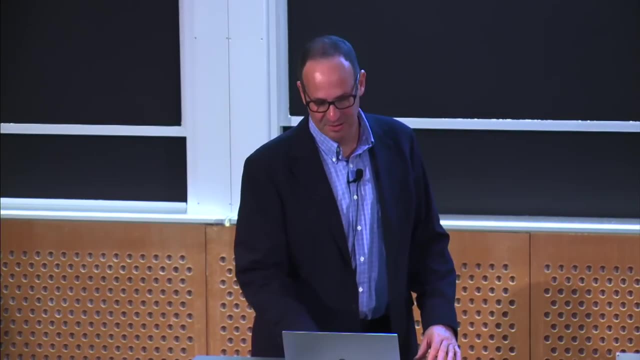 Let me go back to the PC. Who else has questions? Go back over and look at a POH graph Like which one? What you want to do with the FAA exam ones? Yeah, Landing performance. Or this one from the actual test. 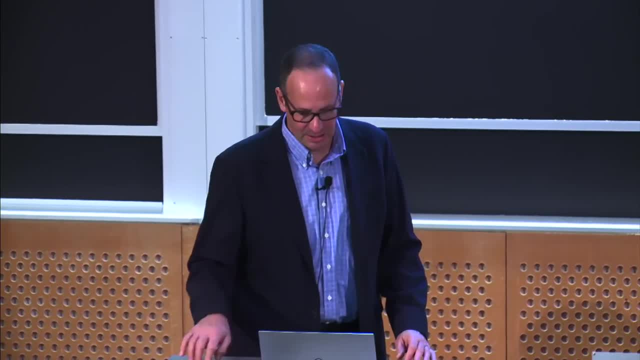 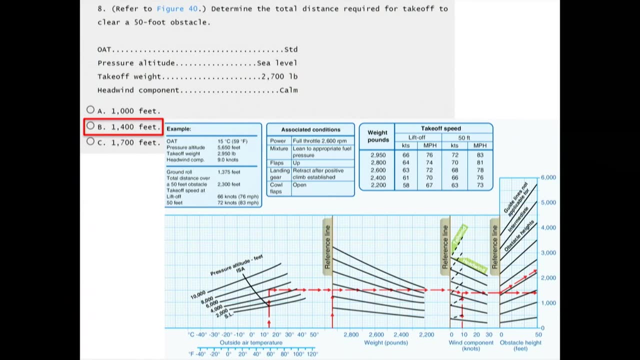 No, that was This one, Yeah, OK. So I don't think they ever give it worked out for you. Let me switch to the laser pointer mode. OK, So what did they tell us? They told us it was standard and sea level. 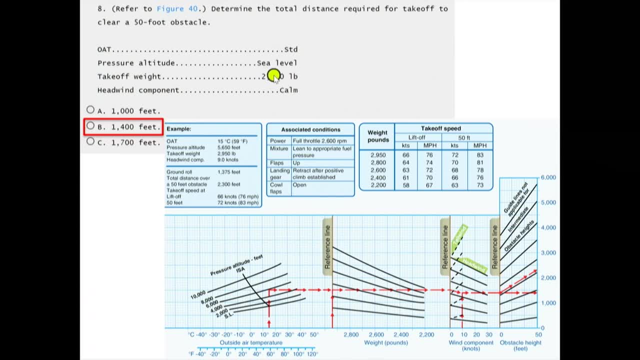 That's the one part of the standard atmosphere that people I think are expected to remember: That at sea level it should be 15 degrees Celsius. So we come down here We say it's 15 degrees out, We're going to hit the sea level pressure altitude. 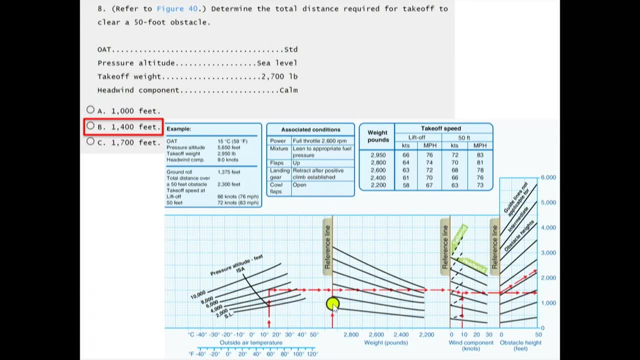 We're going to slide over this way, just like in the example, And then we're going to slide down following this curve, Ah To 2,700 pounds, And we're going to go over here And we're going to say, look, there's no wind. 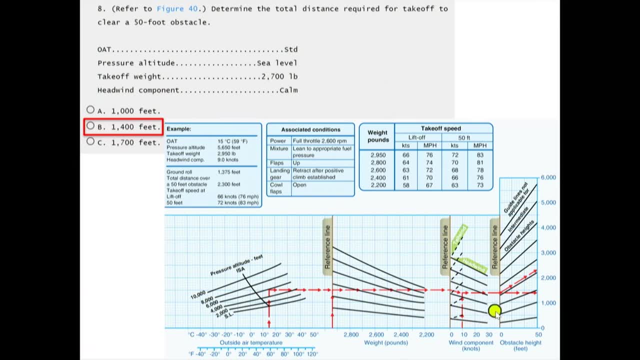 The wind's calm, So we'll keep going over here And we find that we need about a little less than 1,000 feet, maybe 800 feet, for a ground roll, But to clear the 50-foot obstacle. look at the bottom there. 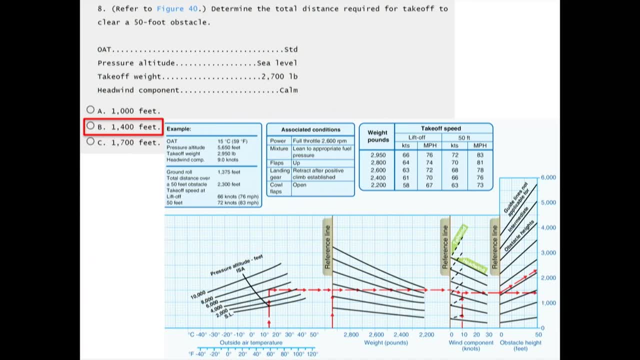 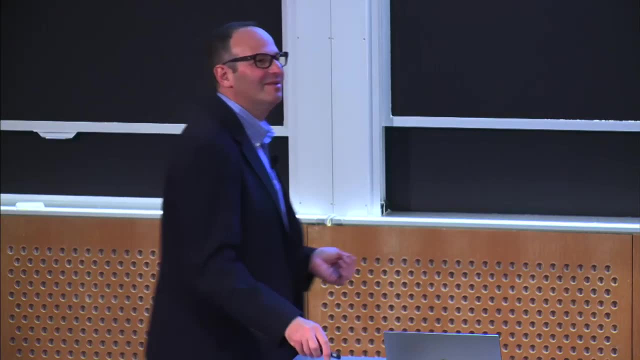 We need to go up following one of these lines And that's how we get to the floor. This is the 1,400 number. Did that help? You still look a little bit skeptical? Yeah, it just doesn't look like that line. 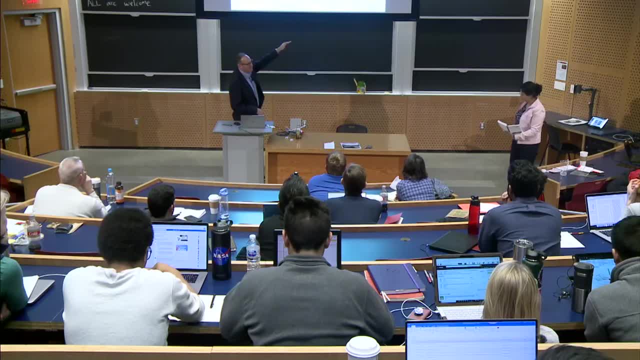 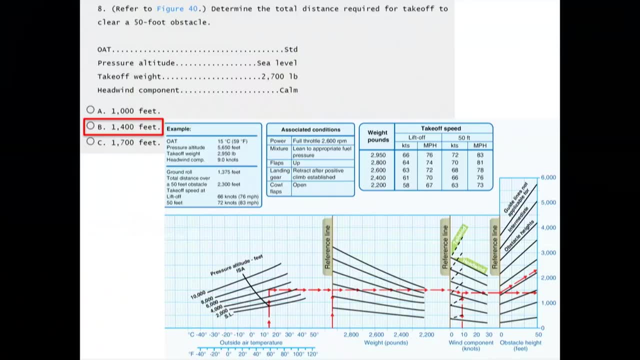 Well, remember, we would be doing this with a virtual pencil. None of these lines are just for reference, telling you kind of what slope to follow with your pencil. So it's not like these are the only available points, So it's not like it's going to be. 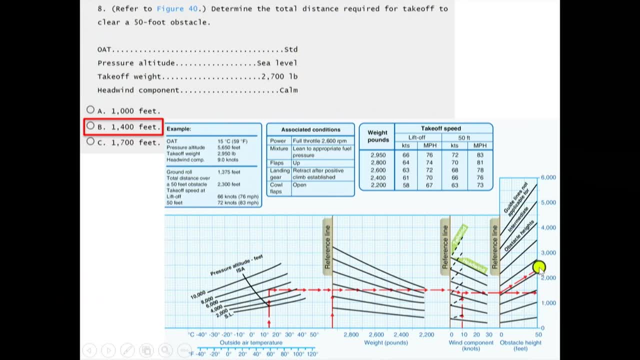 either this for the answer, or this for the answer, or this for your answer. Even in their worked example you can see their red line, for the answer is just parallel to that gray line. They're not picking one of the gray lines. 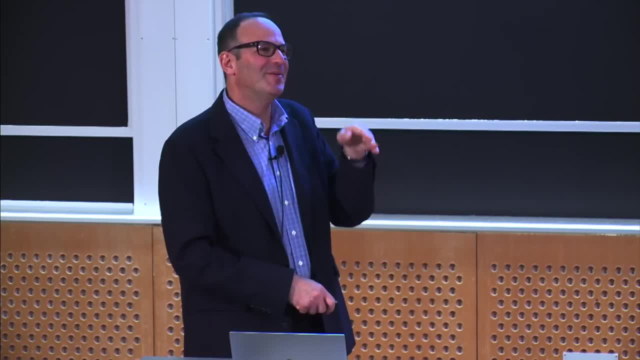 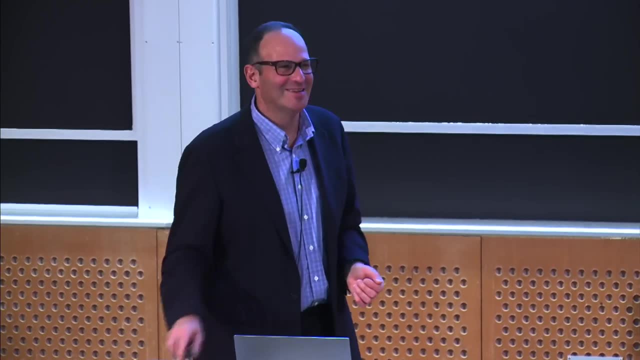 So they're guidelines for how you should move your pencil in each phase. I hope this motivates you to buy that Gironimo app. This certainly would motivate me to do it. If you want to look at it on a real book, I'll pass around. 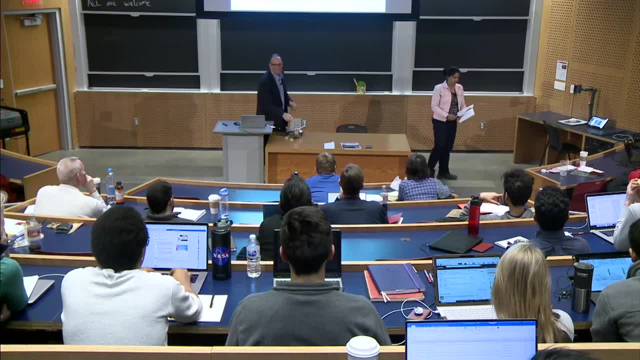 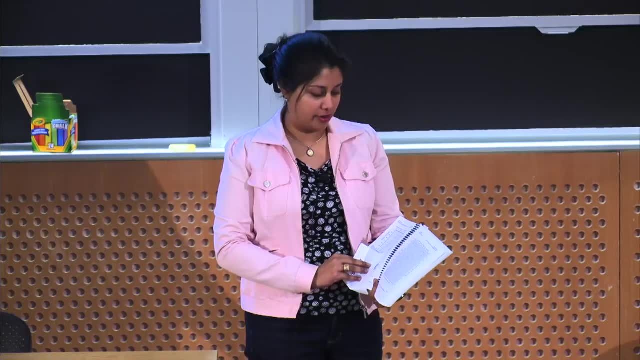 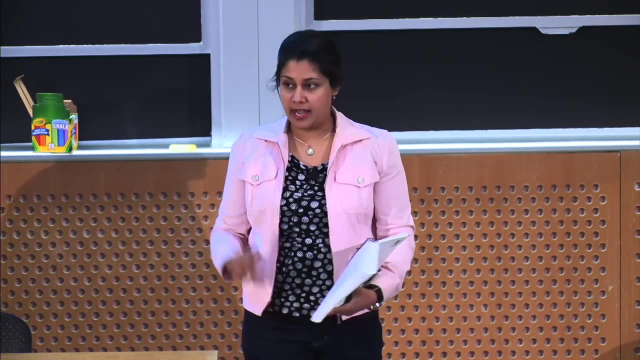 Again, This is my POH for Cessna 172.. So this might be the type of plane that you're using as your training aircraft, And I have a couple of pages that are marked with a piece of paper. So one talks about how you calculate the takeoff distance. 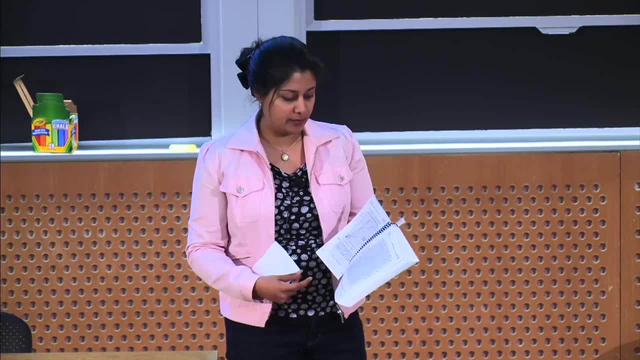 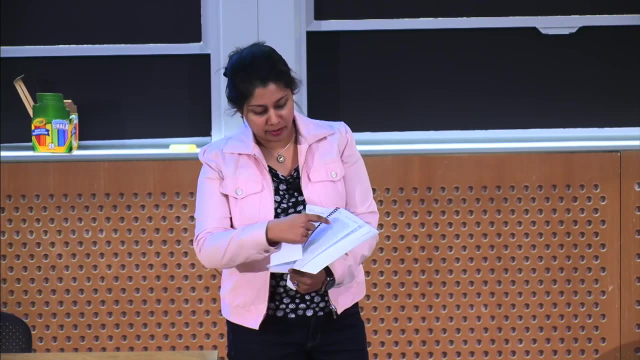 And one is weight and balance. We'll actually have a whole section dedicated to weight and balance, but just to give you a sense of how you can follow with your pencil And you'll actually see some pencil markings of my own And fairly close to the limits here- 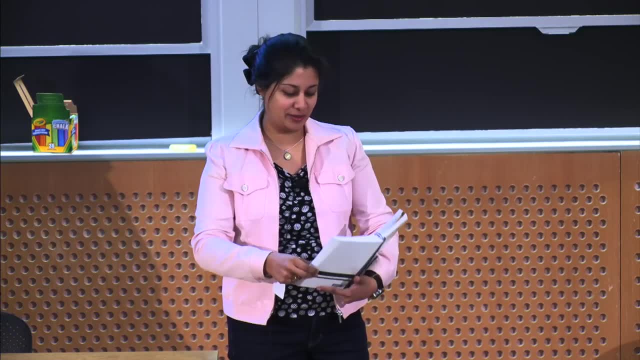 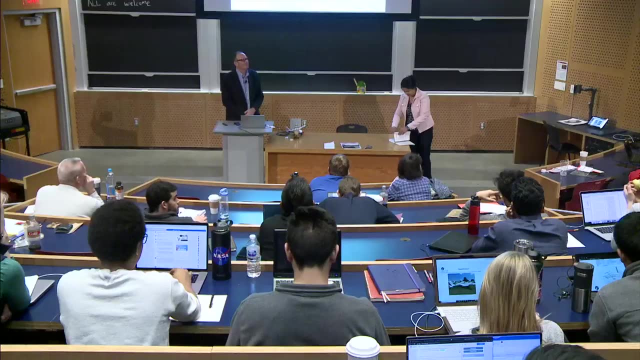 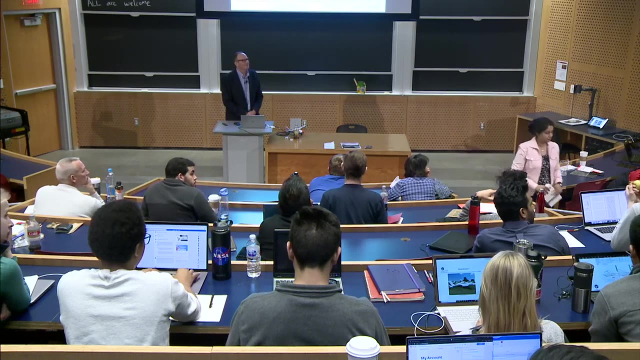 of our center of gravity moment envelope here, but still within the box. So just to give you an idea of how you can do that with a real paper and pencil. Yeah, I have a general question regarding pressure and density, So for this I've used density.